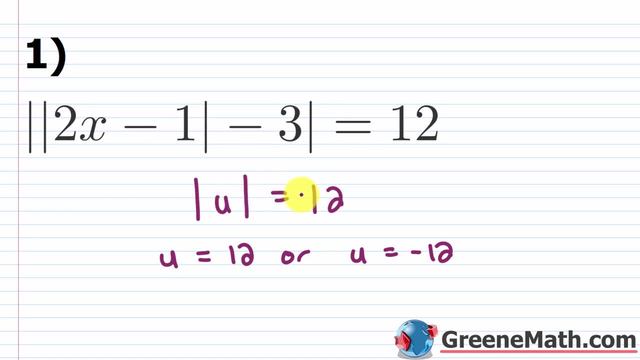 12.. So that will be true as well. So how can we use this rule on this guy here? Well, just consider this outer guy here as being set equal to 12, right? So what's inside is your u, So you would take what's inside here. let me. 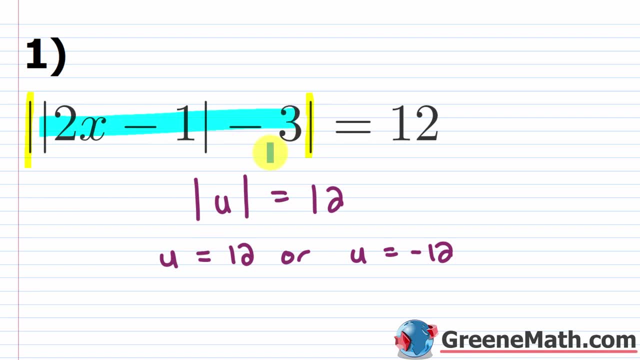 just highlight this in a different color. So this guy right here, we would set it equal to 12, then we would say: or it's equal to negative 12, right, Either way, you get a true statement. If you got 12 in there, well, the absolute value of 12 would be 12.. If you got negative 12 in there, 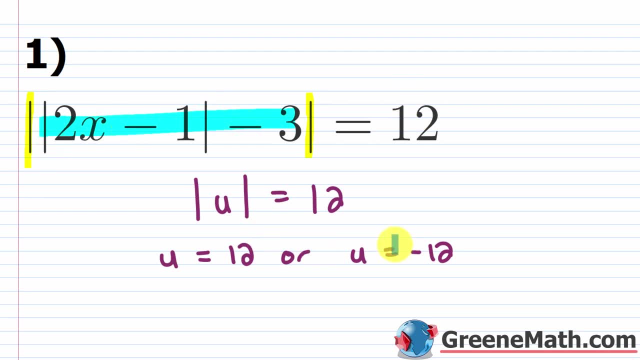 well, the absolute value of negative 12 would be 12 as well, just like we saw here. Okay, let's get rid of this And let's just set this up So we will have the absolute value of 2x minus. 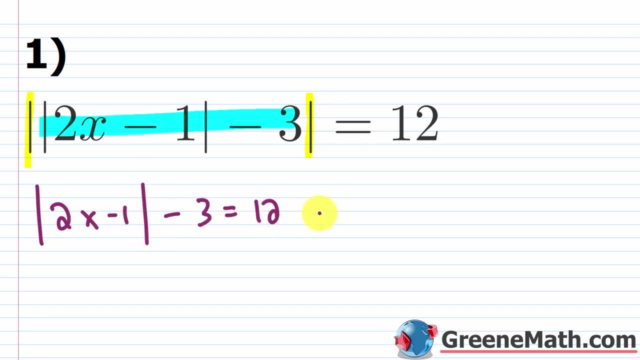 1 minus 3 is equal to 12, then I'm going to go. or the absolute value of 2x minus 1, then minus 3 is equal to negative 12.. Now, when you solve these types of problems, sometimes you'll get a setup. 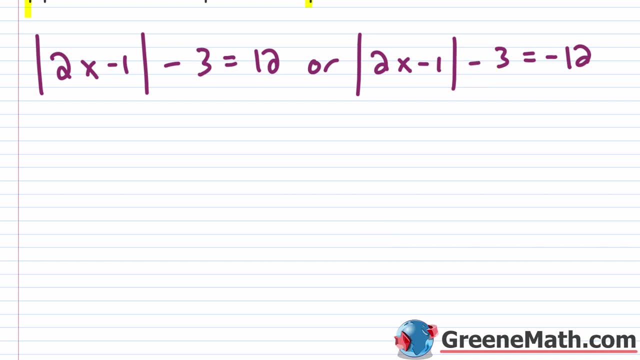 where there's no solution. Okay. so you're going to see that over here on the right. I'll get to that in a moment. So for these two guys, the first thing you'd want to do is isolate the absolute value of 2x minus 1.. So this guy right here and this guy right here, Okay. so on the left, 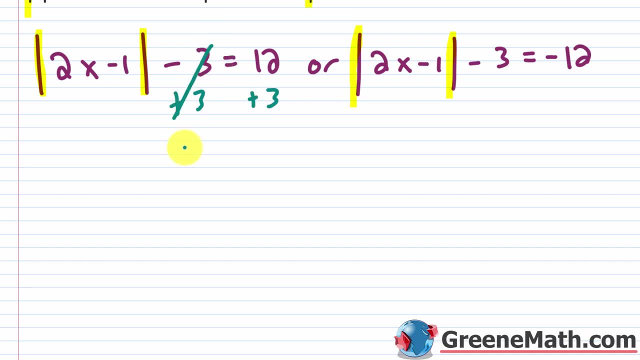 you would just want to add 3 to both sides of the equation. this would cancel. you'd have the absolute value of 2x minus 1. And this would be equal to 12 plus 3 is 15.. Let's say or over here. 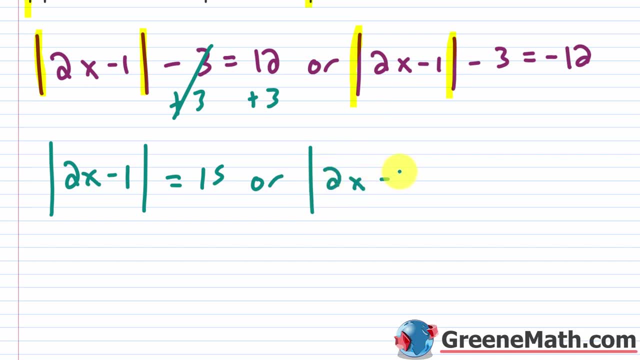 again, I'm going to isolate this guy. So we'd say the absolute value of 2x minus 1.. Again, I'm just going to add 3 to both sides of the equation. Let me make this 3 a little bit better. 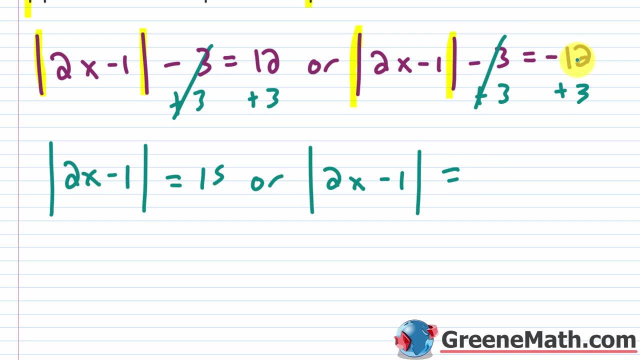 here. Let's cancel this and we'll say it's equal to negative. 12 plus 3 is negative 9.. Now, before we go any further, do you see a problem with this guy on the right? Well, yeah, you have isolated your absolute value operation And you're saying it's equal to some negative. 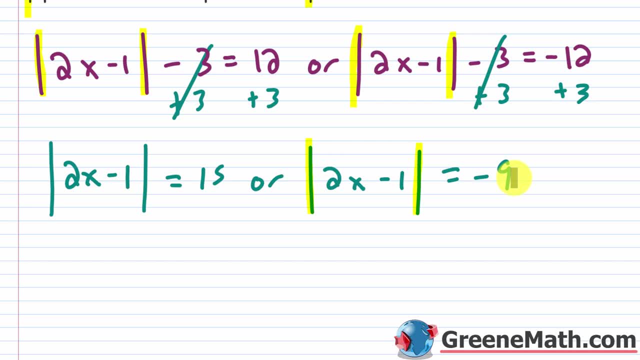 number. that is not possible. The absolute value operation will give you something that is zero or positive only, right, So your answer cannot be negative there. So what we would do here is just say that there's no solution. right, So this is no solution, And that is just for this guy on. 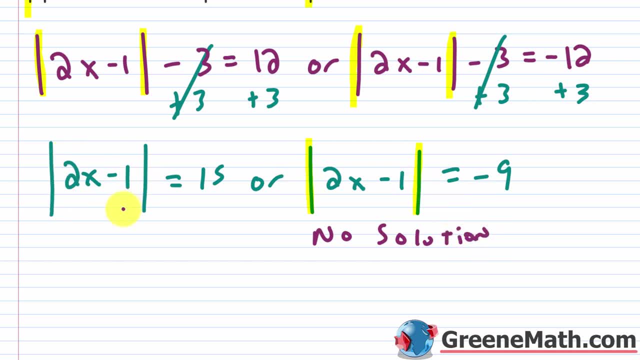 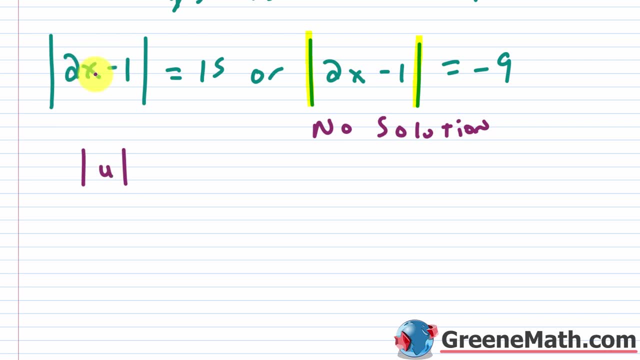 the right On the left, we can get a solution right. The absolute value operation can get a positive 15.. So for this one again, you turn to your rule. We would say: the absolute value of u, in this case u, is the 2x minus 1, that's equal to, let's say, 15.. Well then, u is equal to 15,. 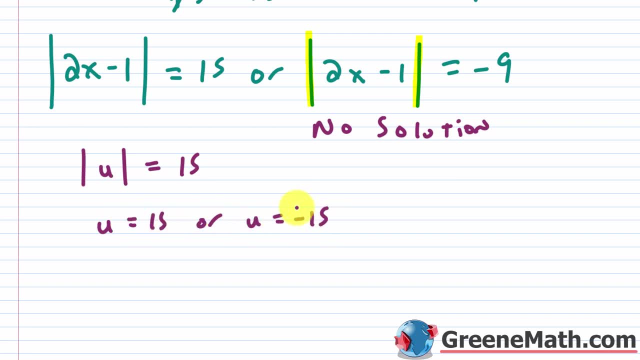 or u is equal to negative 15,. okay, So we just have to set this up. So we would say that 2x minus 1 is equal to 15, or 2x minus 1 is equal to negative 15.. So two simple equations to solve. 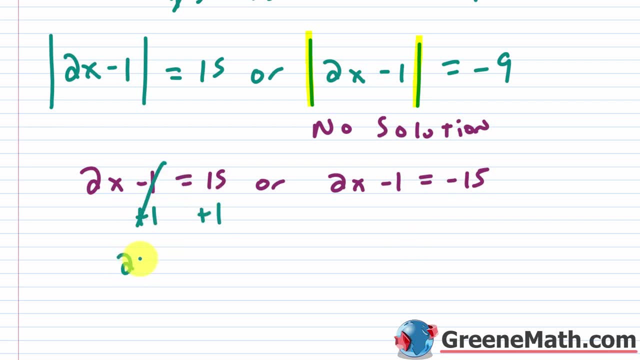 Let's add 1 to both sides. This cancels. We'll have: 2x is equal to 15 plus 1 is 16.. And then I'm just going to divide both sides of the equation by 2.. We'll cancel this. We'll say that x is equal to 16 divided by 2 is 8.. 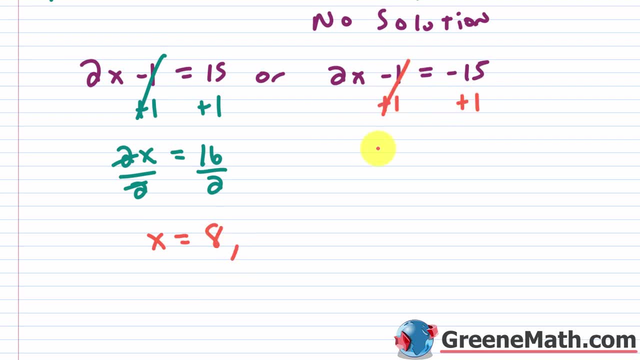 Then over here, let's add 1 to both sides of our equation. We'll cancel this. We'll say: 2x is equal to Negative. 15 plus 1 is going to give me negative 14.. Let's divide both sides of the. 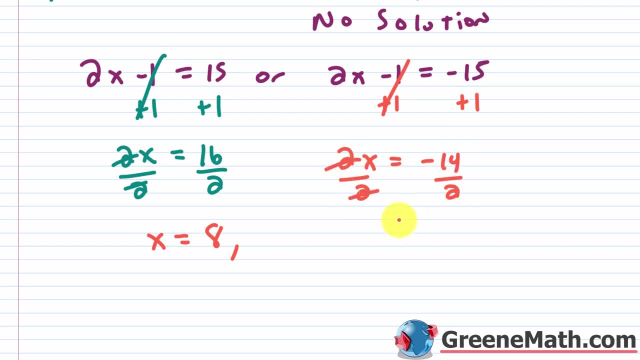 equation by 2. We'll cancel this And we'll say that x could also be negative 7.. So those are your two solutions: X could be 8, or x could be negative 7.. You can pause the video and go back. 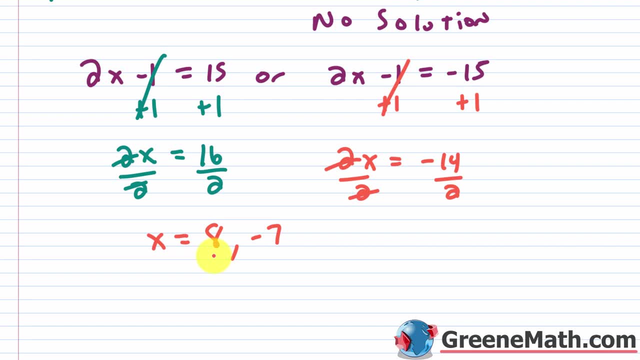 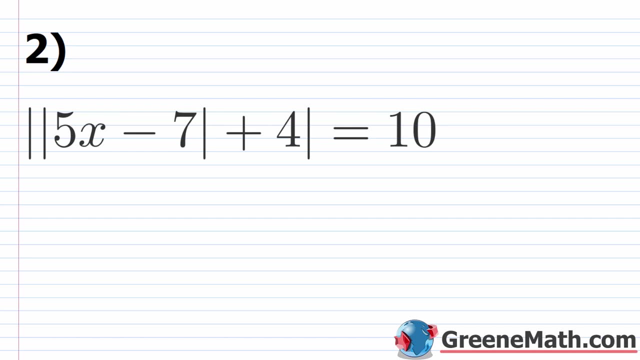 to the original equation and check each one, You'll see that the left and the right sides are equal. I'll just tell you in advance. I've already verified them and they both work All right. let's take a look at problem number 2 now. So here we have the absolute value of 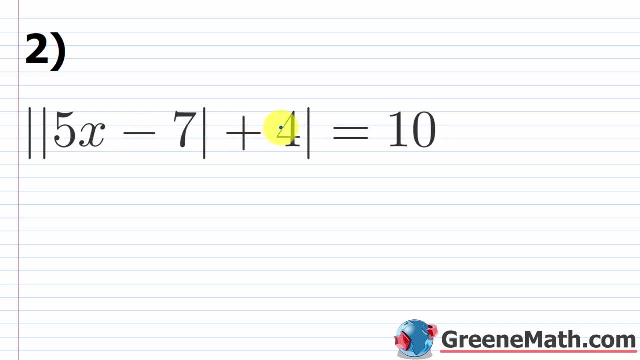 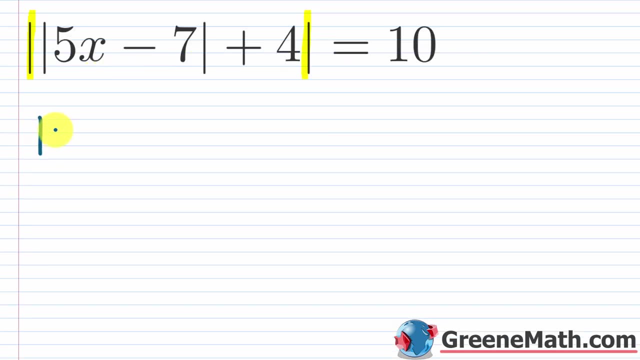 and then it's the absolute value of 5x minus 7, then plus 4, and this equals 10.. So, just like we saw before, we're going to consider this outside guy here and we will say that the absolute value. 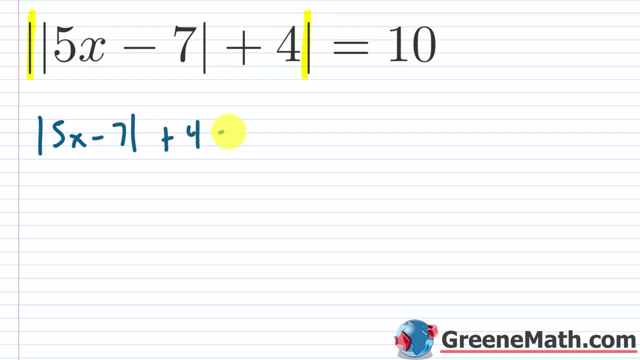 of 5x minus 7 is equal to 10.. We'll say that x could be higher than 7, and then we will say that x could be 7. then plus 4 is equal to 10. then we'll say: or the absolute value of 5x minus 7, and then plus 4. 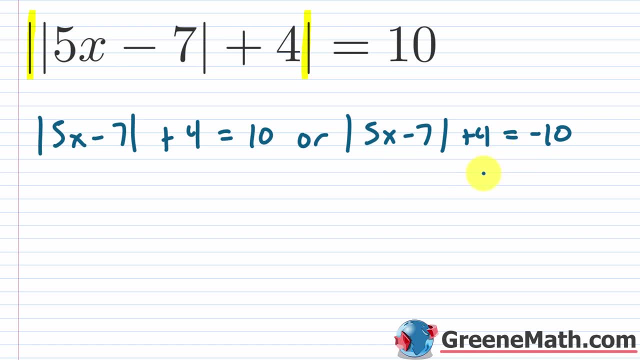 is equal to negative 10. okay, so those are the two scenarios. now again, you want to isolate your absolute value bars in each case. so on the left i would subtract 4 away from each side. this would cancel away. you have the absolute value of 5x minus 7 is equal to 10 minus 4 is going to give. 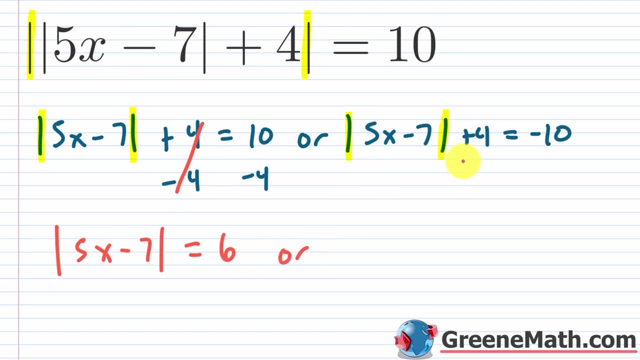 you 6. then over here, if we subtract 4 away from each side again, you're going to see you have a problem. so this is the absolute value of 5x minus 7 is equal to negative. 10 minus 4 is negative 14. 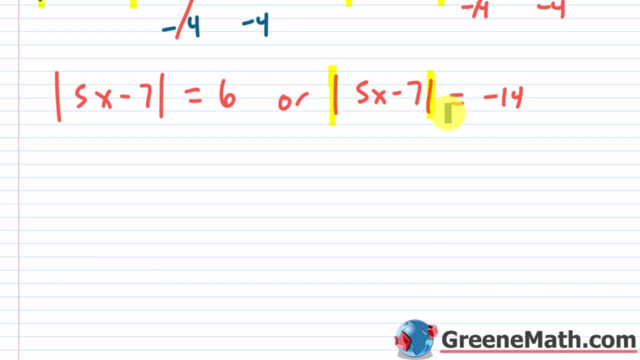 and again, when you think about it, this is isolated. so the absolute value of 5x minus 7. it's not possible for that to give you a result of negative 14 right. this over here on the right has to be 0 or some positive number. so once again, for this scenario we'll say there's no solution over here. 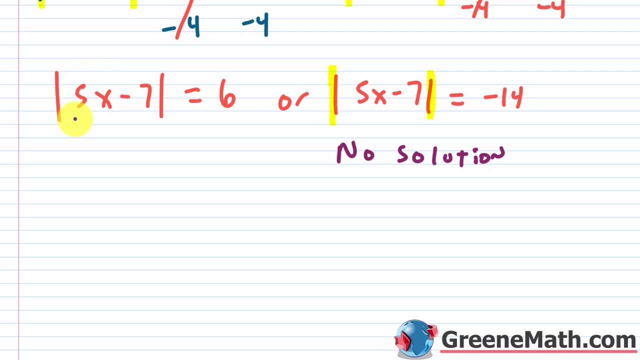 on the right. so no solution over here on the right. so we're going to subtract 4 away from each side. no solution now. on the left we can have the absolute value operation. give us positive 6, that's okay. so we would say that again, 5x minus 7 is equal to 6, or the 5x minus 7 would be equal. 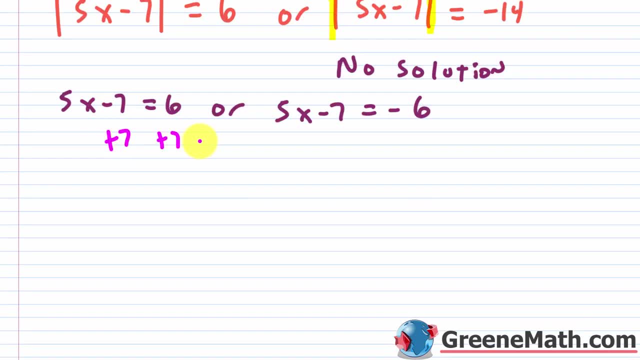 to negative 6. so here let's add 7 to both sides of the equation. this cancels. we have: 5x is equal to 6 plus 7 is 13. let's divide both sides of the equation by 5. let's cancel this and say x is 13. 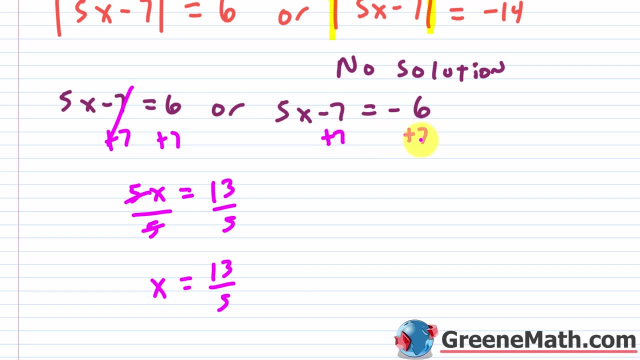 over 5 over here. let's add 7 to both sides of the equation and we're going to have a solution. this will cancel. you'll have: 5x is equal to negative. 6 plus 7 is going to be positive 1. let's divide both sides of the equation by 5. let's cancel this, so x could also be 1, 5th, all right. 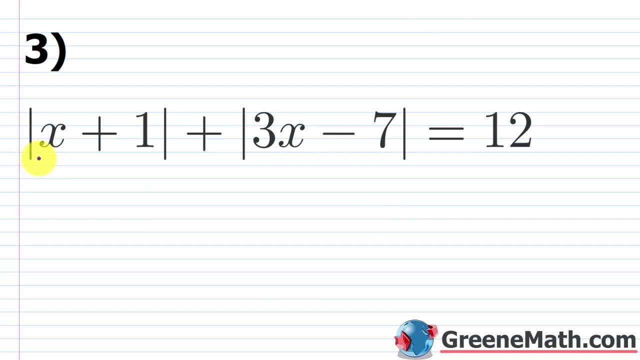 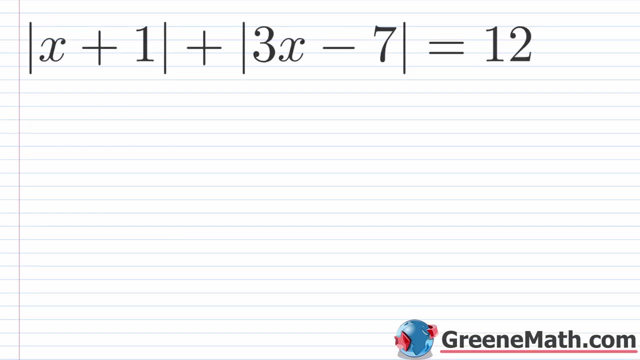 let's take a look at problem number 3 now. so we have the absolute value of x plus 1, then plus the absolute value of 3x minus 7, and this equals 12. now this type of problem is extremely tedious to solve and i got a lot of questions and comments and emails about it when i did it in the lesson. 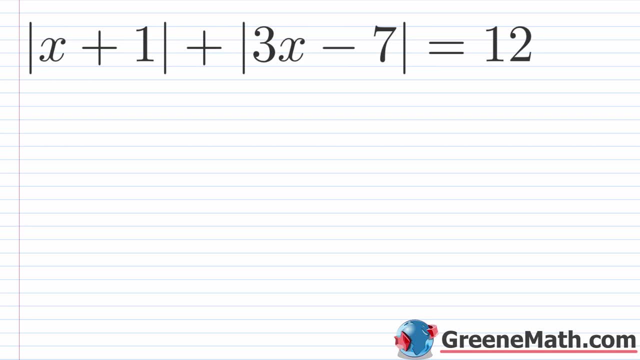 so i want to take my time and i'm going to take my time, and i'm going to take my time and i'm going to this first one and then we can go quicker on the next ones. so the first thing is, you have to realize that the absolute value equations that we've solved up to this point, they had a particular 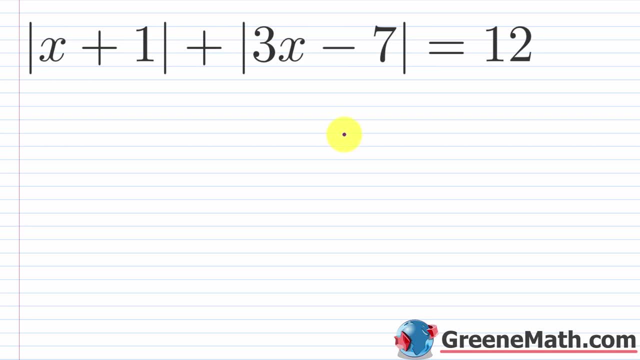 strategy right. so you wanted to isolate the absolute value. on one side, let's say you had the absolute value of some algebraic expression, u, so this is isolated. and let's say it's equal to some positive number, k. so this is a normal case. we say u is equal to k or u is equal to. 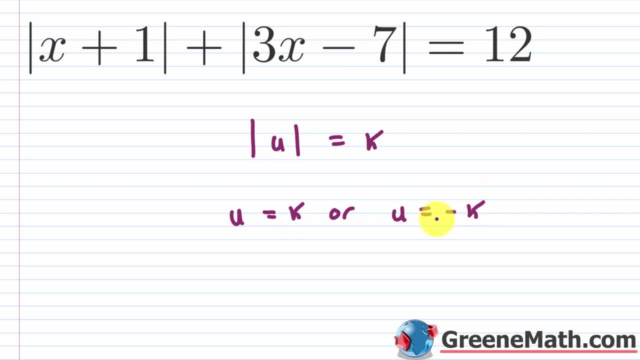 the negative of k. all right, so we cannot do that here. so we're going to take the absolute value operations here, because you have two absolute value operations involved, so this does not apply here. now, the other scenario is you have the absolute value of some algebraic expression, u. 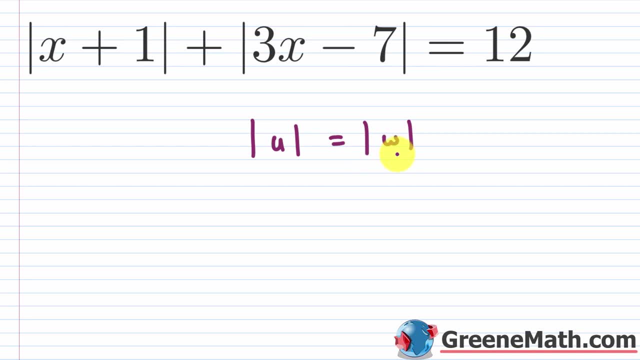 is equal to the absolute value of some algebraic expression, w. well, in this case you would say u is equal to w or u is equal to the negative of w. but again, we can't do that here because you have the two absolute value operations, but then you have this number over here. that's going to stop you. 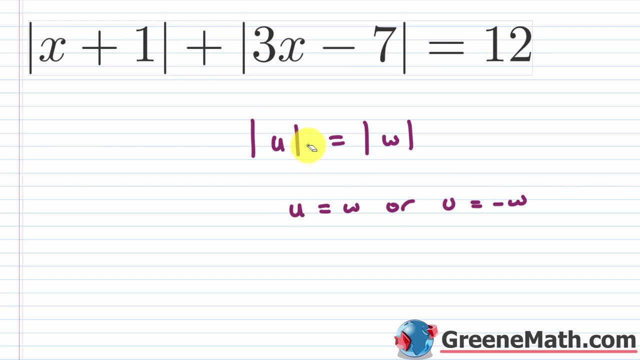 from setting them equal to each other, so this doesn't work either. so what can we do in this particular case? well, we're going to turn to our rule for absolute value, something that we talked about in algebra one. we're going to say that the absolute value of x is equal to x if x is non-negative, so if it's greater than or equal to zero, and then 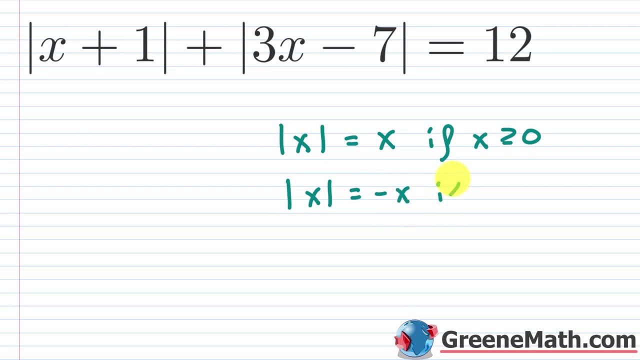 the absolute value of x is equal to the negative of x if x is less than zero. now, how can we use this simple definition to get an answer here? well, notice that we're developing a formula for dropping, a rule for when we can drop the absolute value bars and what we need to do. in other words, 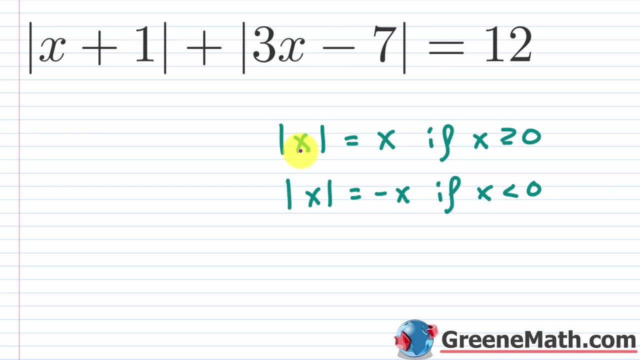 if what i plug in for x here is non-negative. so if it's zero or positive, i can just drop the absolute value bars and i get my answer. so in other words, if i had the absolute value of zero, i could drop the absolute value bars and i just get zero. if i had the absolute value of, let's say, two, i could. 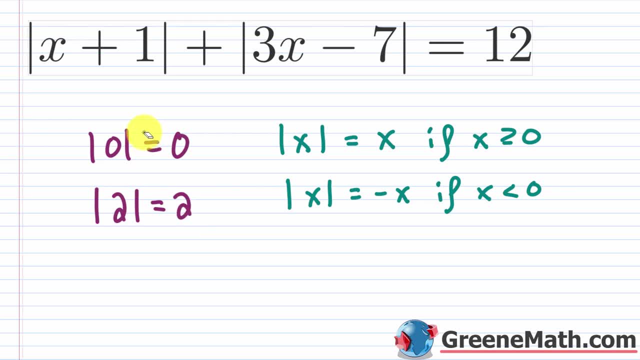 just drop the absolute value bars and i get two right. so it's nice and simple. but if i plugged in a negative here or something that's less than zero, well then i have to do additional work. i can't just so the absolute value of, let's say, negative nine is not just negative nine, i have to put a negative. 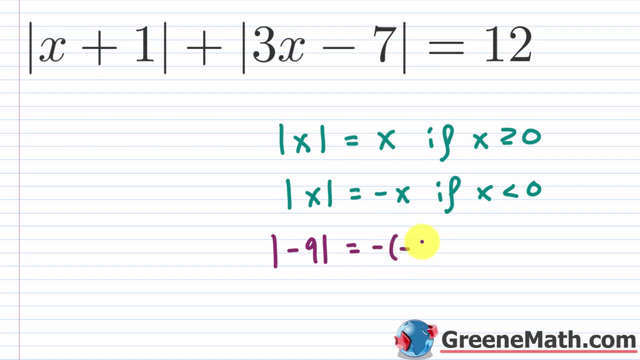 out in front, that's going to flip the sign. so the negative of negative nine, that's going to give me positive nine. okay, so this is what you need to understand. you're splitting things into different cases, okay, so what i'm going to do is apply this strategy to this guy and this guy. so in other, 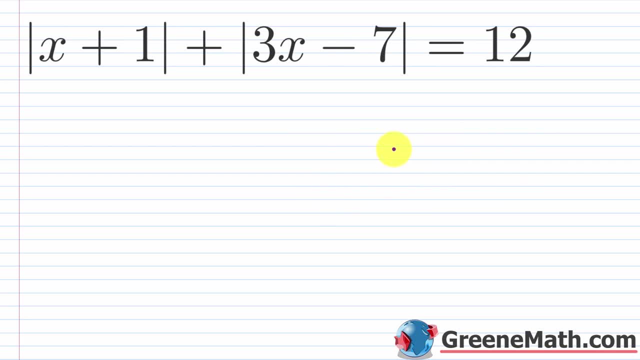 words. let me erase this. if i wanted to develop a rule for dropping the absolute value bars with this guy, we would say: the absolute value of x is equal to zero. so if i wanted to drop, the absolute value of x plus one is simply equal to x plus one. we'll say: if x plus one is non-negative, so if it's. 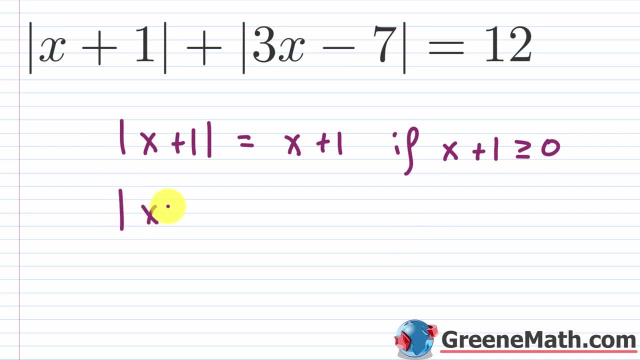 greater than or equal to zero, and then we'll say: the absolute value of x plus one is equal to the negative of x plus one if x plus one is less than zero. okay, so this is a simple inequality to solve. we would subtract one away from each side, so let me actually just erase this in each case. 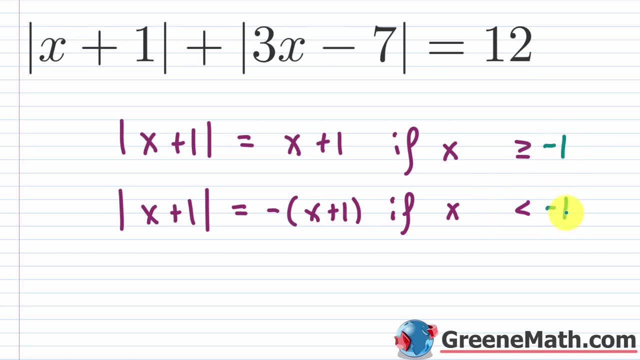 and just put this as a negative one or two. so let me actually just erase this in each case on the right side of each. okay, so if x is greater than or equal to negative one, then basically we could just drop the absolute value bars. right, we would just have x plus one. 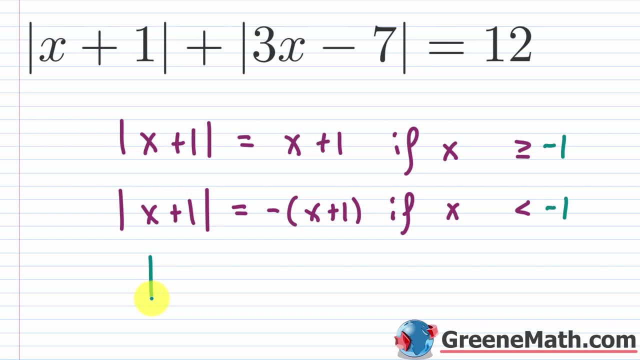 as our answer. you can try that by just saying: let's say we pick something like positive two, so the absolute value of two plus one is equal to. well, it's the same thing as if i just drop the absolute value bars. right, it's two plus one, which is three. okay, you can see our rule works. 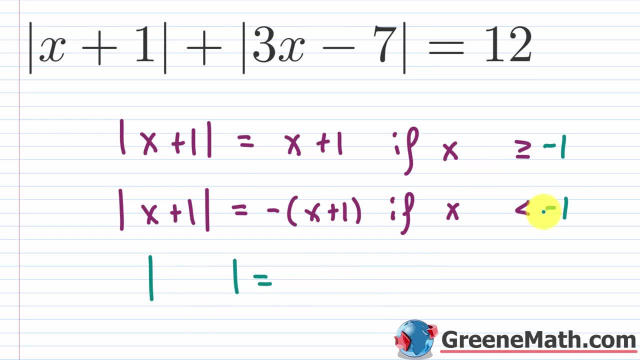 now the other one. let's say i had something that's less than negative one, right, and we have negative two, right, and we now have negative two plus one over negative one, and then that's two, and then we can kinda just pick what. let's say negative x plus one, so negative. 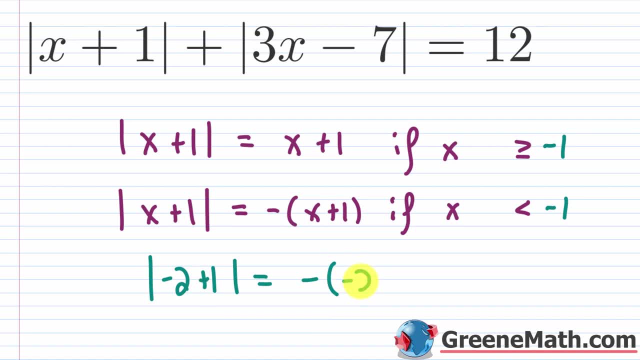 two plus one plus negative one. okay, so now we've got to flip the equation on the left-hand side. so if i had a green bar, you take the green bar and then i'm supposed to pick a blue one. so if i pick my absolute value bar, that doesn't change right. i get the absolute value, all right. so 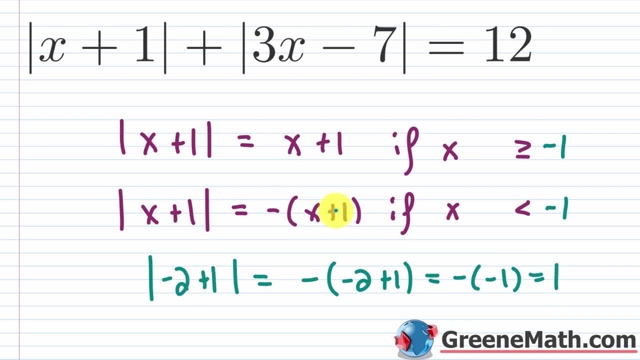 because when you do that, you're stepping over the written always working value. you can pick a negative two. or at the end of the equation, you're saying i can take my absolute value bar and you're saying i can pick negative two, going to be our rule, Okay. so this is the basic setup or strategy. Now you don't have to go. 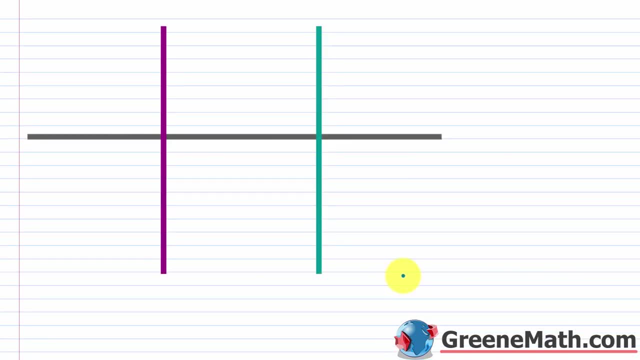 through and write this each time. which you would basically do is come down to a table or a number line And just think about where it's zero, and then anything that's less than that. you want the negative of that expression. And then anything where it's zero or positive, you want the expression. 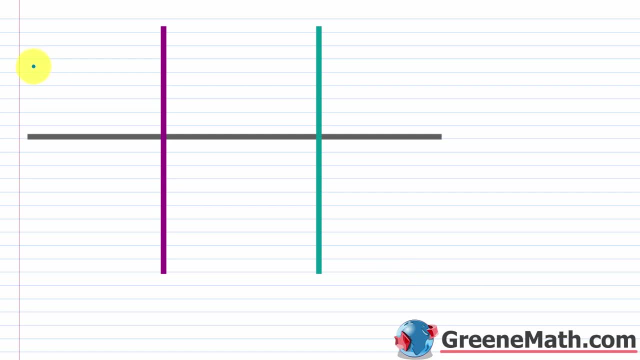 right, so you just drop the absolute value bars. So let me put an interval here from negative infinity going up to and excluding negative one, And in this particular case we want the negative of this quantity x plus one. So we want the negative of this quantity x plus one. I'm going 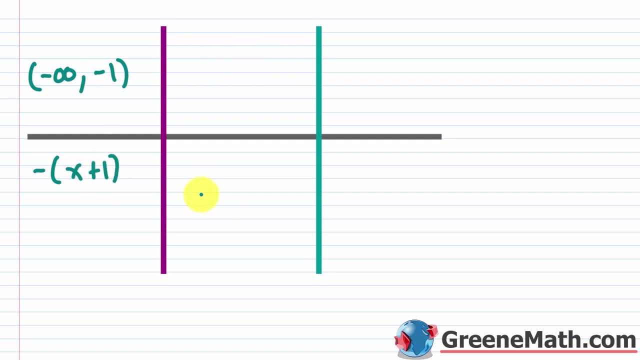 to put the interval here. in a moment we have to work on that other one. But I do know that if it's negative one or larger, then I don't need the negative of this guy. I can just drop the absolute value bars. So it would just be x plus one and then x plus one. Okay, so let's go back up And 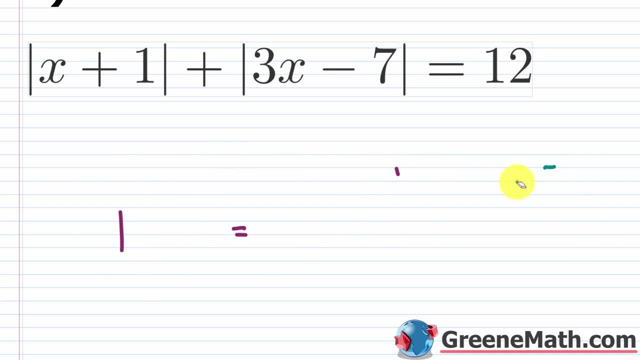 let's think about this other guy. So let's get rid of this And let's think about this other guy. So we have, the absolute value of three x minus seven is equal to- again- I'm just going to drop the absolute value bar- So three x minus seven. This is if. 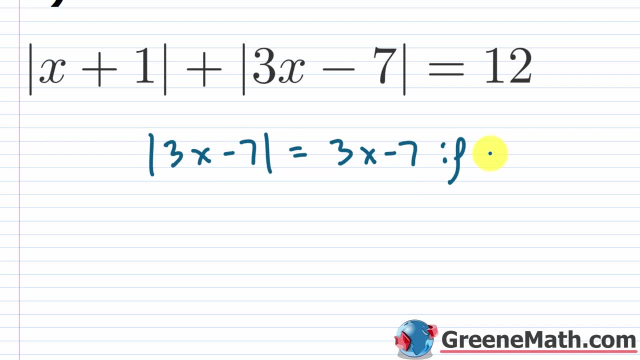 again, this expression is non negative. So we'll say that three x minus seven is greater than or equal to zero. And then we'll say the absolute value of three x minus seven is equal to the negative of three x minus seven. This is if we'll say three x minus. 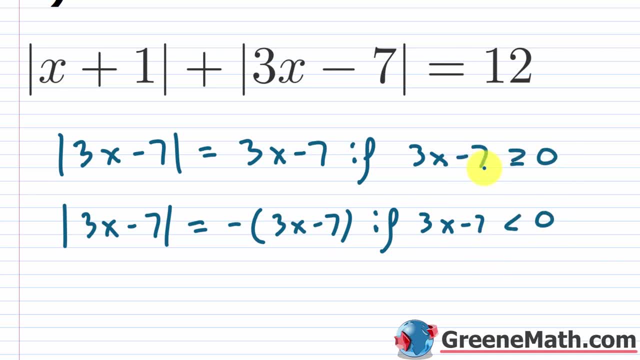 seven is less than zero. So for this one you would add seven to both sides- let me just do this on both of these at the same time- And then you would divide both sides by three. So basically you would say that if x is greater than or equal to seven thirds, that the absolute value of three 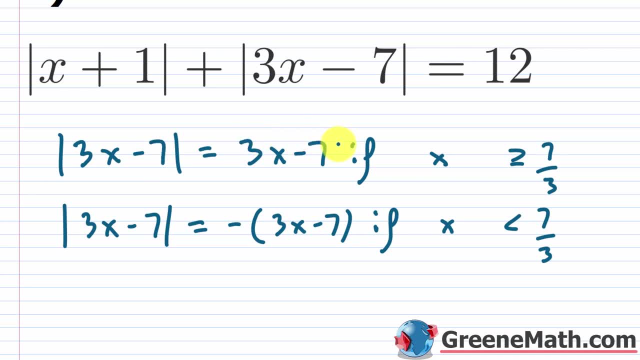 x minus seven can be found by just dropping the absolute value bars right, And then, if you're less than seven thirds, well then the absolute value of three x minus seven can be found as the negative of this quantity: three x minus seven. So we're going to go down here and we're going to go. 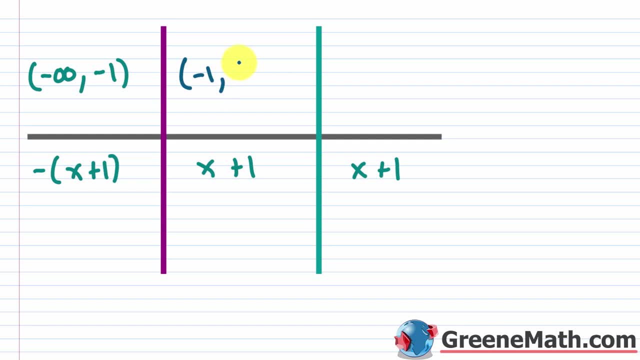 here and we're going to think about the interval between negative one and seven thirds and then the interval that's greater than seven thirds. Okay, and I'll talk about negative one and seven thirds in a moment. I know some of you are going to be confused as to why I didn't include it. 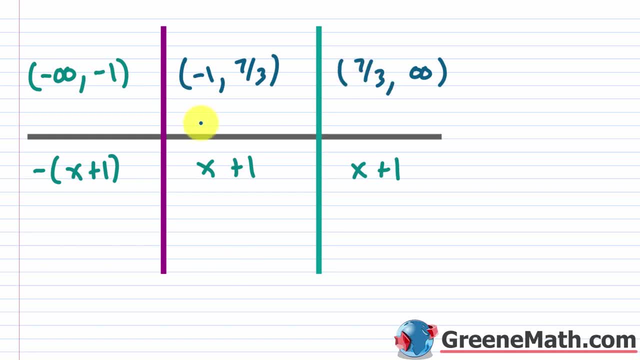 So, first off, anything that's less than seven. thirds, we know that we want the negative of this guy, right? So the negative of the quantity three x minus seven. so the negative of the quantity three x minus seven, and then the negative of the quantity three x minus seven. 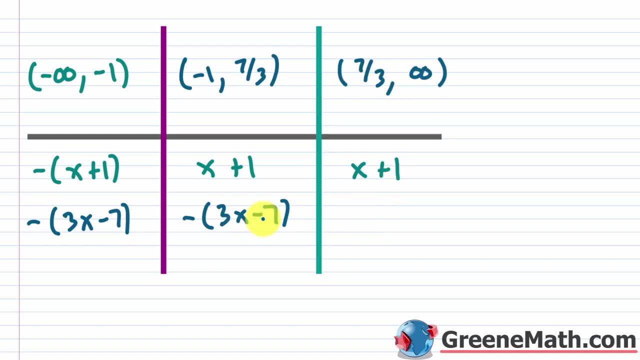 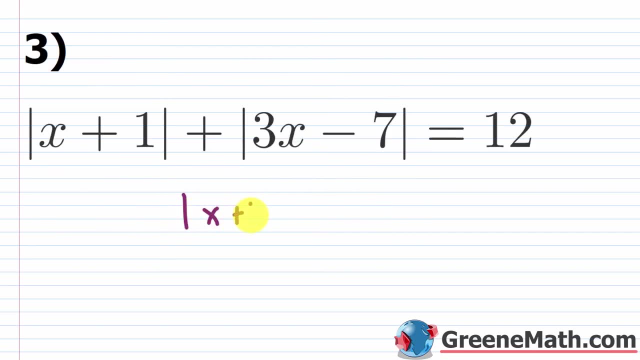 And then if I'm greater than seven thirds, then I just want the expression three x minus seven, so three x minus seven. Okay. so let me come back here and just copy this equation: So the absolute value of x plus one, then plus the absolute value of three x minus seven, this equals: 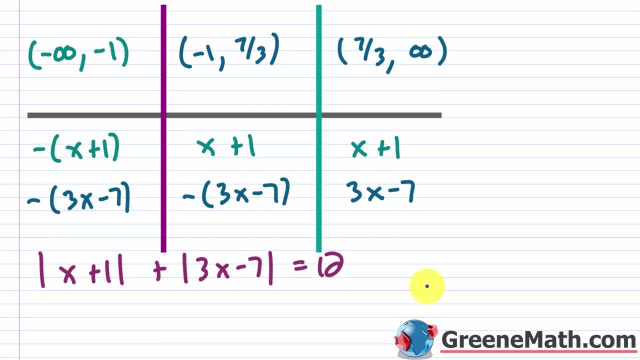 12.. Okay, so let me pause for a minute and talk about something that's probably a question that you're going to ask. I get this question a lot, So when some people set up these problems, you're going to get a lot of questions about how to solve them. And I'm going to go ahead and 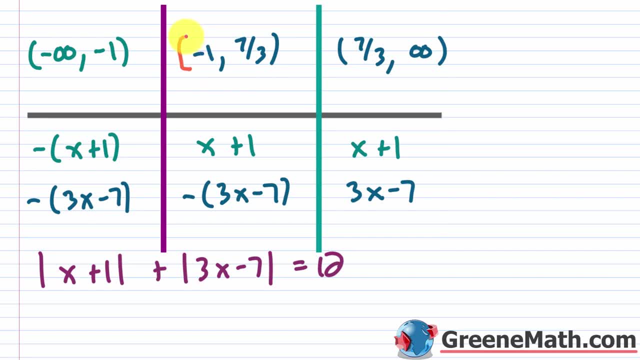 you'll see them include negative one here. And the reason you would include negative one here is because at negative one this guy right here is going to be zero. Plug in a negative one there. negative one plus one is zero, The absolute value of zero. again, you can just drop the absolute. 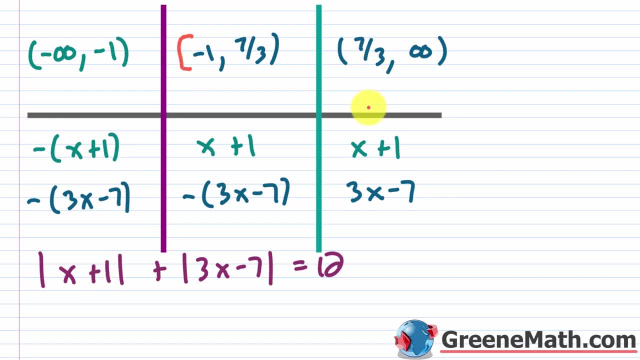 value bars. So you could include that there. And then the same thing over here. you could include this right here if you wanted to. okay, Because if you plug in a seven thirds there, this guy right here is zero And the absolute value of zero again. you could just drop the. 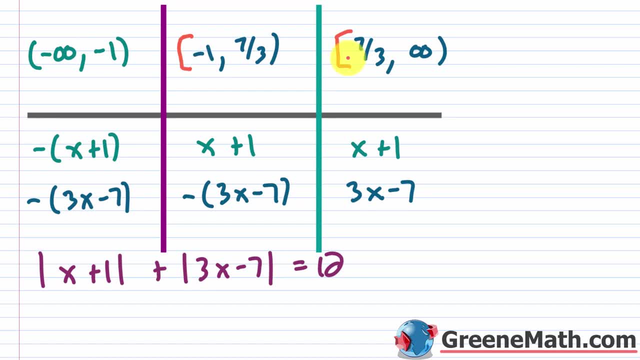 absolute value bars. So if you're doing this problem on your own and you want to include it, you can. okay, It's up to you. This is just scratch work, So I always like to consider those guys separately, okay. 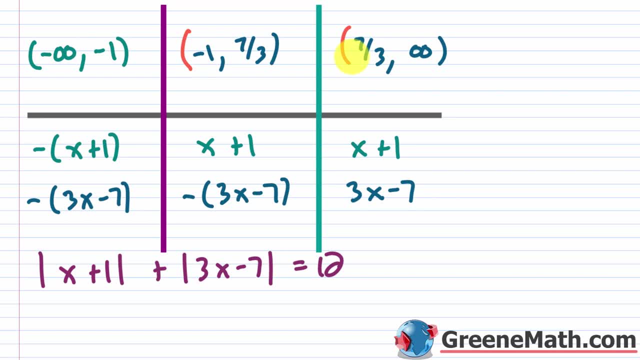 So this is just my strategy, the way that I do it. If you want to do it the other way, it's still valid. It's not going to change your answer. We're going to see, in a few problems, one where we actually get one of these guys as our solution. 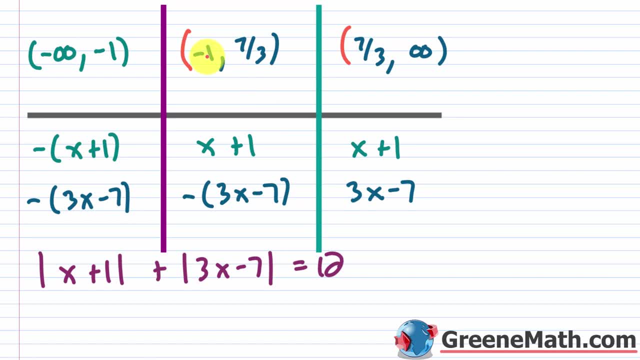 That is pretty much a special case, and I'll show you what to do when that happens. So, from this point, all we would need to do is basically use our rule to set up a different equation for each interval. We would solve that equation. 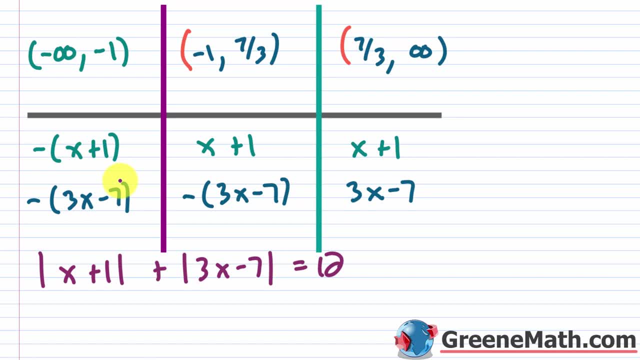 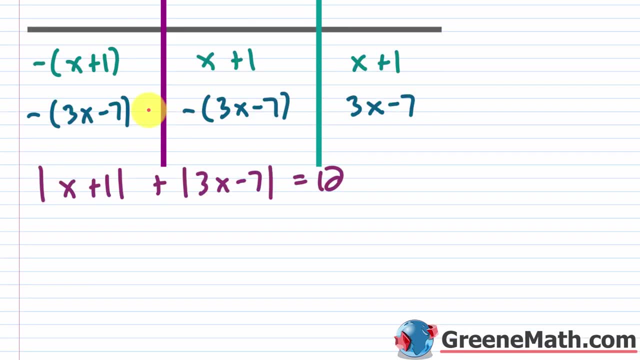 and then we would see: does the solution lie in the interval? If it does, we'll accept it, If it doesn't, we will reject it. okay, So let's start with anything that's less than negative one. So building my equation here, 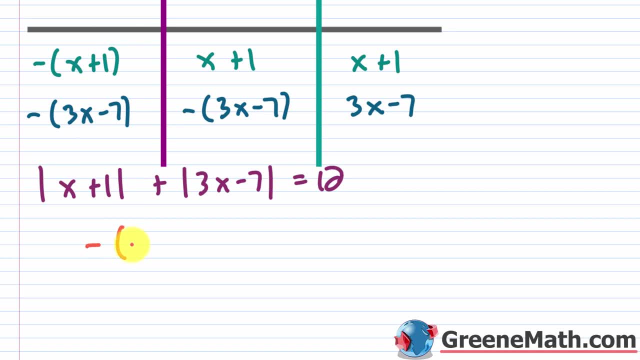 again, if I drop the absolute value bars, I use this rule. So the negative of this quantity, X plus one, and then plus the negative of, you might as well just write minus the quantity three X minus seven Again, that's so I can drop. 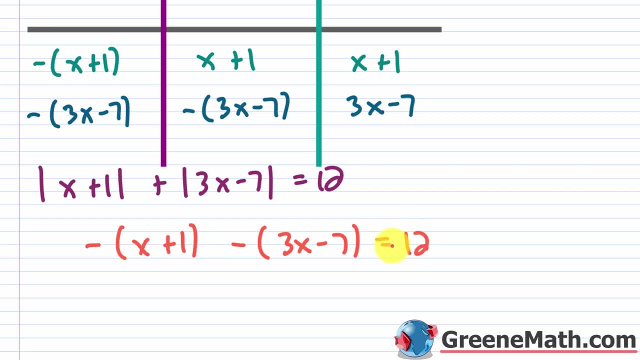 these bars, and this equals 12.. So I'm going to solve this, and if I get something that's less than negative one, I can accept it. If it's not less than negative one, I will reject it. So let's go down, we'll come back up. 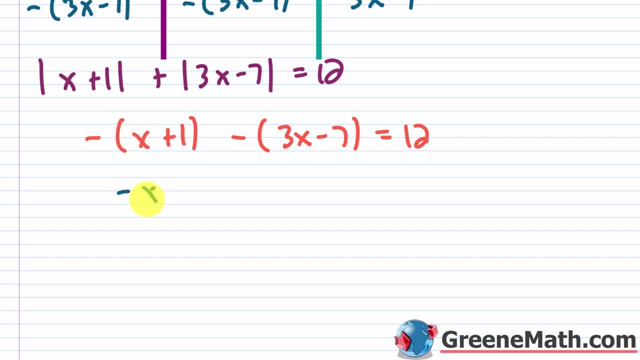 So here we have the negative of X plus one, so it's just basically negative X and then minus one, just multiplying each guy there by negative one, And then here I'll do the same thing. So negative one times three X is minus three X. 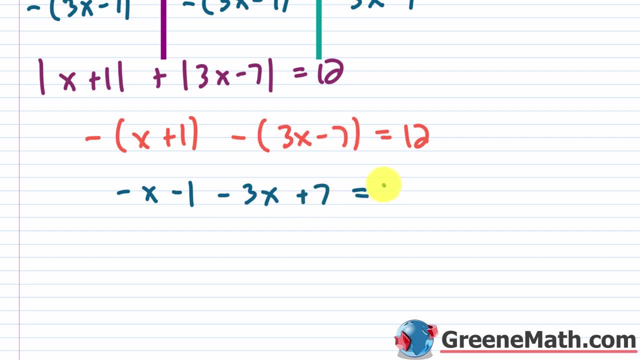 and then negative one times negative. seven is gonna be plus seven. This equals 12, right? So if you struggle with that, you can always just put a negative one there and put a plus a negative one there and you're just distributing this to each. 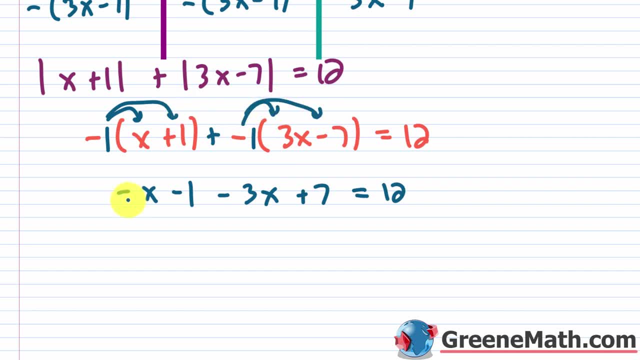 in case you are confused about that. okay, So from here, negative X minus three X is negative four X, and then negative one plus seven is going to be positive six, and this equals 12.. We will subtract six away from each side of the equation. 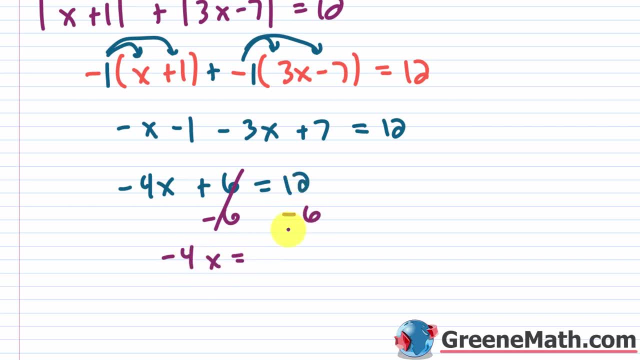 Let's cancel this. We get negative four. X is equal to 12 minus six is going to be six. Divide both sides of the equation by negative four. We'll say that X is equal to. let me show this is canceling. 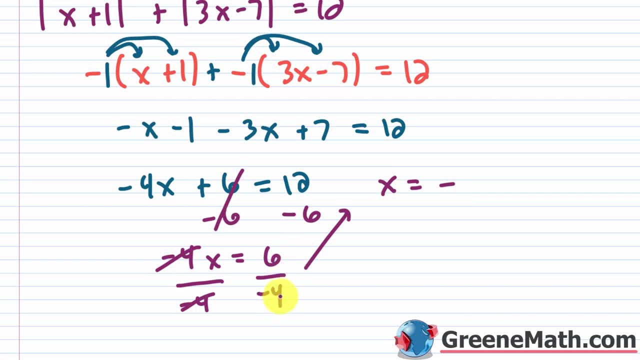 You would have a negative, because a positive over a negative is a negative, and six and four are each divisible by two. Six divided by two is three and four divided by two is two. So you get X equals negative, three halves. Coming back here, let me write X. 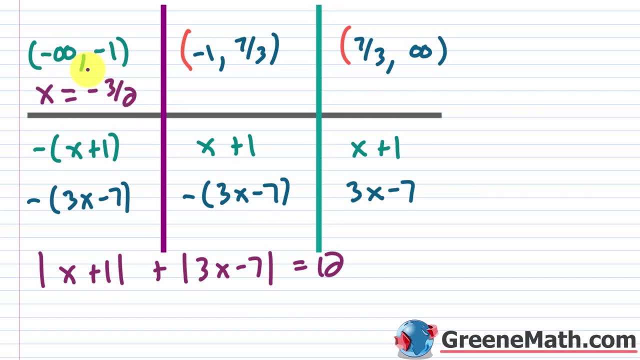 is equal to negative three halves. Is this in my interval? Yes, because I'm looking for something that's less than negative one. This is basically negative 1.5, so it's to the left of negative one on the number line. 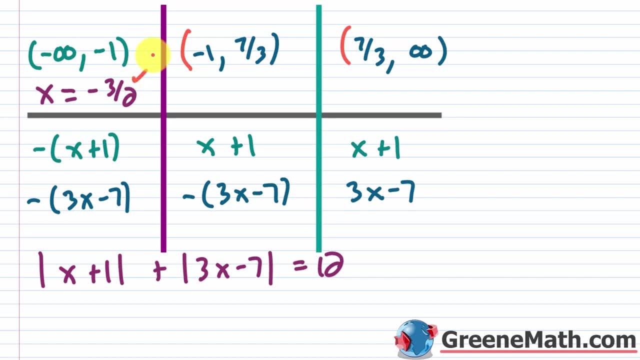 right, so this is in this interval, So we would accept this solution. So I'll just put a check mark there Now. in the next interval, this is between negative one and seven thirds. So we're going to use our rule. 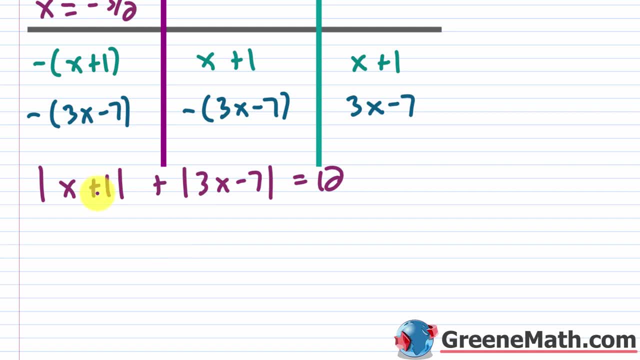 So again, for this one you could just drop the absolute value bars, because this one's going to be positive in that interval. Or again, if you wanted to include negative one itself, then it would be non-negative. So we'll just say X plus one. 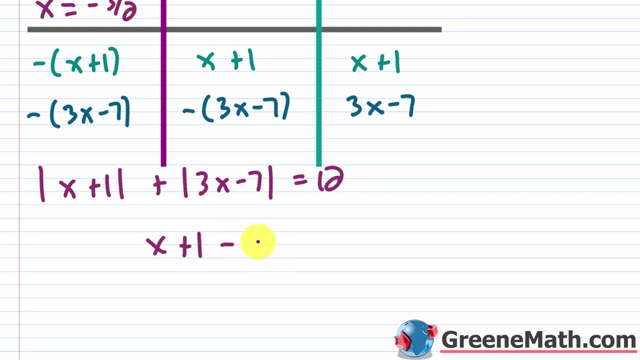 Then to drop this guy again. this guy is negative in that interval. So let's put minus this quantity three X minus seven, And again you can go plus negative one if that's a little bit easier for you, And this equals 12.. 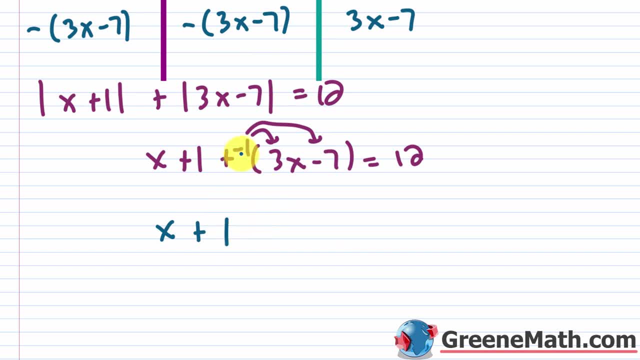 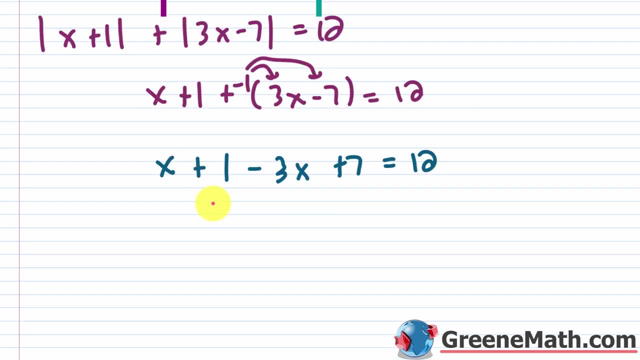 Okay, so we have X plus we have one. the negative one times three X is minus three X. The negative one times negative seven is plus seven And this equals 12.. Okay, so we will have X minus three X, which is negative two X. 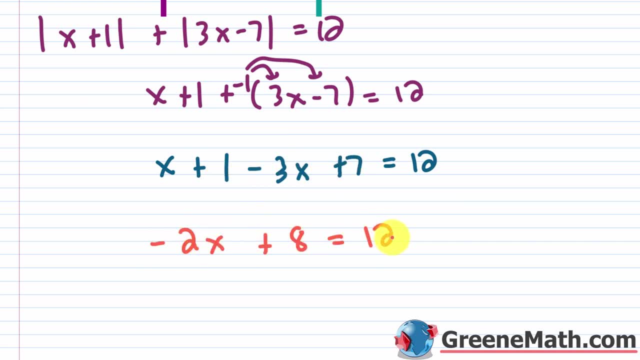 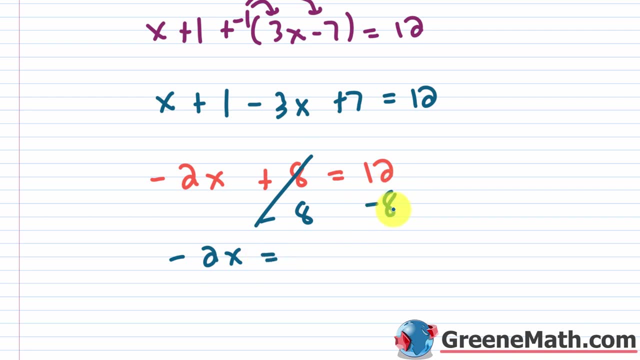 And then one plus seven is going to be eight. This equals 12.. So here we would subtract eight away from each side of the equation. This cancels. You have negative two. X is equal to 12 minus eight is going to be four. 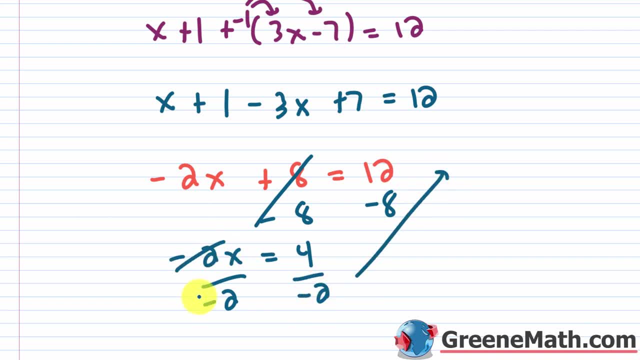 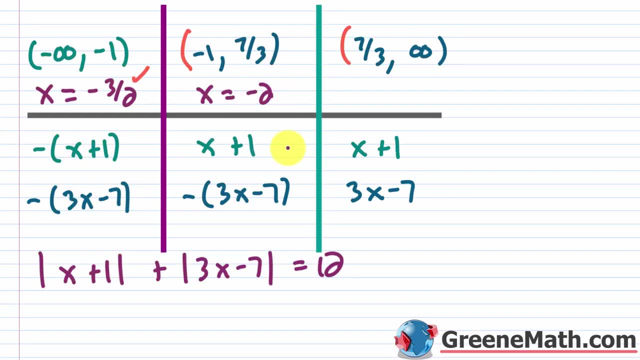 Let's divide both sides of the equation by negative two, And we're going to cancel this and say: X is equal to four divided by negative two. Negative two is negative two. So, coming back, I'm just going to write: X is equal to negative two. 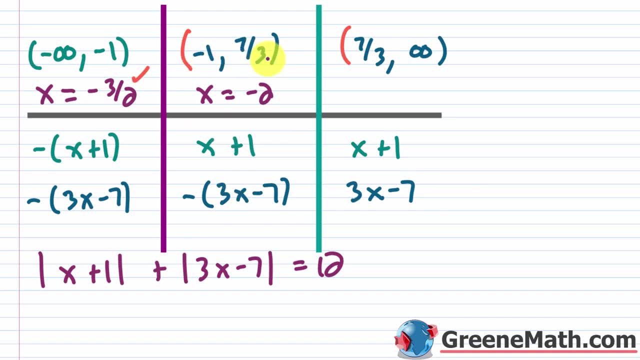 Now, is this in this interval? No right, Because this is between negative one and seven thirds, Or again, if you wanted to include negative one, you could say that's part of it, but it does not fit in this interval here. 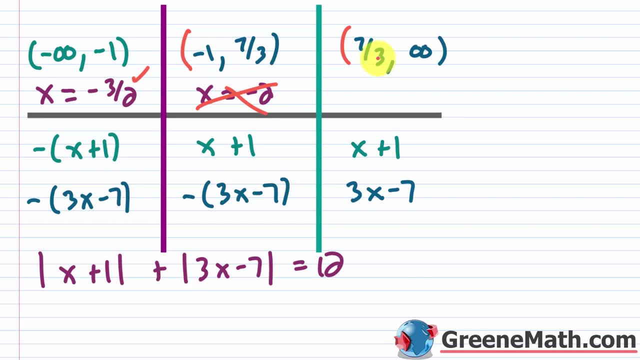 So you're going to reject this? Okay, you don't want that answer? So then now I'm working with this interval between seven thirds and infinity, Or again, if you want to include seven thirds, you could if you wanted to. it's not going to change anything. 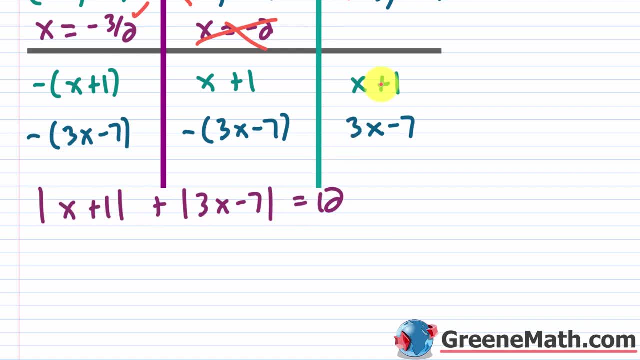 So we're going to say that we can just drop the absolute value bars because everything is going to be negative. So we can just drop the absolute value bars because everything is going to be negative. So we're going to say that we can just drop the absolute value bars because everything is going to be either non-negative if you included seven thirds, or positive if you didn't. 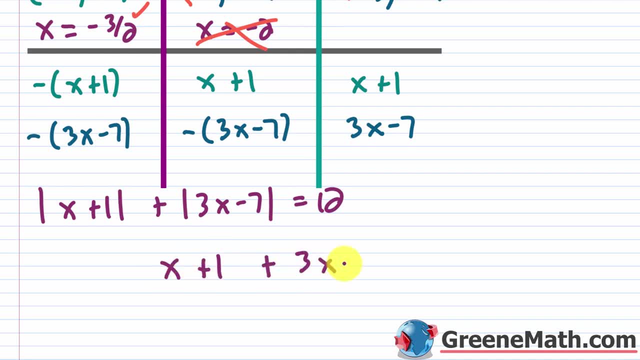 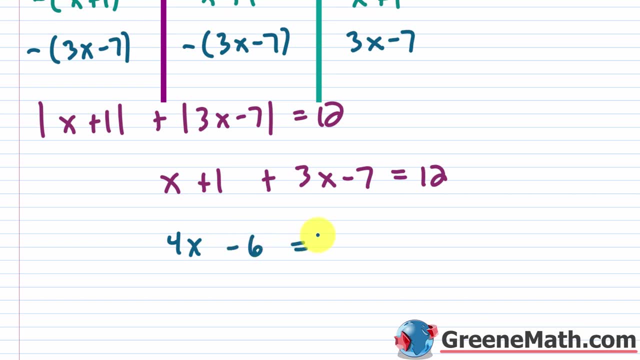 So we'll say X plus one, then plus three, X minus seven is equal to 12.. So we'll say X plus three, X is four, X, And then one minus seven is going to be negative six And this equals 12.. Let's add six to both sides of the equation. 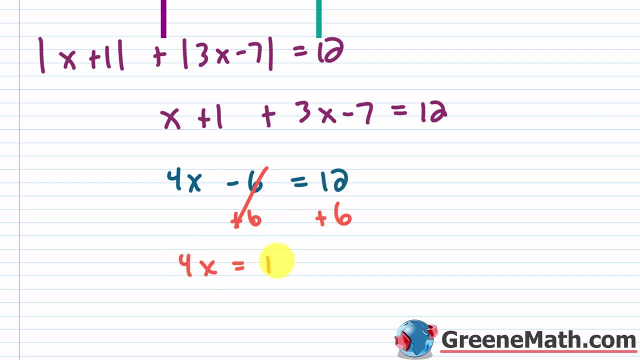 This cancels, We get four. X is equal to 12 plus six is 18.. Let's divide both sides of the equation by four. So we're going to cancel this with this And we'll say: X is equal to For 18 and four. 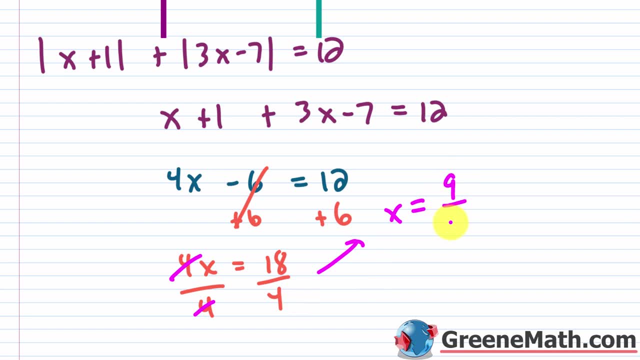 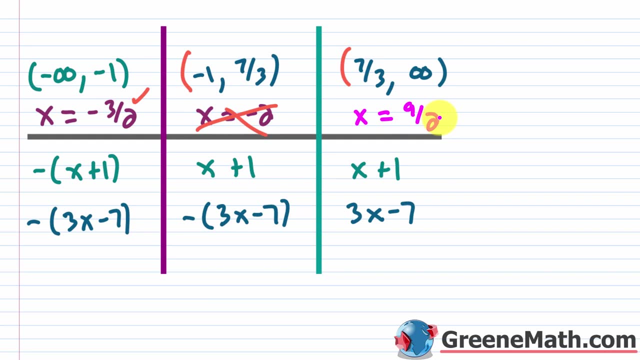 they're each divisible by two. 18 divided by two is nine. four divided by two is two. So this is X equals nine halves. So coming back up here, I'll say X is equal to nine halves. Now, nine halves is 4.5.. 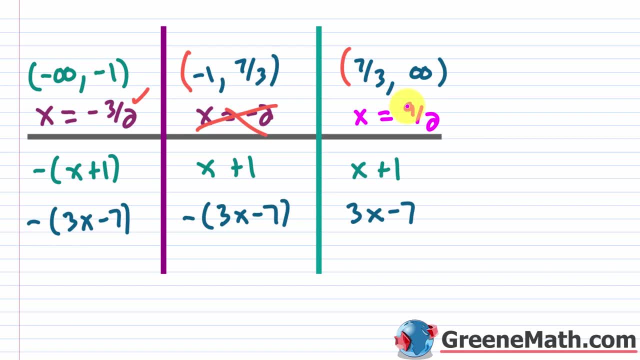 And if you think about seven thirds, I would say that's two and a third. So 4.5 is obviously greater than two and a third, So it fits in this interval. So you can accept this solution. So, going back, let me just write this out here: 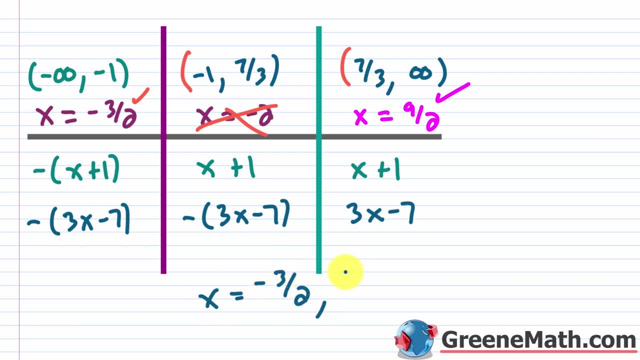 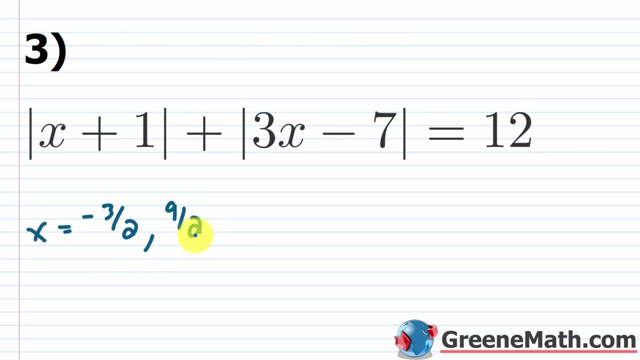 You have, X is equal to negative three halves, and then also nine halves. So, coming back here, I'll just paste the solution there. So this would be our full solution. Again, you can always pause the video and check each one of these. 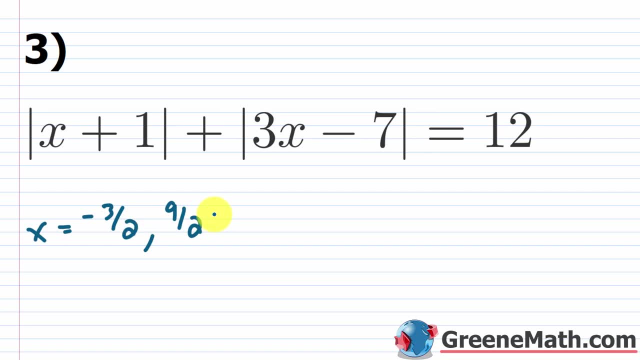 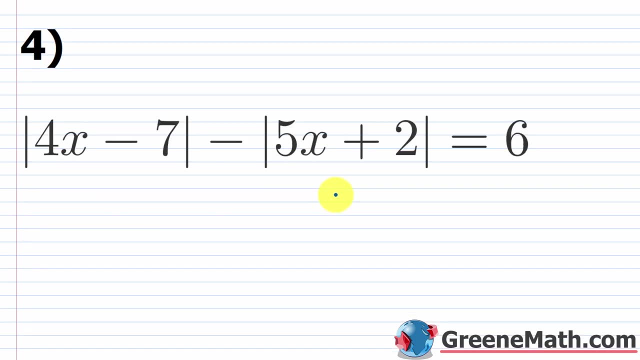 make sure it works in this equation. I've already verified each one of these solutions. You can even take that solution that we rejected, that negative two. you can plug it in and see it's not going to work. All right, let's take a look at problem number four. 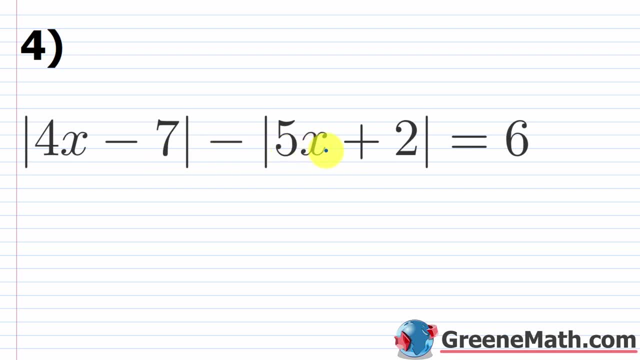 So we have the absolute value of four X minus seven, then minus the absolute value of five X plus two, and this equals six. So we spent a lot of time on the last example like this, So we're going to go ahead and do that. 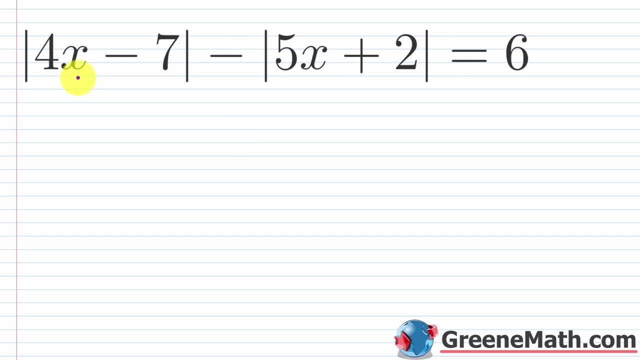 So we're going to go ahead and do that. So we're going to go ahead and do that. So for this one, I'm going to go a lot faster Again. the first thing I'm going to do is figure out where this is zero and where. 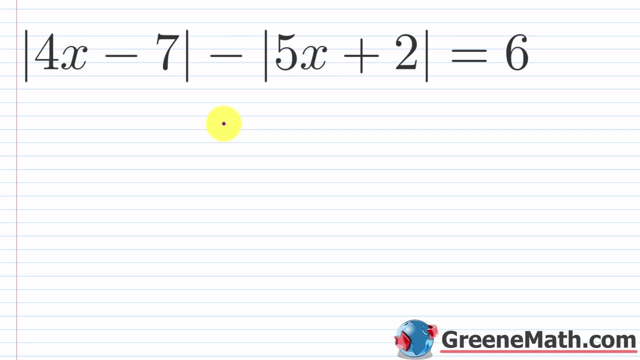 this is zero. And then I'm going to set up intervals on my number line. So we're going to say four X minus seven is equal to zero. We'll add seven to both sides, We'll cancel this away and say four X is equal to seven. 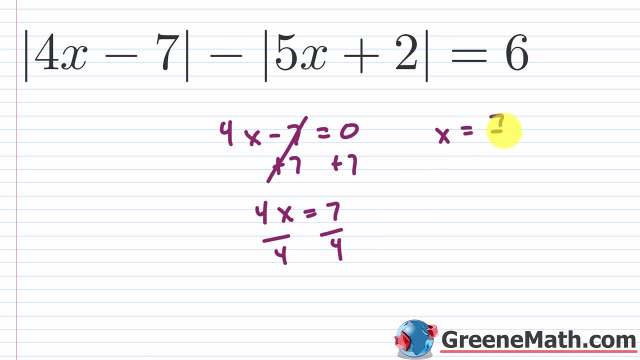 divide both sides by four and we'll get: X is equal to seven fourths. Okay, So the other one. we're going to set five X plus two equal to zero. Let's subtract two away from each side, We'll say five X is equal to negative two. 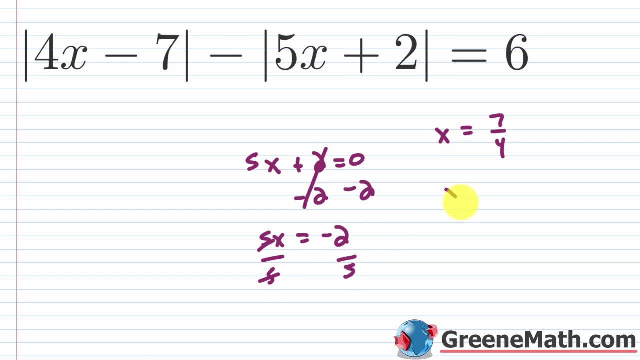 divide both sides by five, We'll cancel this. We'll say X is equal to negative two fifths. Okay, So we have those two guys and basically we're going to use them to set up our intervals on our little table here. Let's paste this in here. 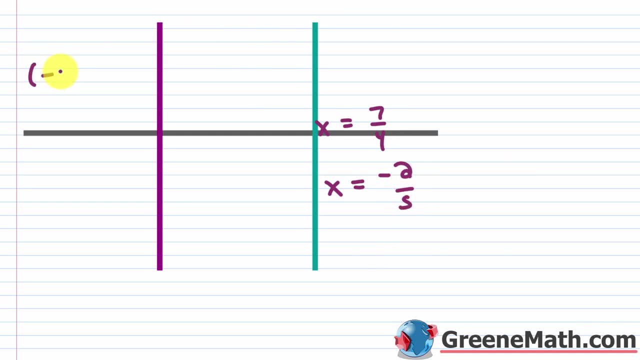 So negative two fifths is my leftmost value. So I'll say from negative infinity up to an excluding negative two fifths. Again, if you want to include negative two fifths you can. you could say this is negative two fifths here. 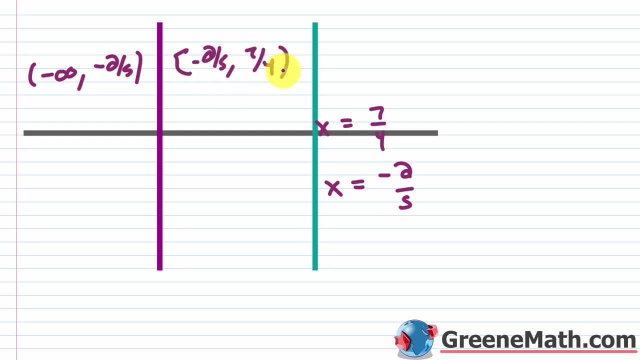 And then you're going to exclude negative two fifths, Exclude seven fourths. So that interval. there again, my preference is to do it this way. If you want to do it the other way, it's up to you. It will not change your answer in any way. 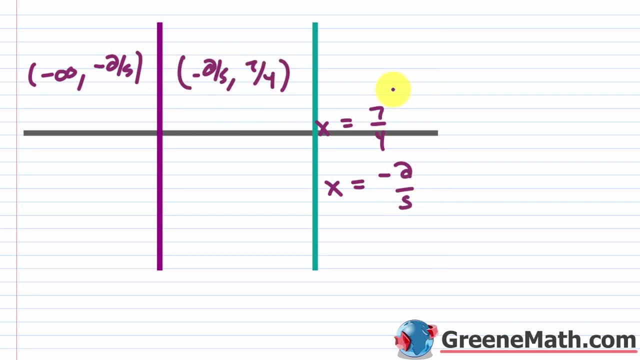 shape or form, Okay. Then the other one is going to be from seven fourths out to positive infinity. Again, if you want to include it, you can won't change your answer. I am going to exclude it, Okay. So let's look at our equation. 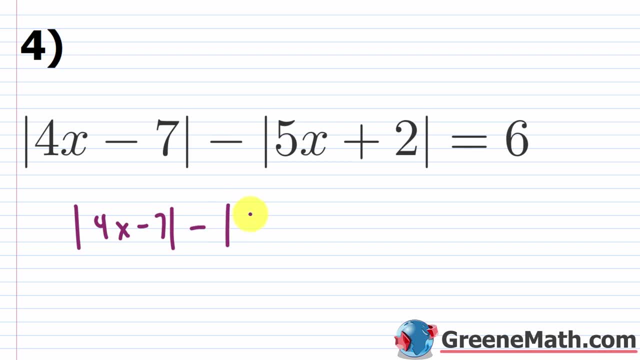 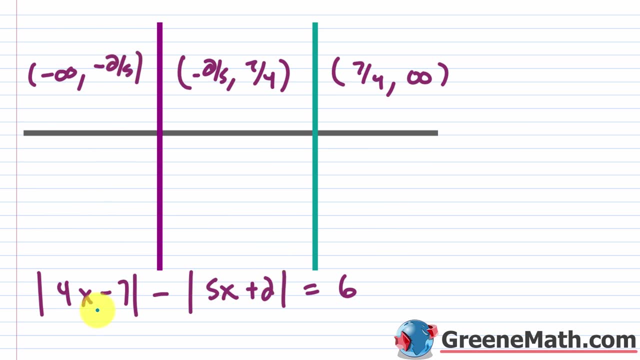 We have the absolute value of four X minus seven, then minus the absolute value of five X plus two, Then this equals six. Coming back here again in this interval, right here, both of these guys are going to be negative. So I want the negative of this quantity. 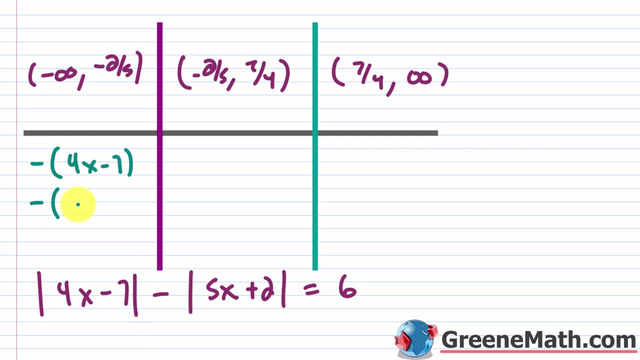 four X minus seven. And then I want the negative of this quantity: five X and then plus two. Then for this one right here, this guy will be positive, or you could say non-negative if you included this. So I'll just have the five X plus two here. 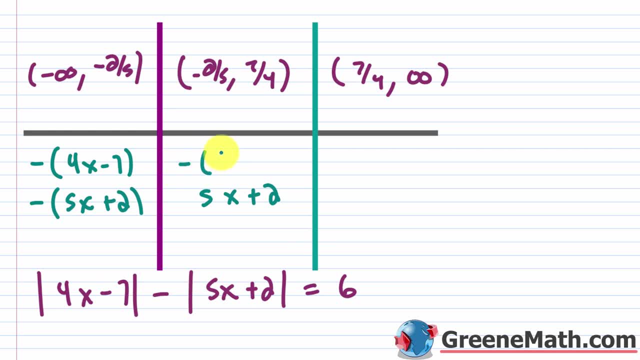 And this guy is still going to be negative. So the negative of this quantity: four X minus seven. And then in this guy, right here again, if you included this, then this guy would be non-negative and the other guy would be positive. 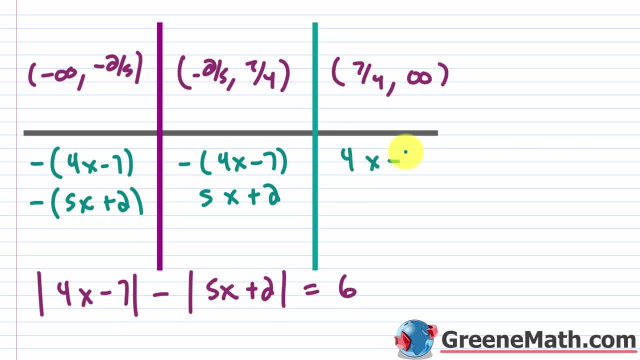 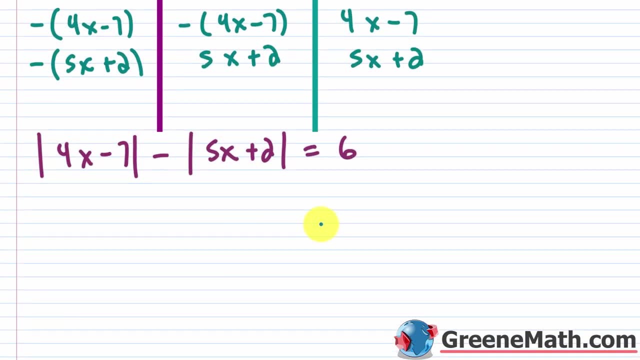 But if you exclude it, like I did, they're both positive. So four X minus seven: again, it doesn't change your answer if you're included or included, and then you have five X plus two. Okay, So let's go through and set up our equations. 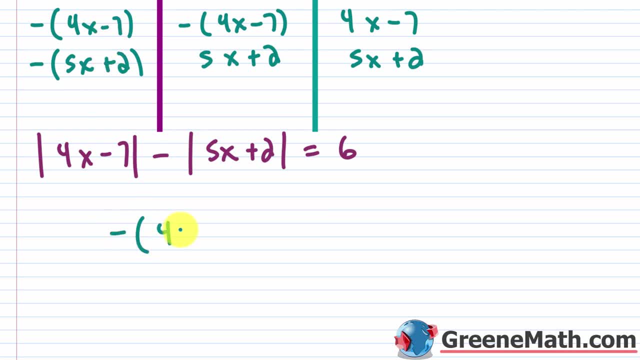 So in the first case they're both negative. So you want the negative of this quantity- four X minus seven, and then you have a minus. So you have to be really careful here. This is minus, And then you want the negative of this. 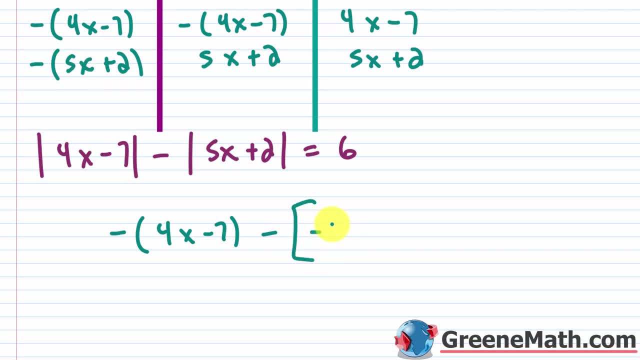 So let me put this inside of brackets or something, So I don't make a mistake. So the negative of this quantity five X plus two. just be really careful: if you have a negative, Okay, Then this equals six. So here I'm going to distribute this negative to each. 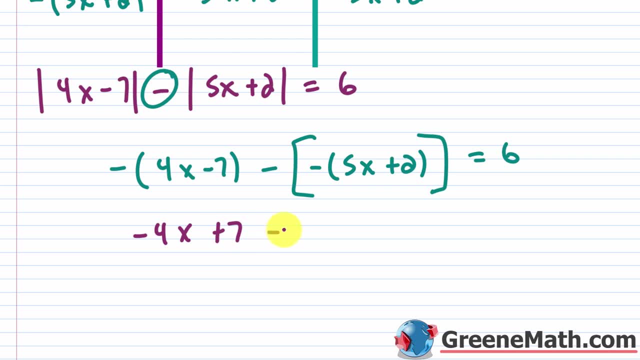 So this is negative four X and then plus seven, And then I'll put my minus sign out in front And then inside of here this would be negative five X and then minus two, And then to distribute this negative, this would be a plus. 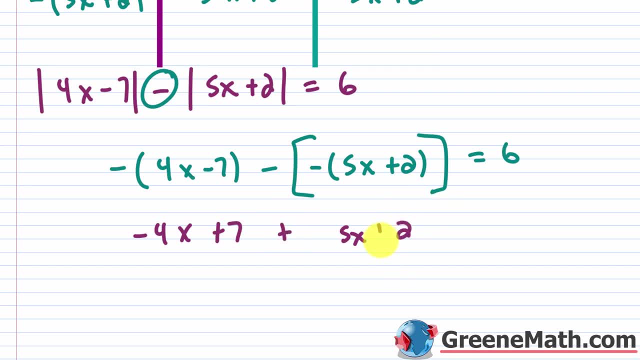 And then this would be a plus also. Okay, So make sure you use brackets or parentheses So you don't make a sign mistake With something like this. So then this equals six. Okay, So negative four X plus five X is just X. 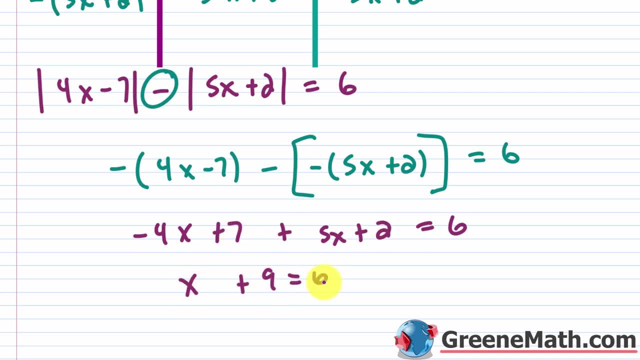 And then seven plus two is nine. So plus nine in this equals six. Let's subtract nine away from each side. We'll cancel this and say that X is equal to six minus nine is negative three. So let's say X is equal to negative three. 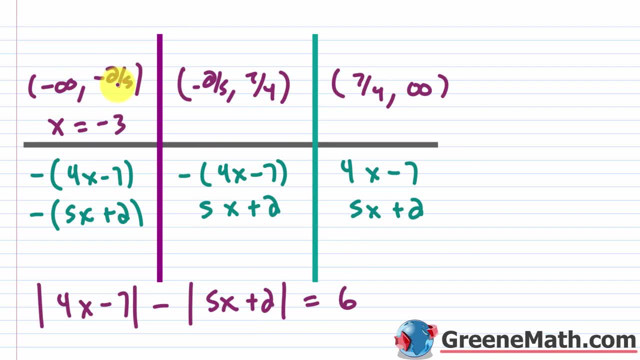 Now is that in this interval- Again, this is anything that's less than negative two fifths and negative three would be in that interval, So we can accept this solution. So let's look at this interval here between negative two fifths and seven fourths. 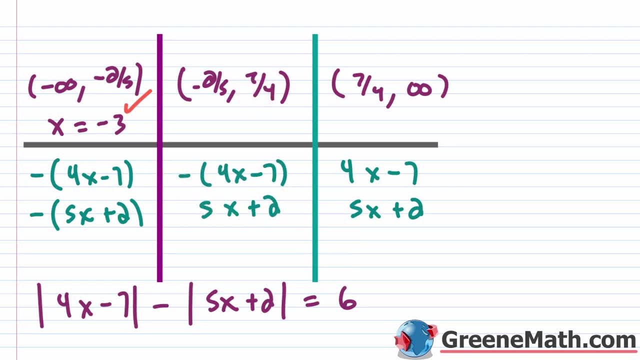 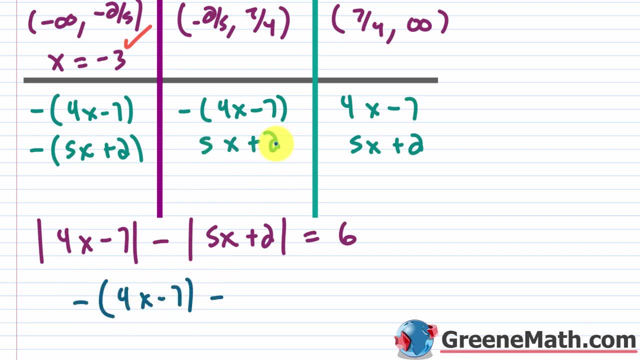 So we have that this guy is negative and this guy is positive. Okay, So let's take this first guy and say it's the negative of the quantity four X minus seven, then minus. now this guy's positive here, But again, because you have this negative here. 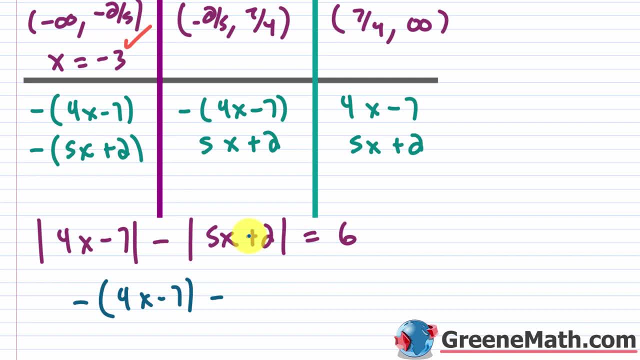 you have to subtract the whole thing away. So this is really easy to make a mistake on. Go ahead and wrap this in parentheses so that you don't make a sign mistake, because you have to subtract away five, X and then also two. then this equals six. 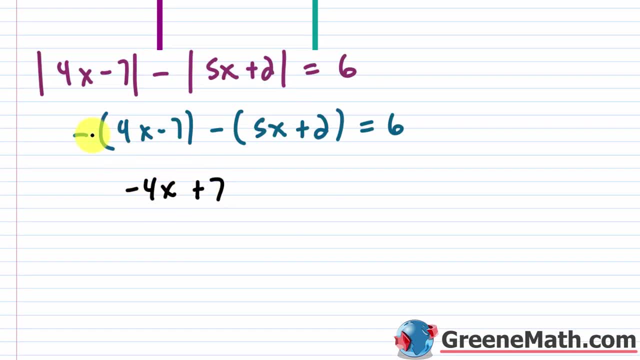 So here we'll have negative, negative four, X, and then plus seven again, just distributing the negative to each, And then I'm going to do the same thing here. So this is minus five, X and the minus two, and this equals six. Okay, 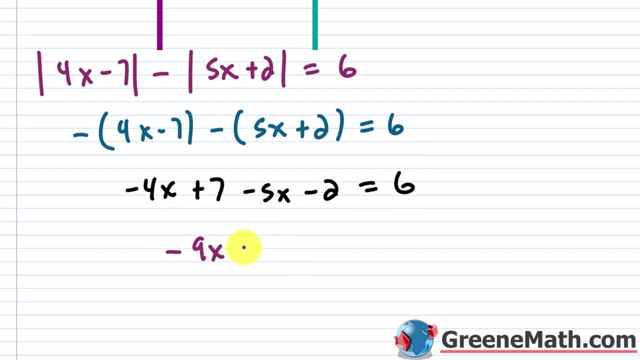 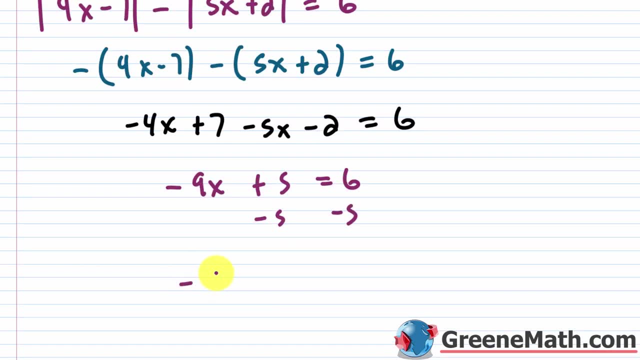 So negative four X minus five. X is negative nine X. and then seven minus two is going to be five. So plus five this equals six. We'll subtract five away from each side. We'll say: negative nine X is equal to six minus five is going to be one. 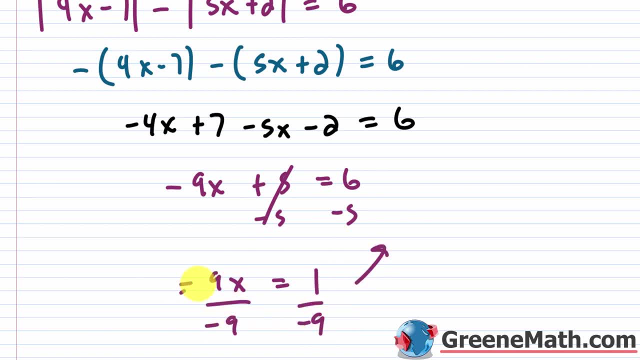 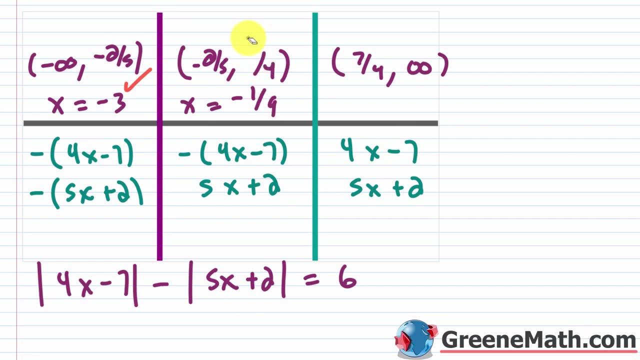 And then I'll divide both sides by negative nine. We'll say that this cancel cancels. X is equal to negative one ninth. So let's put: X is equal to negative one ninth. So is that in this interval, Well, negative. two divided by five is negative 0.4.. 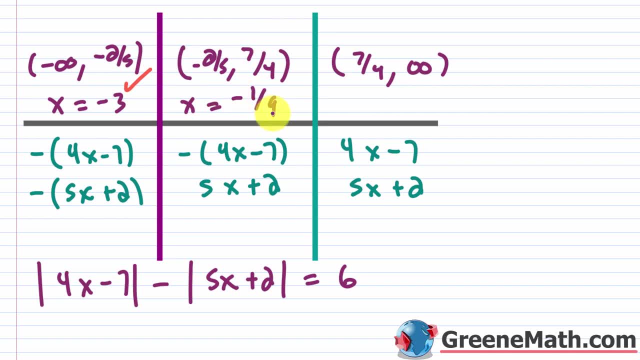 Okay, As a decimal, And then this negative one over nine, that's negative 0.1 repeating. Okay. So this value right here, this negative one over nine, is a larger value or is to the right of this negative two over five and it's to the left of this seven fourths. 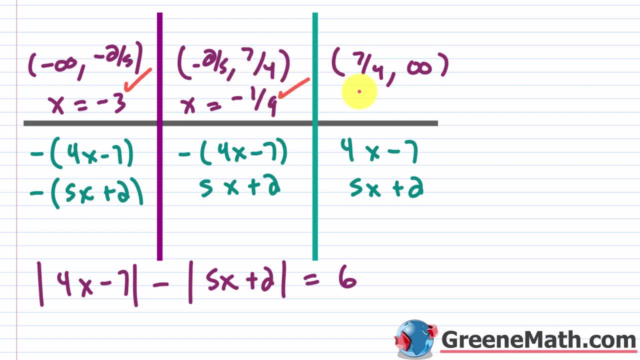 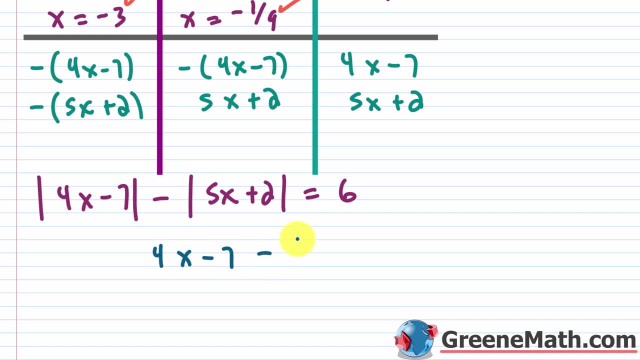 Okay, So we can actually except this solution. Okay, Let's look at this last interval. In this case we can just drop the absolute value bars in each case, So we'll have four X minus seven and then minus again when I drop this. 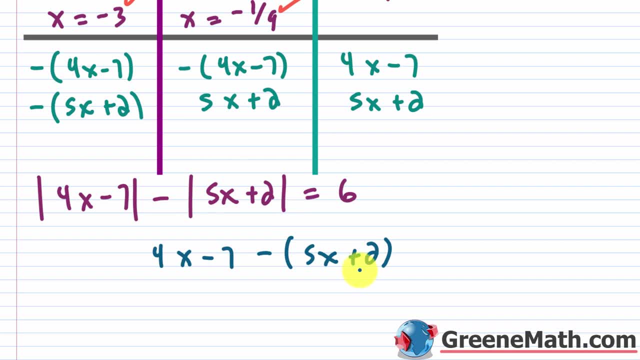 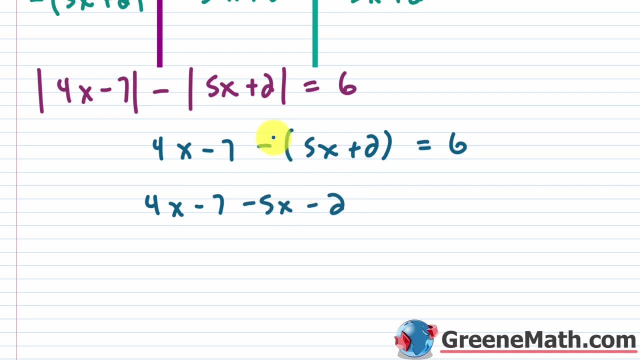 make sure to wrap this in parentheses. I want to subtract the whole thing away. Then this equals six. So here you'll have four X minus seven, then again minus five X and then minus two. just distributing this to each, and this equals six. 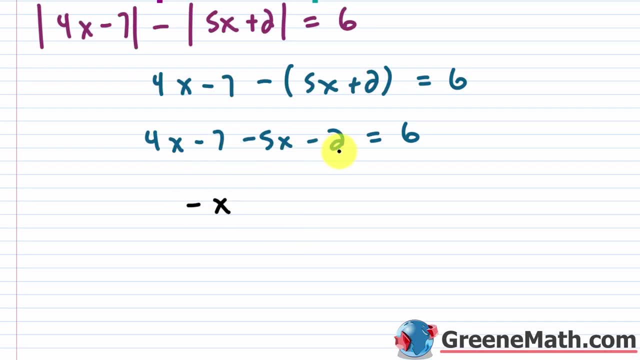 Okay, So four X minus five X is going to be negative X and then negative. seven minus two is going to be negative nine. This equals six. So we're going to add nine to both sides of the equation. This cancels. You get negative. X is equal to six plus nine is 15.. 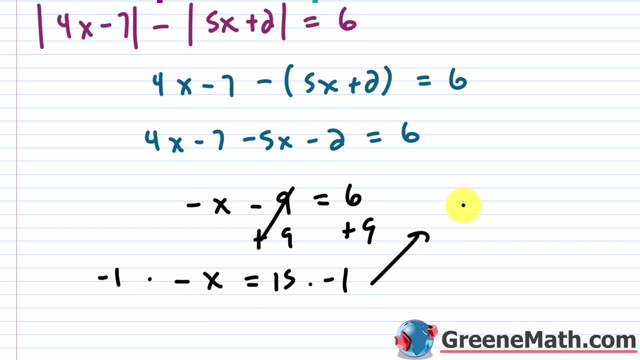 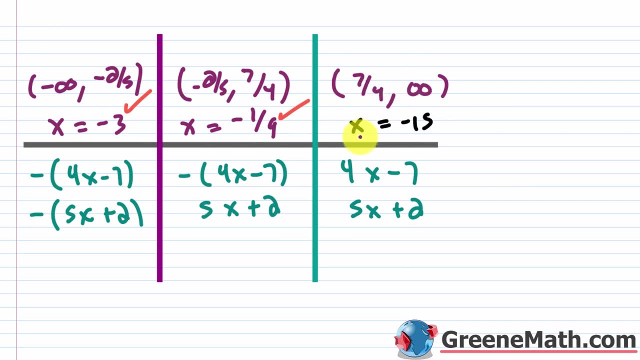 Let's multiply both sides by negative one, And that's going to give me that X is equal to negative 15.. So let's put: X is equal to negative 15.. Now, obviously this is not in this interval, so you can just reject this solution. 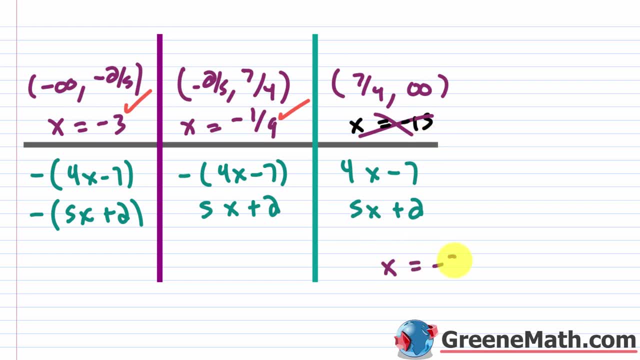 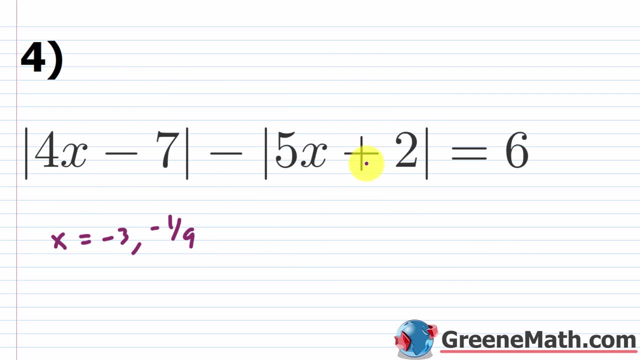 So your valid solutions. here you would say that X is equal to negative three or X is equal to negative one, ninth, Let's put that there And again. you can pause the video and check each one of these solutions and verify that they work. 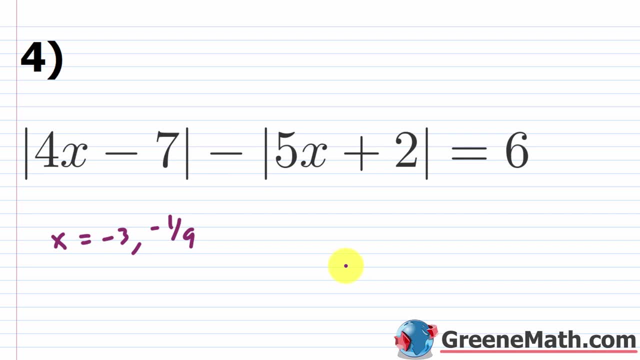 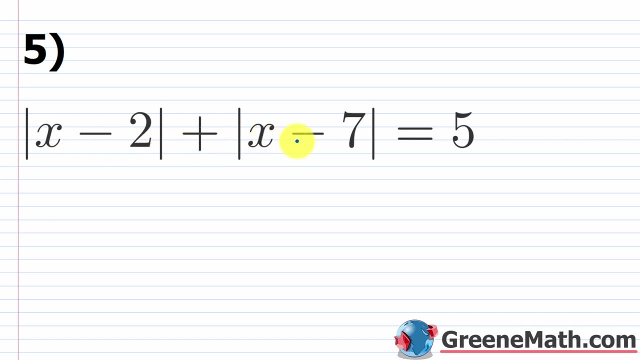 And you can also check that X equals negative. 15 does not work. All right, let's take a look at problem number five now. So we have the absolute value of X minus two, then plus the absolute value of X minus seven, and this equals five. 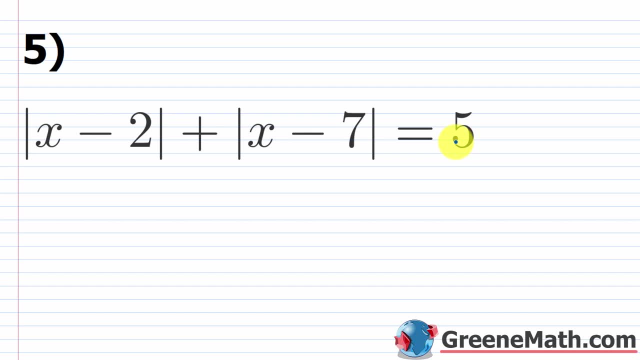 So this problem is a bit tricky, So maybe you tried to solve it and you couldn't get it, So let's just go through it here. I'm going to start in our usual way. I'm going to think about X minus two. 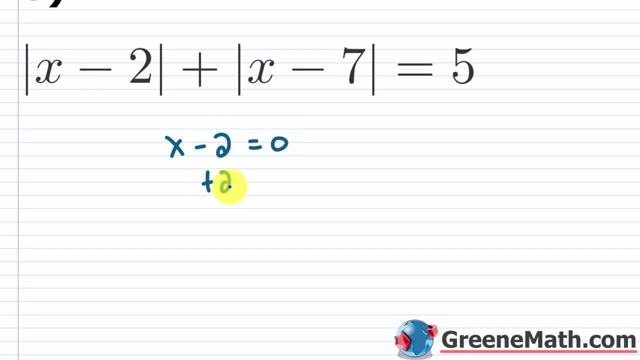 Basically, where's that equal to zero? So let's set that equal to zero. We'll add two to both sides of the equation. We'll cancel that. So we'll say X is equal to two. So we know at this point that, basically, if X was two, 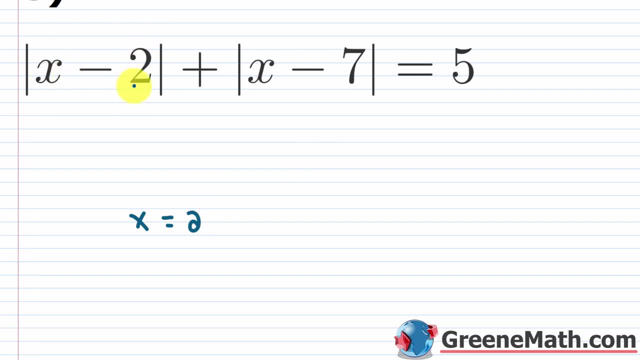 then this would be zero, right? If X was something greater than two, this would be positive, And if X was something that was less than two, this would be negative. All right, let's slide this over here. Then we also have this X minus seven. 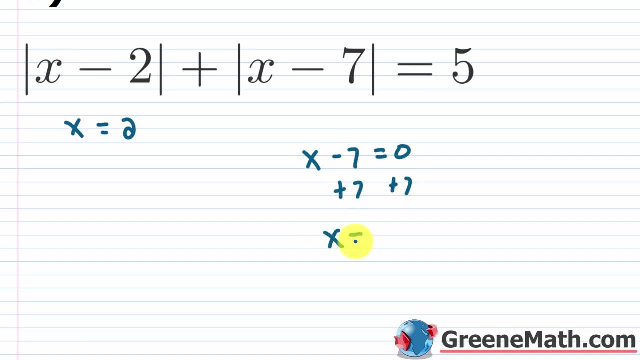 Let's set that equal to zero. add seven to both sides. We know this is X is equal to seven. Okay, So again, if X was seven, this is zero. If it's greater than seven, this is positive, And if it's less than seven. 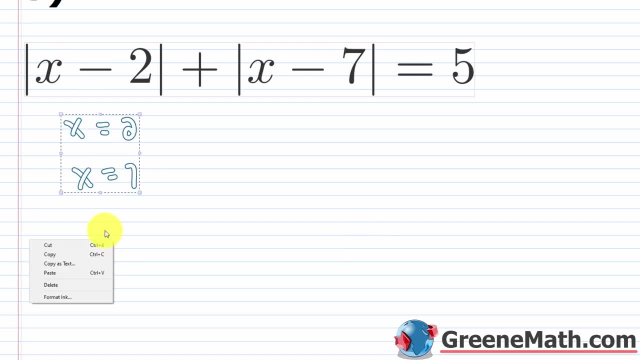 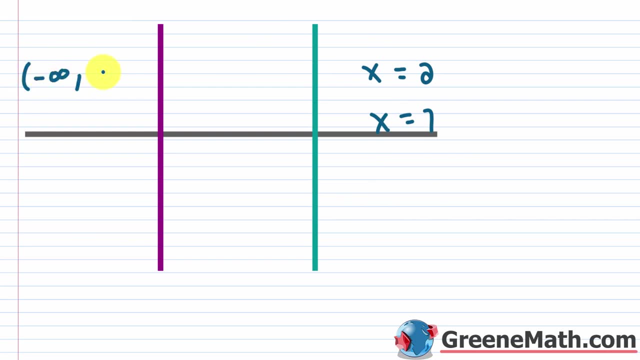 then this is negative. Let's put: X is equal to seven here. So let's go to the table and let's set up our intervals. So you're going to have one that's from negative infinity going up to an excluding two, And then I'm going to do this in two ways, just to show. 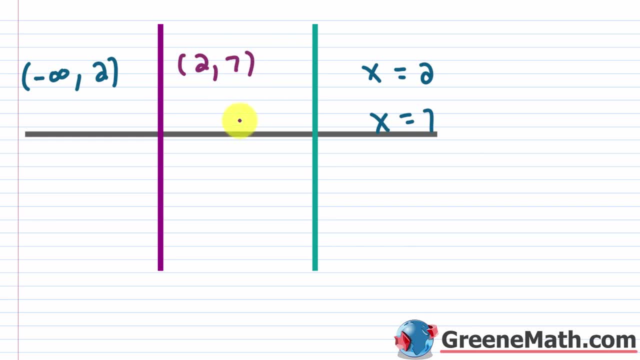 you the difference. So here I'm going to go between two and seven, And with this one I'm going to go including two but excluding seven, So a lot of people prefer to do it this way. I'll show you the difference between the two and the seven. 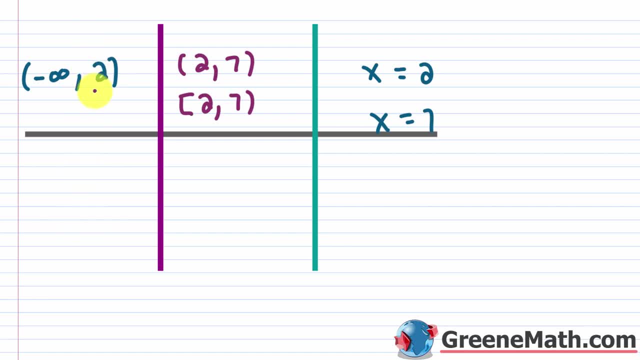 The two on this one, because what's going to happen is, when you solve this, you're going to end up with two as a solution, And then here you're going to get something weird. You're going to get an identity. So let's just keep going. 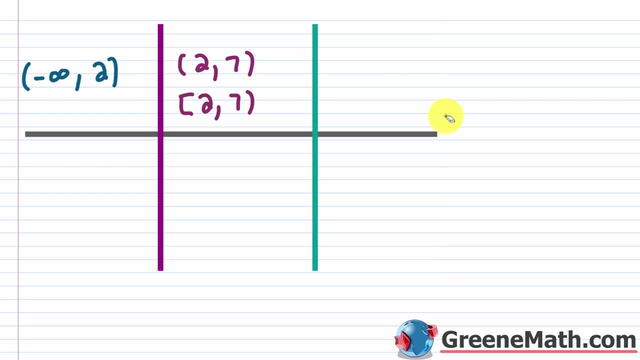 And then I'll explain more as we go. Then, over here, let's split this into two, So we'll say this is anything greater than seven, And I'll also include seven here for those that want to see it. Okay, Before I actually set anything up, 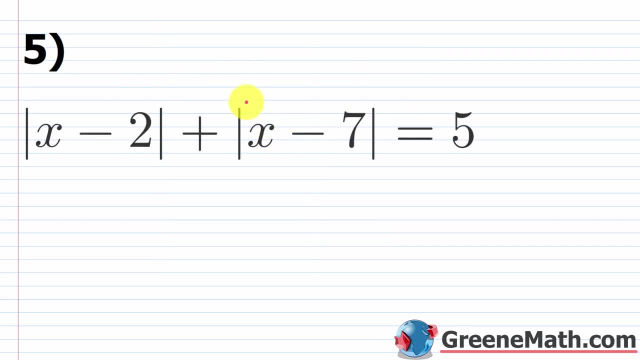 I want to go up and I want to advise you, if you're struggling with this problem, to take the left side of this and use an online graphing calculator like Desmos. it's completely free. I'm going to use math GV, So you can just type this in and you want to. 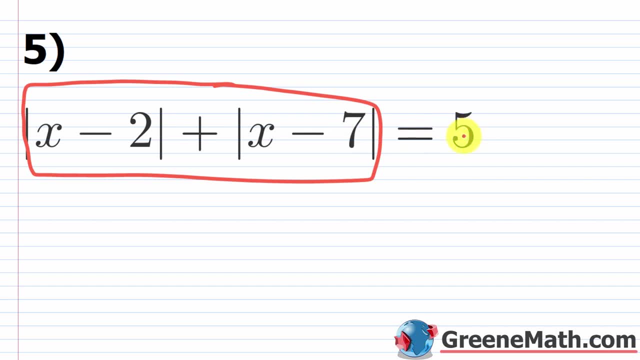 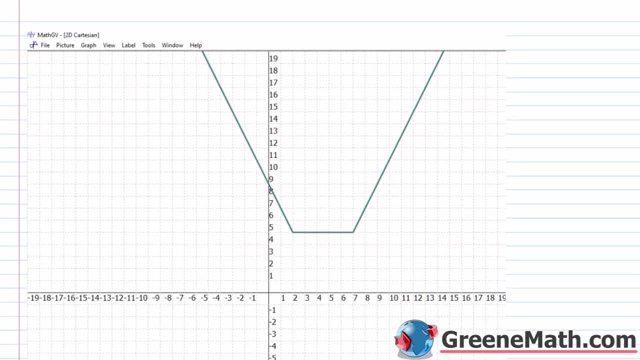 see where is that functions value equal to five? In other words, where's the Y value equal to five? So go find where the functions value is five and look for the associated X values. So I have used math GV to make a little graph. 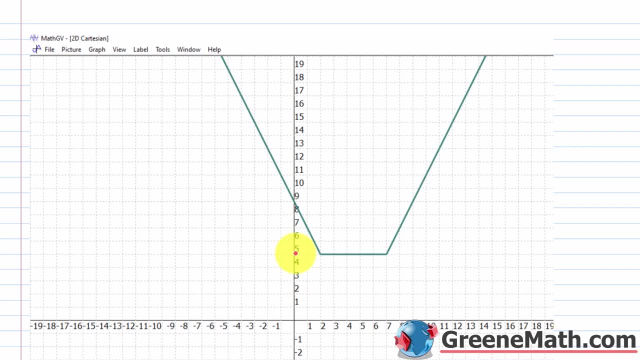 for us. And so again I'm looking for where the functions value is five. So I'm coming across and you'll see that it's right here, through, right here, And you can highlight the whole thing if you want. And basically that starts where there's an X value of two. 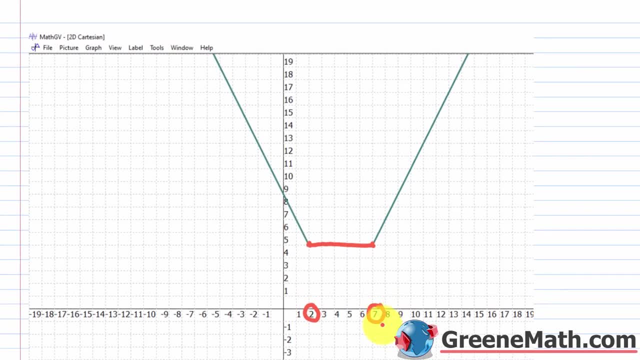 and continues through where there's an X value of seven. So graphically I can see that the solution is: X is greater than or equal to two and less than or equal to seven. So we know that from this graph. Now let's see if we can figure this out algebraically. 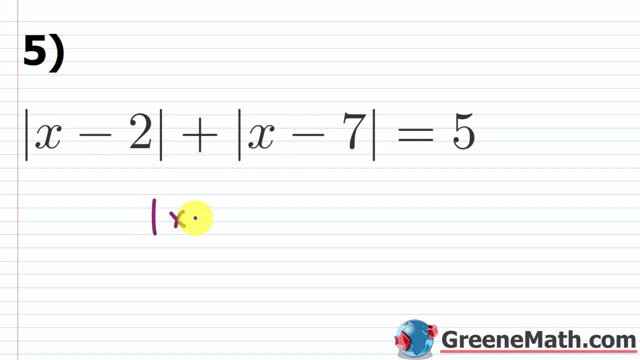 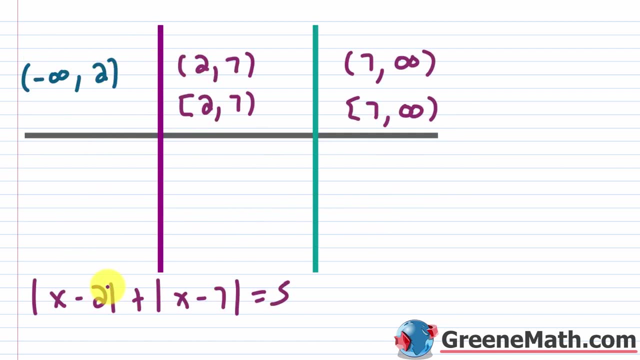 Let's come back up here and let's grab this guy. So we have the absolute value of X minus two plus the absolute value of X minus seven. This equals five. So in this first column I know that everything is negative, So I would have the negative of this quantity, X minus two. 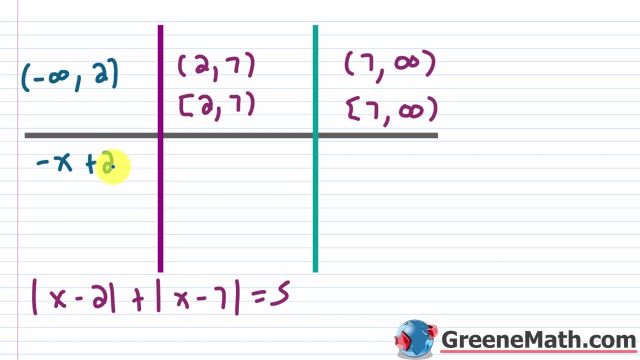 So that's negative X And then plus two. I just distributed the negative. Now here, whether you use this method or this method, basically you can just drop the absolute value bars. here You could say that it's not negative, here You could say it's positive. either way, 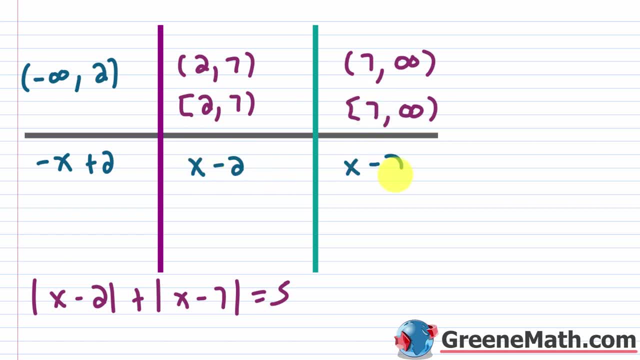 It's just X minus two, and then here it will be positive. So it's just X minus two. Okay, With this, X minus seven, it's going to be negative here and then also here, right, So I'm going to say that's negative X. 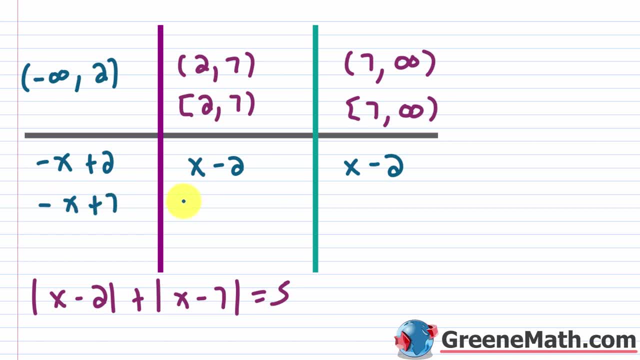 and then plus seven again, just distributing the negative to each guy. So then negative X plus seven. And then again, when I get here, whether I use this guy or this guy, it's either going to be non-negative with this case or positive with. 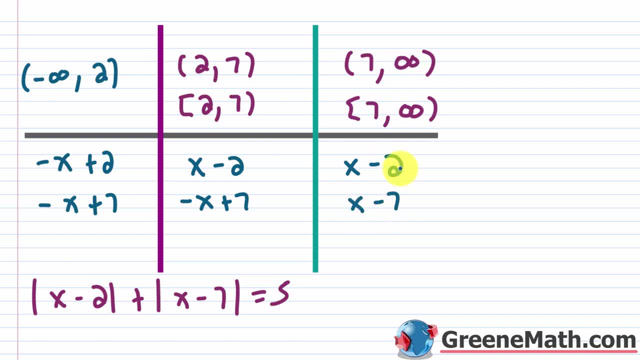 this case. either way, just drop the absolute value bars. It's X minus seven, So whichever one you want to do, Okay, So coming down here, I'm going to solve the first case and we're going to get something. that's a bit weird. 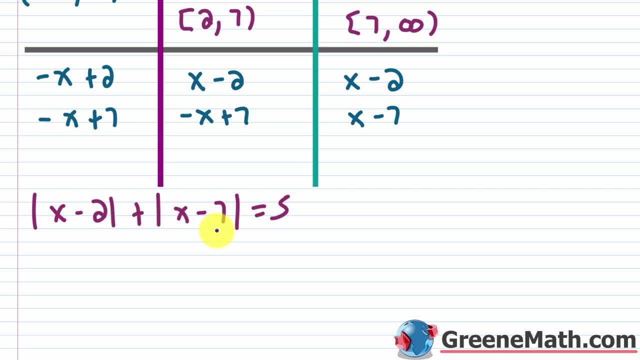 Okay, So the solution we're going to get is positive two. Okay, So I'm going to come through here and say this is negative X plus two, And then this is a plus sign here, So you can just go minus X plus seven. 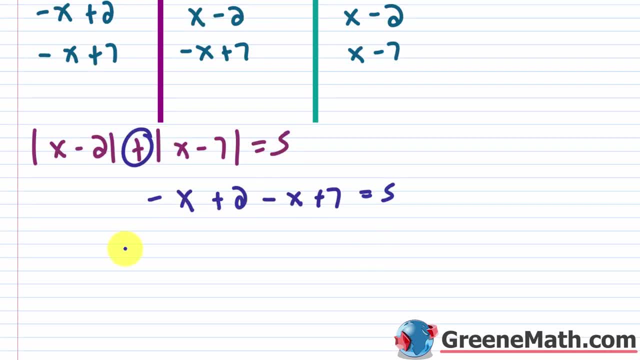 And this equals five. Let's just solve this really quickly: Negative X minus X would be negative two X, and then two plus seven would be nine, And this equals five less subtract nine away from each side. We'll cancel this. I'll just say this is negative two X is equal to five. 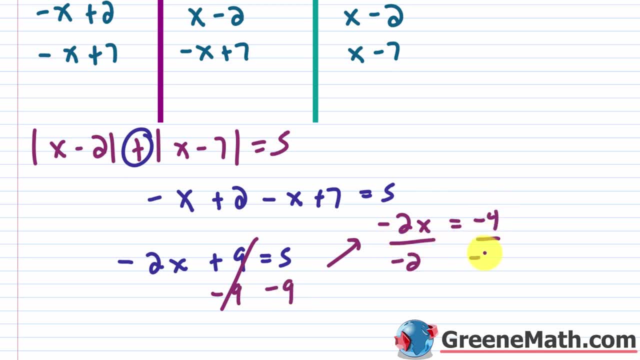 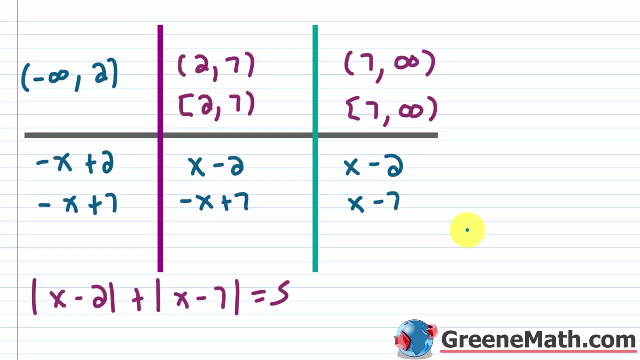 minus nine is going to be negative four. divide both sides by negative two. This would cancel, And we're going to see that X is equal to positive two. Okay, So does that work? Well, currently it doesn't right, Because in this interval, 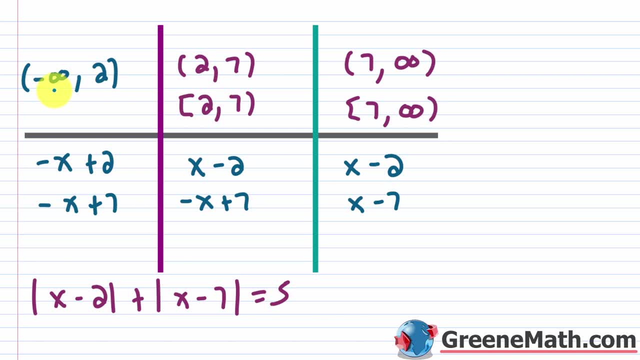 again, I'm coming from negative infinity and I'm going up to an excluding positive two. So I would say X equals two. That's going to have to get rejected right here. Okay, Now you might have some questions because, again, when we go back to the graph, 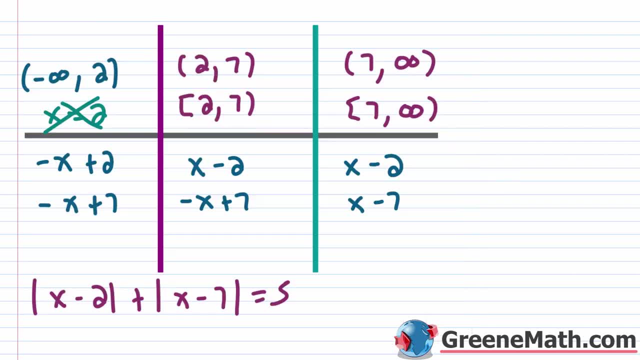 you can see that two is clearly included in the solution, And so a seven. So the way we're going to get that is basically when we think about this guy right here. So I'm going to solve this and I'll come back up and 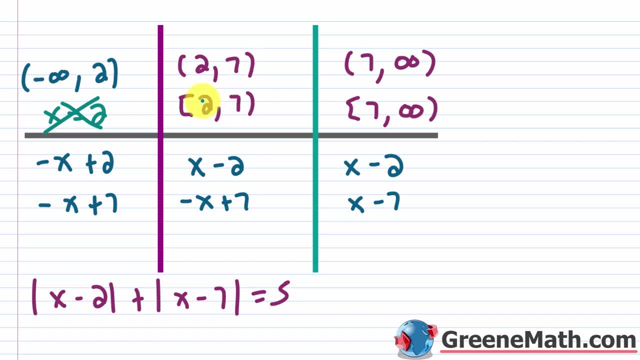 I'll talk about this scenario in this scenario. Okay, So this is where, if you're confused about including it or excluding it, this is where you can do it. You can get some clarification. Okay, So for this one, we would just do X minus two. 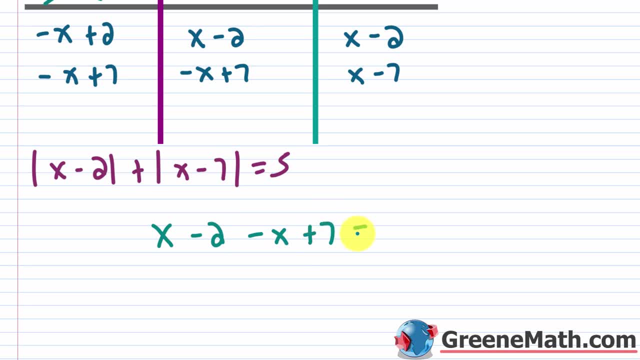 And then again, because this is a plus sign, I can just go minus X and then plus seven And this equals five. So if you have X minus X, that's zero right. So that's going to basically cancel. So this is going to go away. 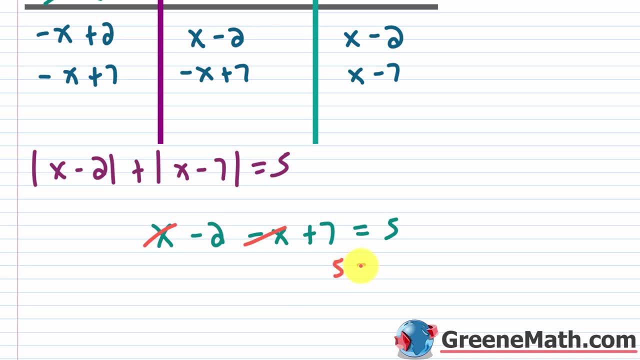 So now I have negative two plus seven, which is five. So you get five equals five. So we saw equations like this earlier on in the course. they're called identities. They're always true for any value of X, but we have to only consider the values of X. that 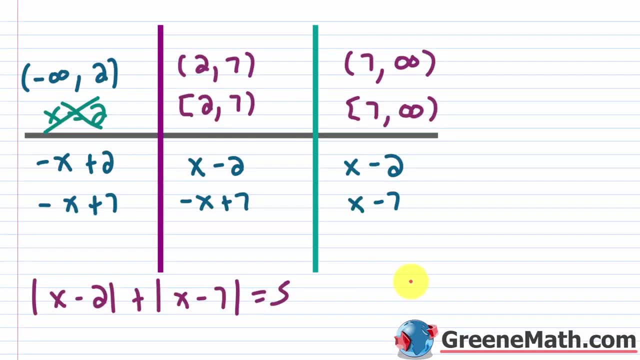 are in our interval. If I get something like this, I'm just basically going to say that this tells me that it's X is greater than two and less than seven. Okay, So here's where you have to make a decision If you're using this method right here. 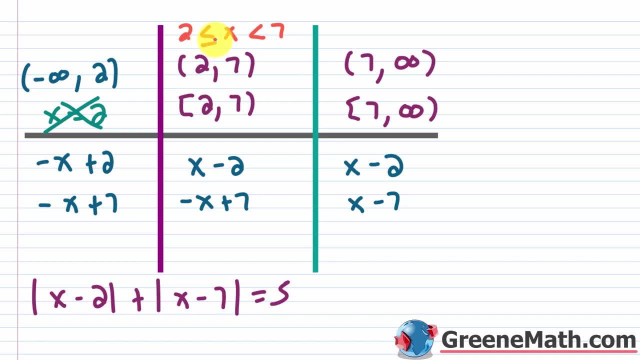 which again includes two. then at this point I can legally include two, right, Because, again, the setup is the same, whether I think about it this way or this way. right, If this was zero, well then I could just drop the absolute value bars. 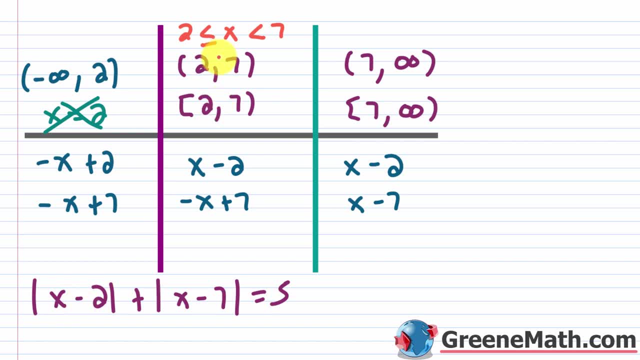 If it's positive again, I can also just drop the absolute value bars, So you can legally include that. Now, what I I always do is just use this and then I say, okay, does two work? I go back and plug it in. 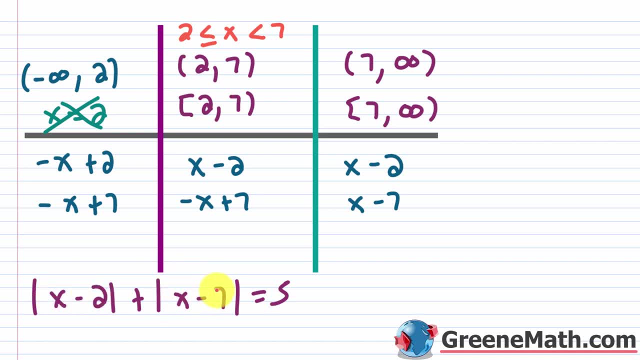 Two minus two would be zero. So basically, here you would have two minus seven, which is negative five, And then the absolute value of negative five would be five. right, This is five equals five. That's a true state. So that's how I would go about including two. 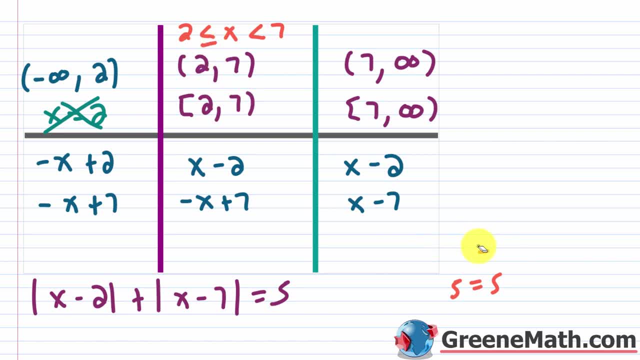 But again, if you want to do it this way, that's up to you. It's a little bit quicker Now. on the other end, you see that seven is excluded. right, It's excluded here and it's excluded here, But again. 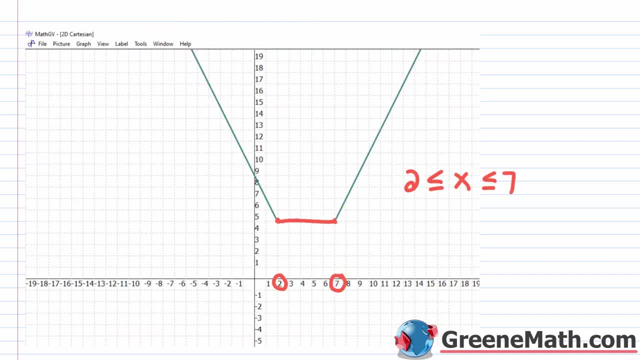 when we think about coming back to this graph, you'll see that seven is included. So how are we going to get that part of the answer? Well, that's going to come in here. So let's come down and let's solve this part. 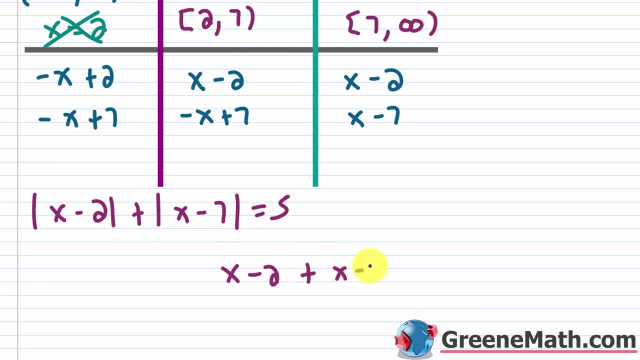 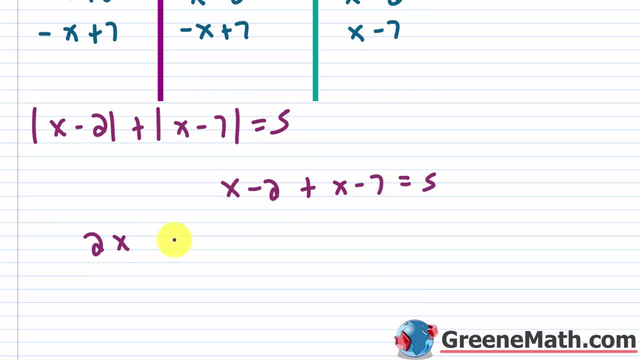 So we have X minus two, And then again this is a plus X minus seven, and this equals five. So here you're going to get X plus X, which is two X negative two minus seven is going to be negative nine, and this equals five. 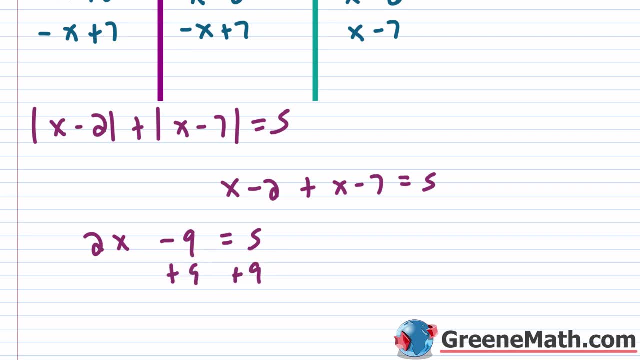 So what we'll do here is add nine to both sides of the equation. This will cancel And we'll say: this is two, X is equal to five plus two plus nine is 14.. Let's divide both sides of the equation by two. 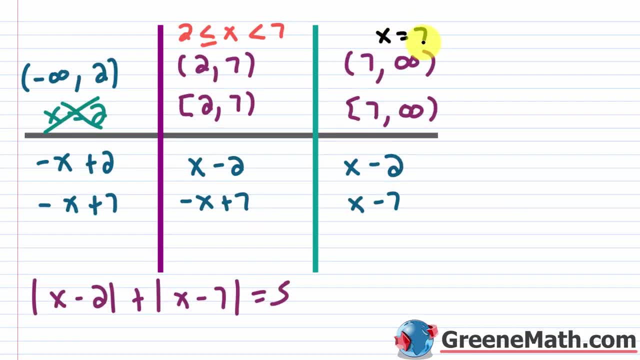 And we'll say that X is equal to seven. So coming back up here, I have: X equals seven. Okay, Now again, if you've included seven here, then you're done. Basically, you can just combine these and say that X is. 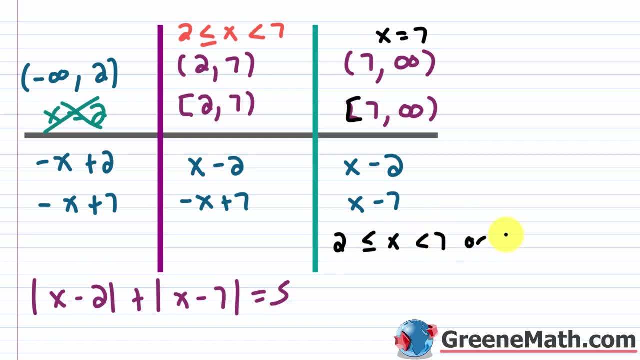 greater than or equal to two and less than seven, And then you would say: or X is equal to seven. Now, this is easy to combine, because you can just say that this is basically: X is greater than or equal to two and less than or equal to seven. 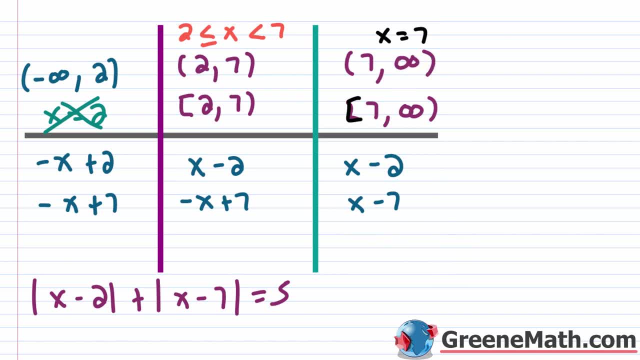 right, That's easy to combine. but let's say you did my method that I've been talking about. Well, here you're not done because technically, seven is not in there, So you'd have to take the extra step of plugging seven in to verify that it's going to work. 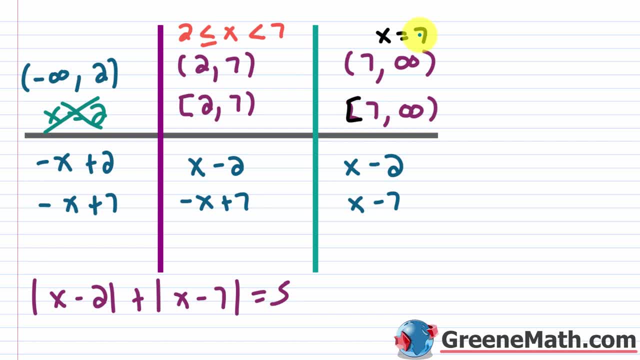 right, Just like I did with two. So in this particular case I would say that seven minus two is five, So you'd have the absolute value of five. And then this right here: seven minus seven is zero. So that's gone. 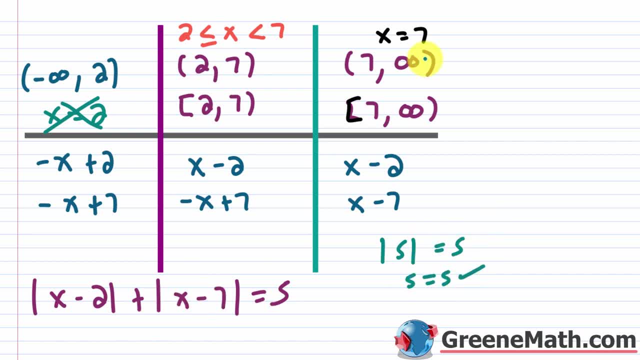 So the absolute value of five is equal to five. You get five equals five, So that works. So that's how I could verify that seven's part of the solution. So, again, just depending on the method you want to use, Okay. 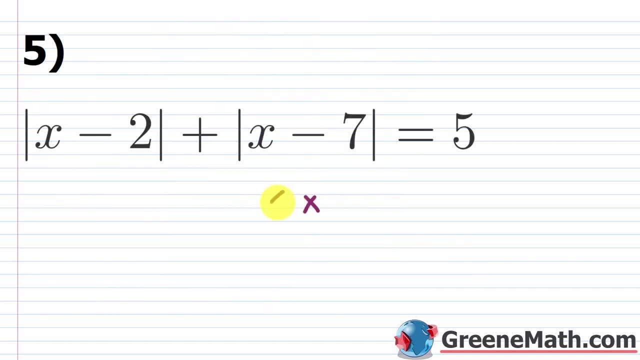 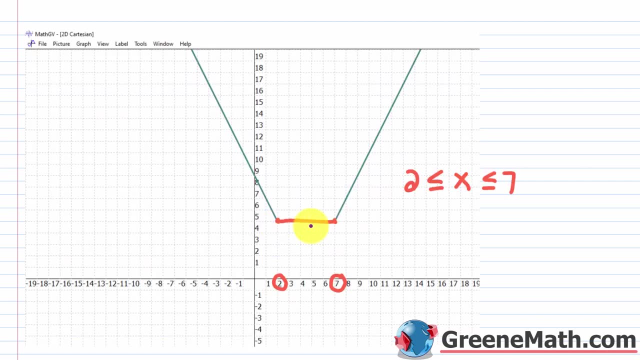 So let's go back up and let's write our solution. So we'll say: X is greater than or equal to two and less than or equal to seven. And again, if you have doubts about this, you can again just go to the graph and see that that's the solution. 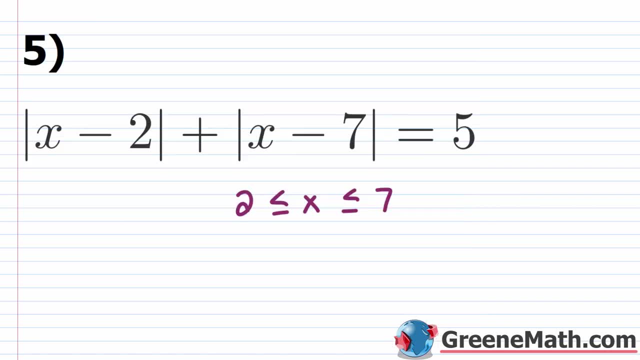 You can also pick values that are in that interval, So between two and seven, including two and seven. we already saw two and seven work, but you can just pick something like three or 3.5 or 3.25 or whatever you want. 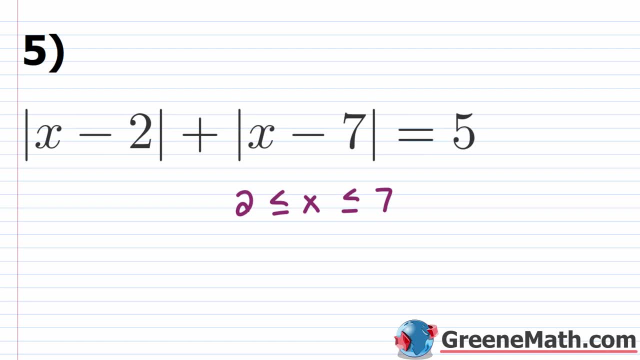 anything in that interval, plug it in and verify that you get a true statement. Let's just pick one real quick and then we'll conclude the problem. So let's just say we chose three, So three minus two would be one. So this is the answer. 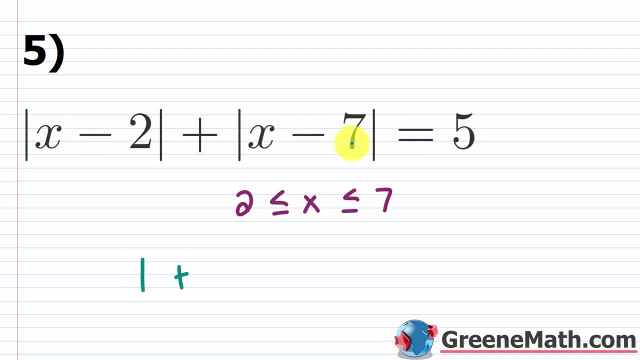 The absolute value of one, which is one. then plus three, minus seven, would be negative four. The absolute value of negative four is four. Does that equal five? Yes, you get. five equals five. So this is a true state. So this would be our solution. 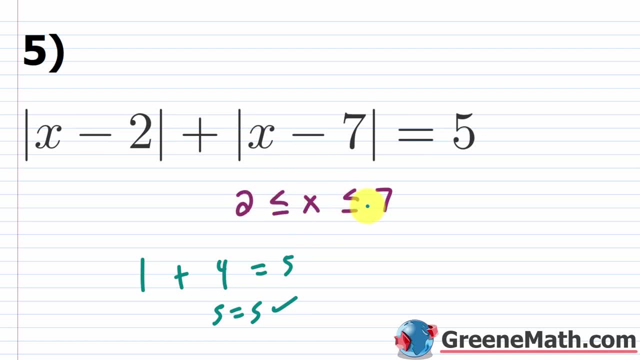 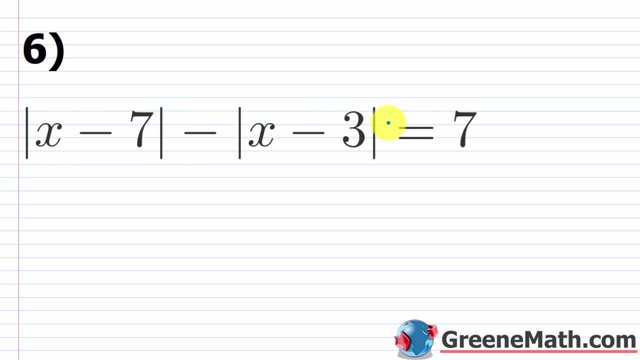 X is greater than or equal to two and less than or equal to seven. All right, let's take a look at problem six now. So here we have the absolute value of X minus seven, then minus the absolute value of X minus three. 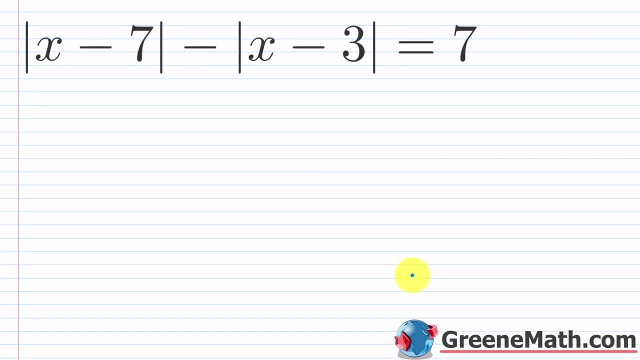 and this equals seven. So in this particular case I'm just going to tell you in advance you're not going to get a solution. So I thought we would look at an example like this. So here we can kind of speed through. 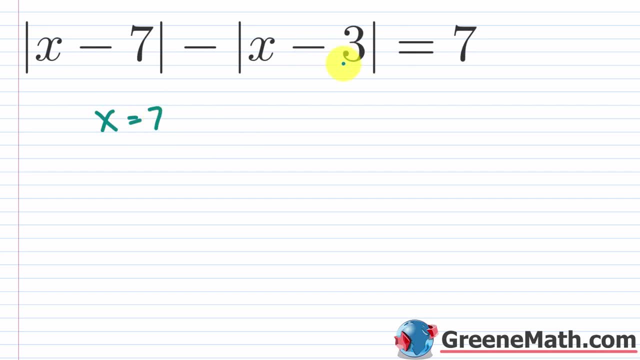 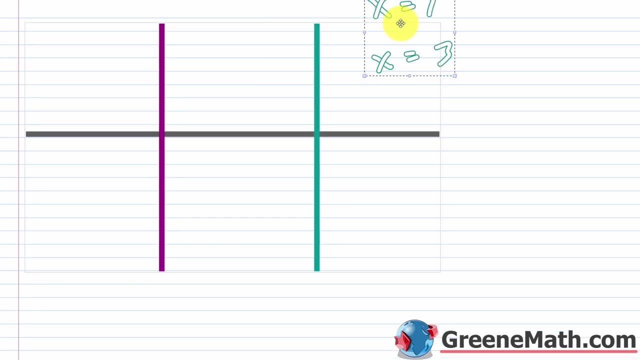 This. we know that this one is just X is equal to seven, And for this one it's just X is equal to three. I think we don't have to waste time with that anymore. Let's come down here. Let's paste that here. 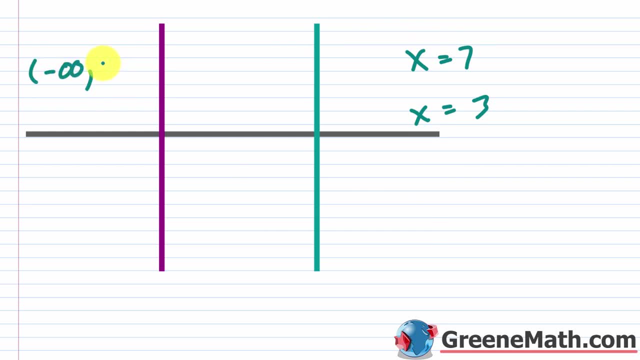 So I'm gonna have an interval from negative infinity up to an excluding three, And then here it's going to be between three and seven, And again, if you want to include three, you can include three. there It's not going to matter. 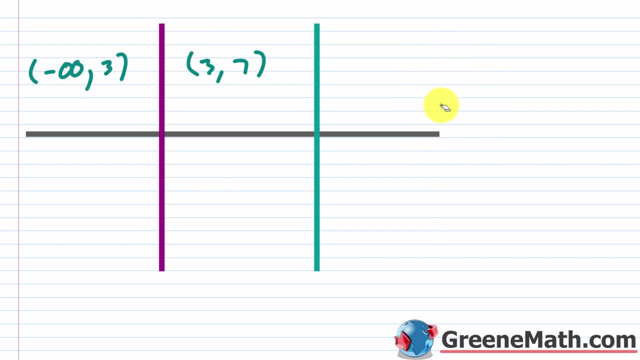 but I'm just going to exclude it. And then you want anything that's greater than seven, right here And then basically here. if you wanted to, you could include seven, but once again, I'm going to exclude it, Okay. 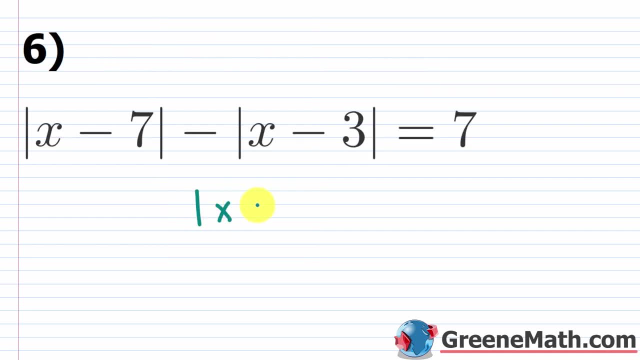 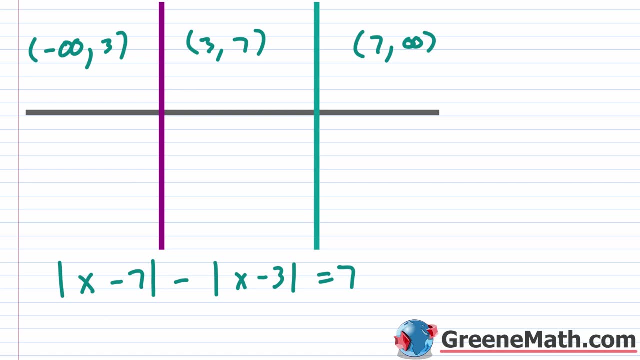 Let's look at our equation. I'm just going to copy this. So this is the absolute value of X minus seven, then minus the absolute value of X minus three, and this equals seven. And let's go through our cases. So in this first guy, 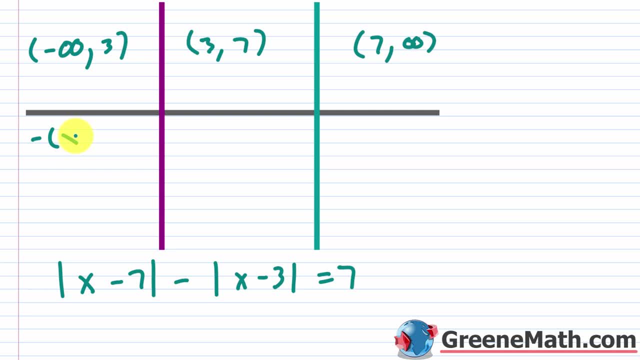 this leftmost guy. they're both negative, So I want the negative of the quantity X minus seven. Let me just distribute this Now: this is negative X plus seven And then basically I'm going to have that again right here. So this is negative X plus seven. 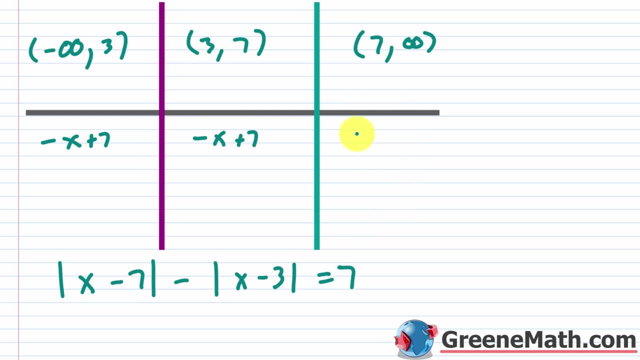 Again. and then in this guy right here, this is going to be positive. So I'm going to say: this is X minus seven. Okay, For this next guy, you have X minus three. So that's going to be negative here. 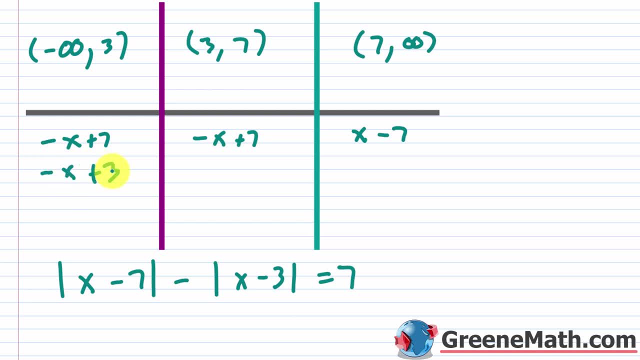 So that's the negative of X and then plus three. So I just distributed a negative to the X and then the negative three to get this, And then here it's going to be positive and here it's going to be positive. So it's just X minus three. 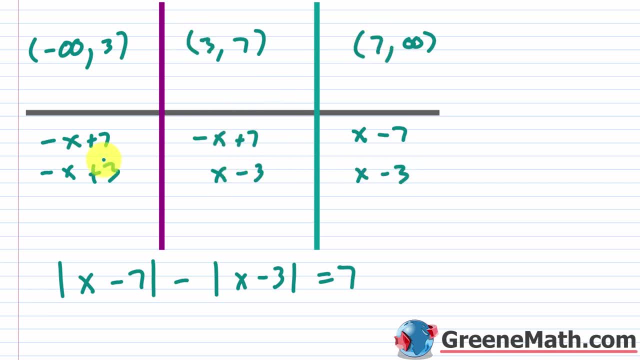 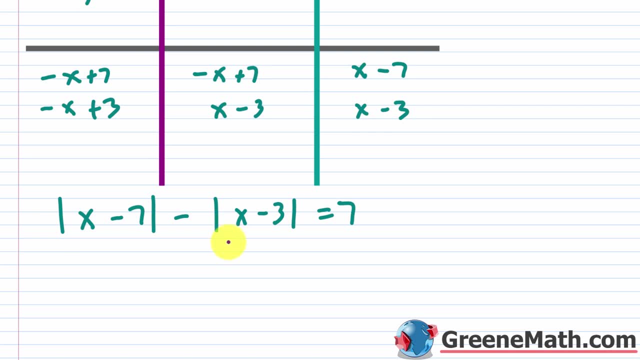 And again, if you're including things like the three and the seven, nothing is going to change here. Okay, So it won't make any difference Whatsoever. So let's go through and set up our first equation. So this is going to be negative X plus seven. 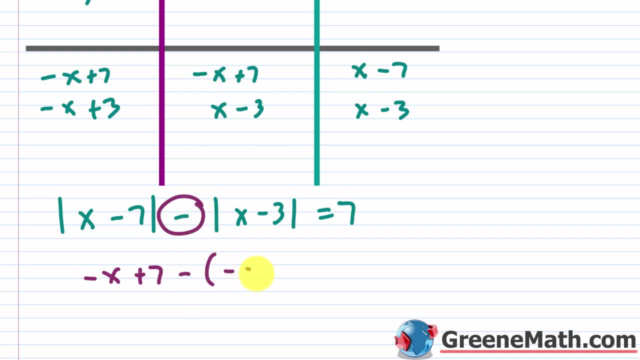 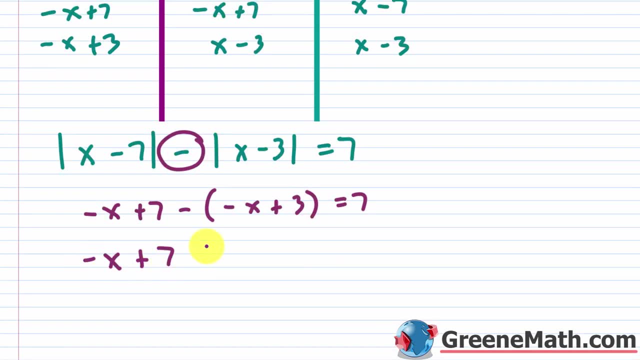 You have to be really careful because of this minus, So minus the quantity negative X plus three, and this equals seven. So let's solve this real quick. This is negative X plus your seven, And this is the negative of negative X, which is plus X. 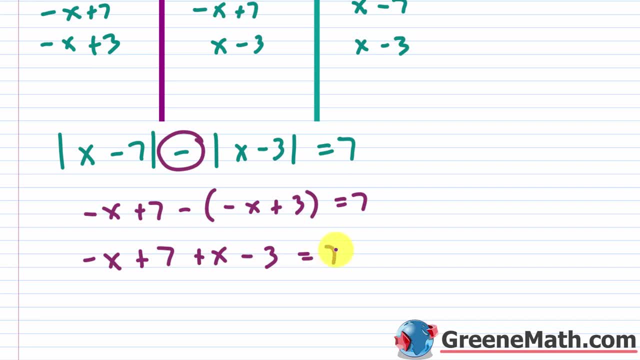 And then the negative of three, which is negative three. This equals seven. And then from here you have negative X plus X. that's gone, basically right, Those are going to cancel. So you have seven minus three, which is four. So you get four equals seven. 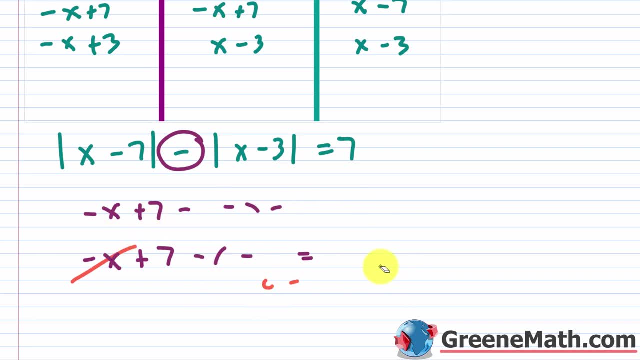 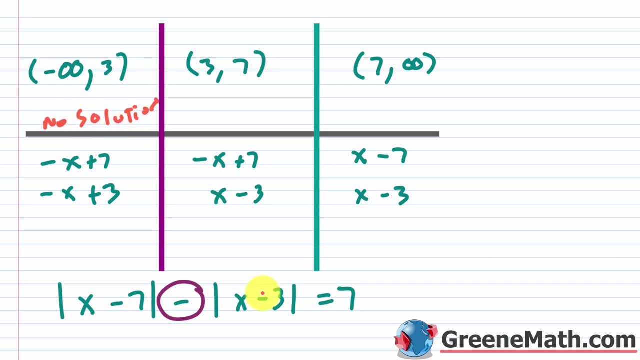 which is a false statement, right? So this is false. So there's no solution in that first one. You can come up here and just put no solution if you want, or you can just leave it blank. I'll just put no solution, like that. 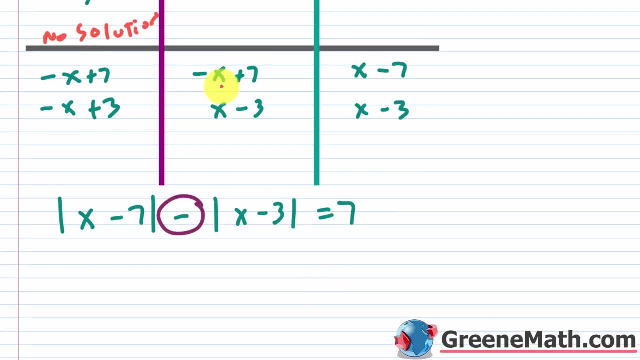 Okay, For the next guy, we're trying to get between three and seven. So this is negative X plus seven And then minus again. you have to be careful here. You're plugging in an X minus three where this is right here. 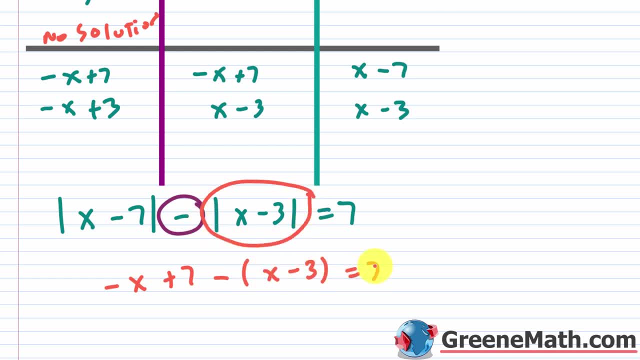 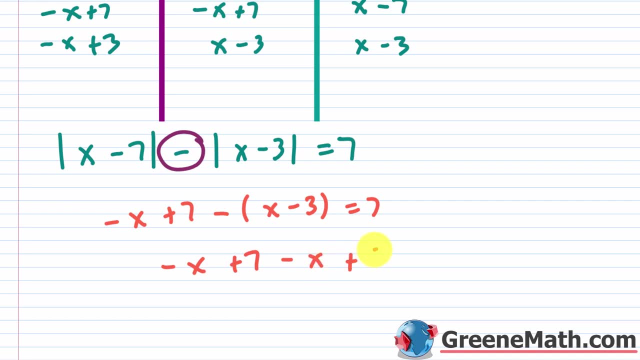 but you have to wrap it in parentheses, You have to subtract the whole thing The way. that's very important. So this would give me negative X and then plus seven and then basically minus X and then plus three, and this equals seven. So negative X minus X would be negative two X, and then seven plus three is 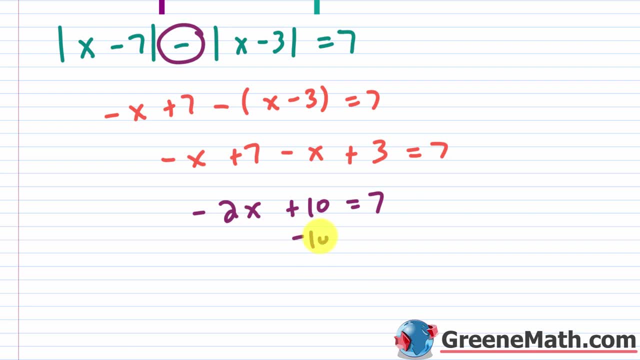 10.. So plus 10 and this equals seven. So let's subtract 10 away from each side. Let's cancel this. You get negative two. X is equal to seven. minus 10 is going to be negative three. Let's divide both sides by negative two. 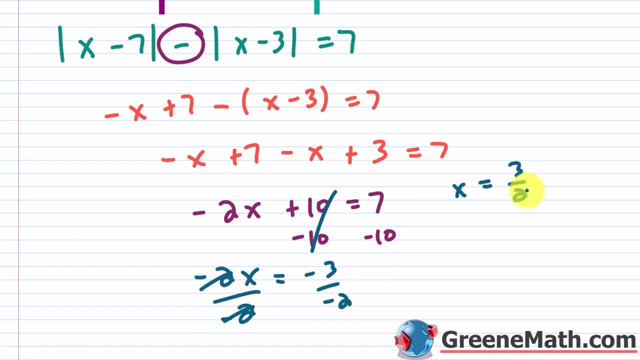 This cancels And you're going to get: X is equal to three halves, So let's put X is equal to three halves. three halves or 1.5 is to the left of three on the number line, So this is not going to work. 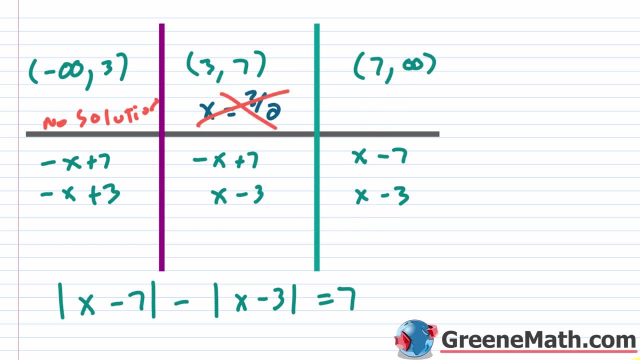 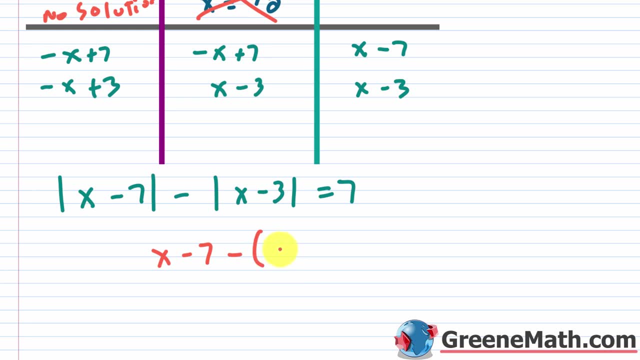 This has to be rejected. Okay, So now we're down to the last guy. We're just going to drop the absolute value bars in each case. So X minus seven and then minus again- make sure you use parentheses here- the quantity X minus three and this equals seven. 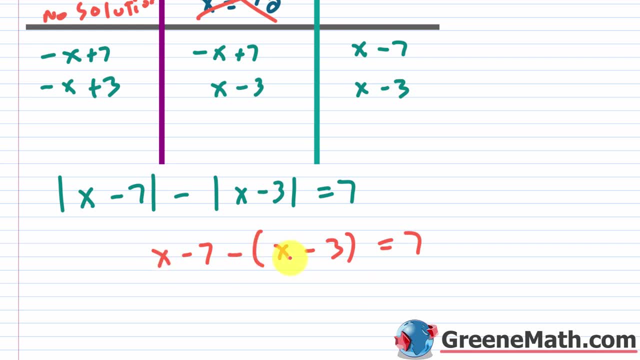 I think you can see this is not going to work because you can have X minus an X, So that is going to drop out And this is not going to be seven over here. So it's not going to be an identity, It's going to be a contradiction. 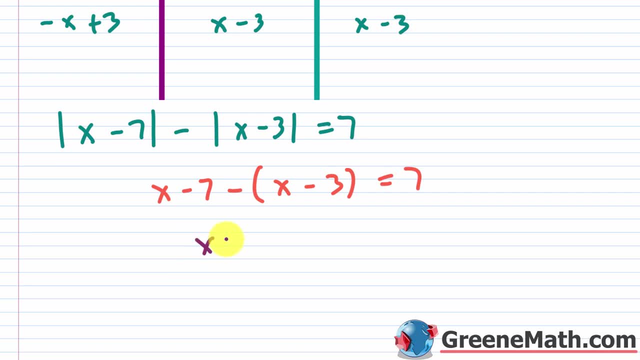 right. So it's not going to work, but let's just go through it for completeness. This is X minus seven, and then minus X, and then plus three is equal seven. Again. this and this that's going to cancel right. 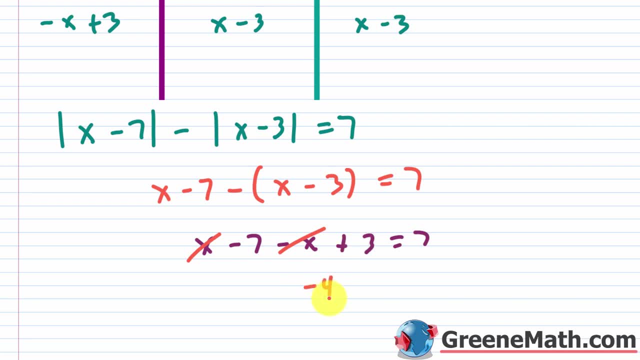 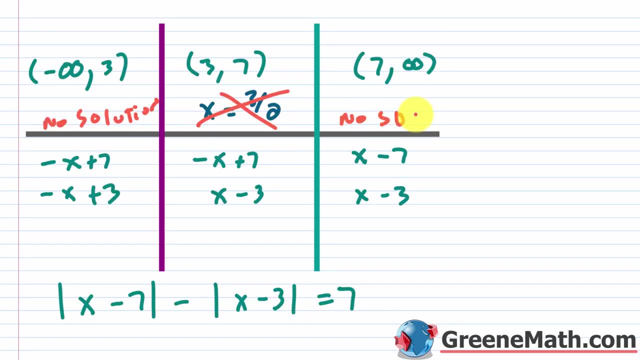 X minus X is zero. negative seven plus three, That's going to be negative four. So you get negative four is equal to seven, which is false, right? So there's no solution there. So, coming back, I'm just going to write that there's no solution. 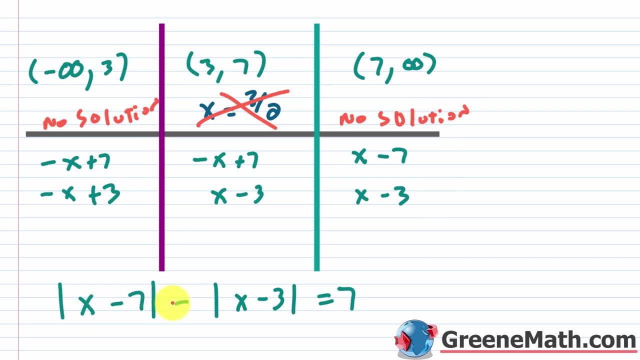 right. So this guy, this absolute value of X minus seven, then minus the absolute value of X minus three, that's never going to be equal to seven. So, coming back, I'm just going to put that there's no solution. And again, 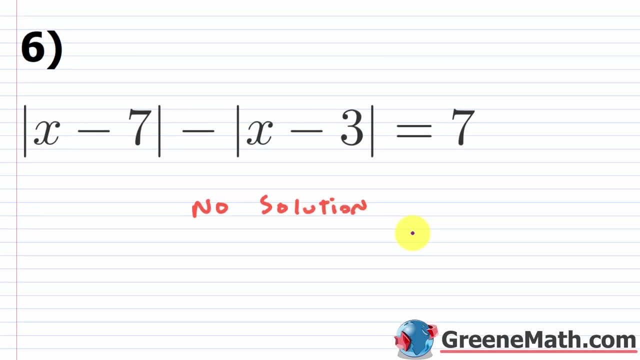 if you're a bit lost on this one or you have some doubts, you can always take this right here, this left-hand side, and you can graph it. You can type it into Desmos or any online calculator. as it is. So, the absolute value of X minus seven: 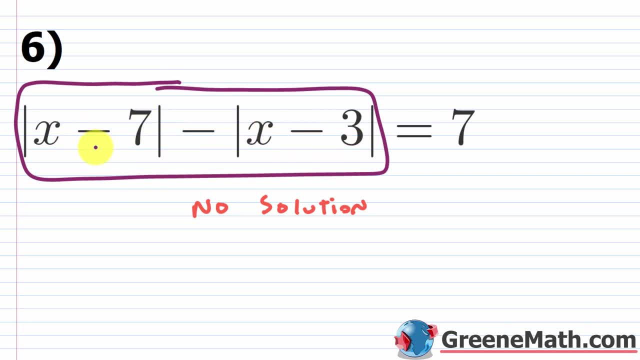 then minus the absolute value of X minus three, you could put F of X is equal to that, If you want it to, you put Y is equal to that, If you want it to. it's all going to produce the same graph. 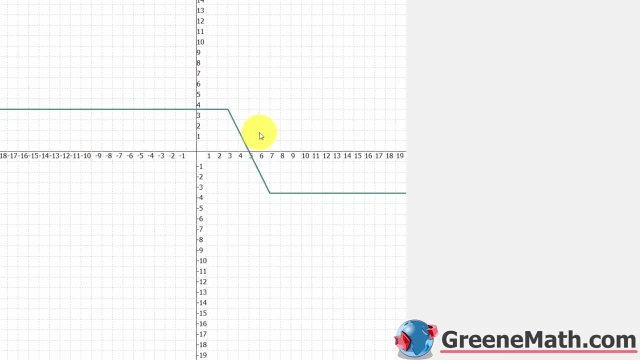 You're going to see where is the Y value equal to seven. pulling this up on math GV Again, you're going to see that it's never going to be equal to seven. Okay, That's why there's no solution. If I had said something like: 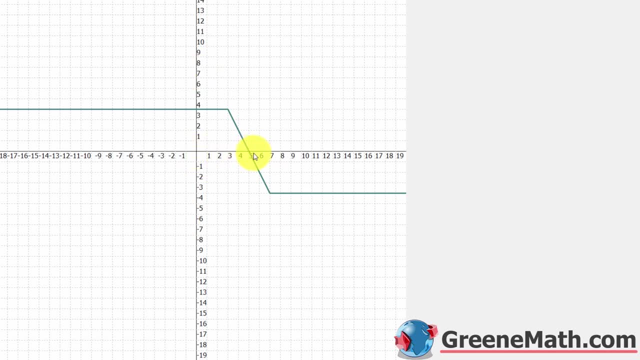 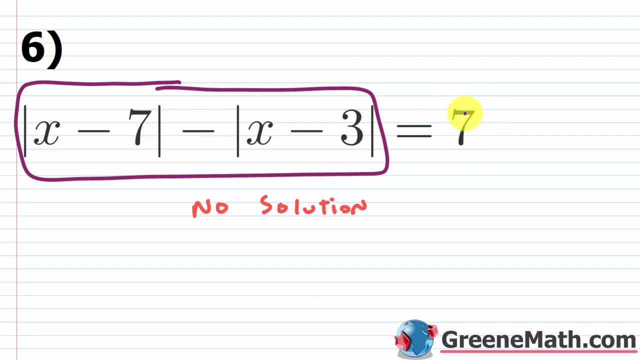 where is it zero? Well, this is a Y value of zero. Just look for the corresponding X value. That's going to be five, right? So if this had been this guy's equal to zero, here we would have found a solution of X equals five. 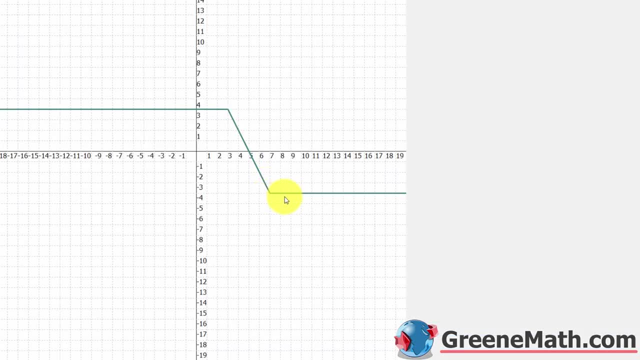 right. So this is one way you can clear up your doubts about things. You can just graph it and see what's going on. In this case, you see that that function that you create is never going to have a value of seven. 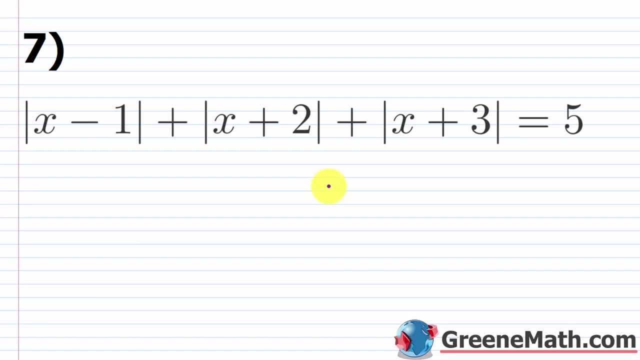 no matter what X value you plug in. All right, let's take a look at problem number seven now. So we have the absolute value of X minus one, then plus the absolute value of X plus two, then plus the absolute value of X plus three. 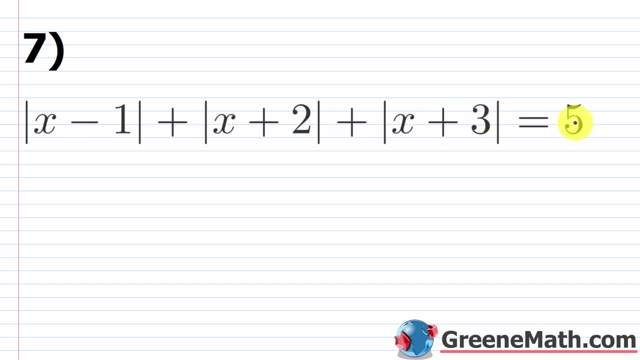 and this equals five. So this one is a bit more tedious, but you use the same strategy, Okay. So it doesn't matter how many of these you have, You can just set up cases. Okay, I'm going to go through this a little bit more quickly. 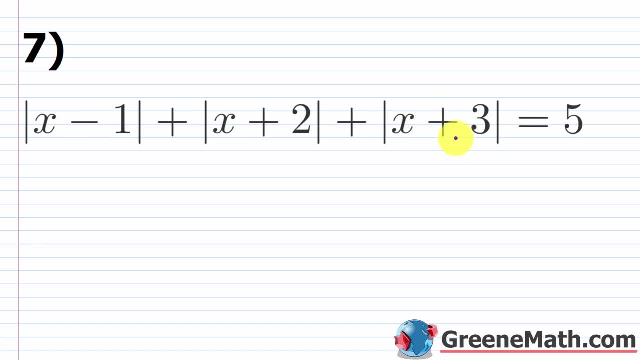 Now I'm going to tell you that one of these end points, specifically negative three, is going to work. So that's another chance for us to look at what to do when that occurs. So for this one, you would basically say X minus one. 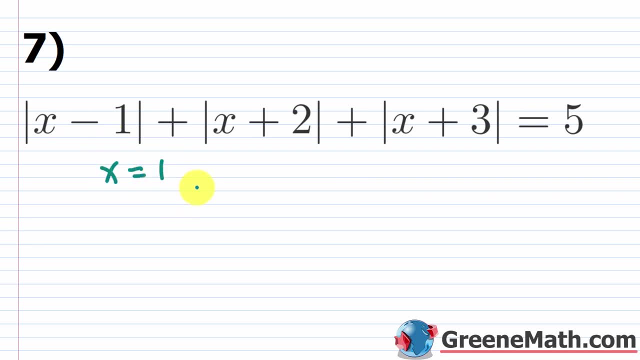 you set that equal to zero and you solve, So you get X is equal to one For this one, X plus two. if you set that equal to zero and you solve, you get X is equal to negative two For this one. 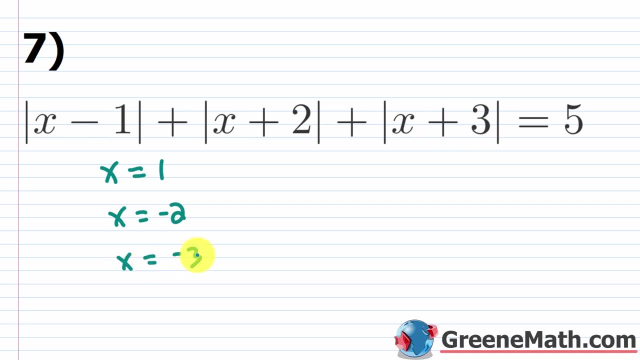 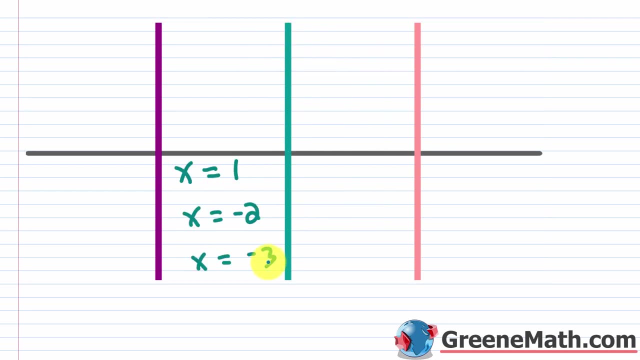 if you set X plus three equal to zero and you solve, you get X is equal to negative three. So let's grab these real quick And I'm just going to paste this in And let's just go ahead and say: the furthest to the left is: 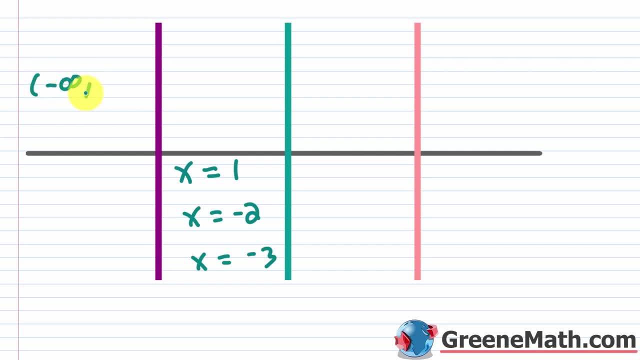 negative three. So I want from negative infinity up to an excluding negative three. Now for this one. if you want to include a negative three, you can. it's gonna make the problem a little bit easier And this would be up to. 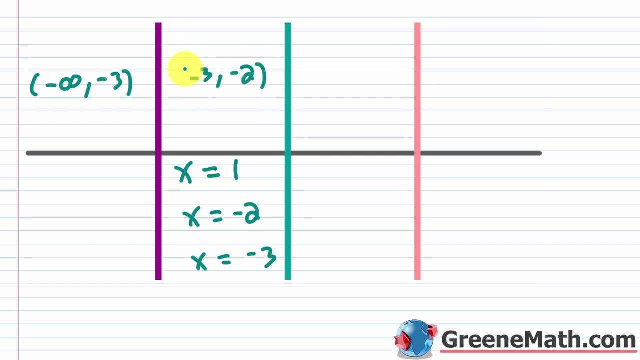 but excluding negative two. Okay, But I'm just going to exclude it for right now And I'm going to show you how you could solve it this way And again. maybe I'll put it down here just for reference, Okay, In case you want to do it that way. 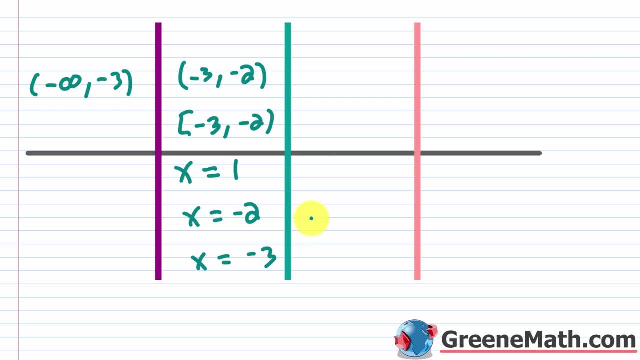 a lot of people like this method better. Okay, So then the other one would be we would have between negative two and positive one, And again you can include negative two there and exclude one there. You're always including on the left and excluding on the. 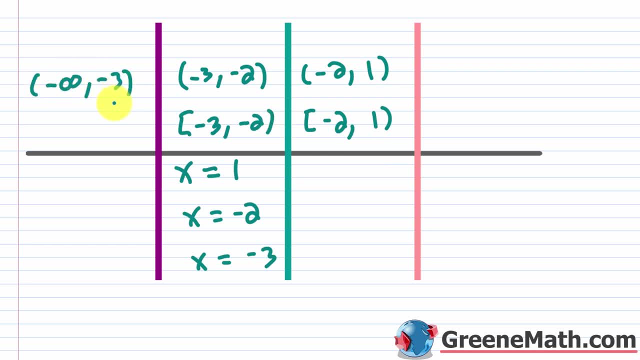 right, but this one furthest to the left: everything has to be excluded. Okay, I specifically want strictly less than negative three. Okay, Then this one right here would be anything that's greater than one, And again you could write this with one being included and out to. 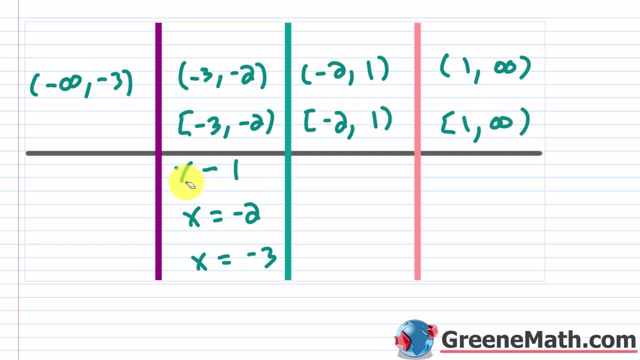 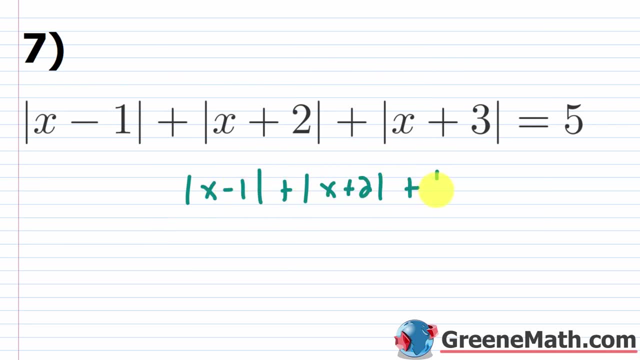 positive infinity. Okay. So let's get rid of this. Let's come up here and say: this is the absolute value of X minus one, and then plus the absolute value of X plus two, and then plus the absolute value of X plus three. 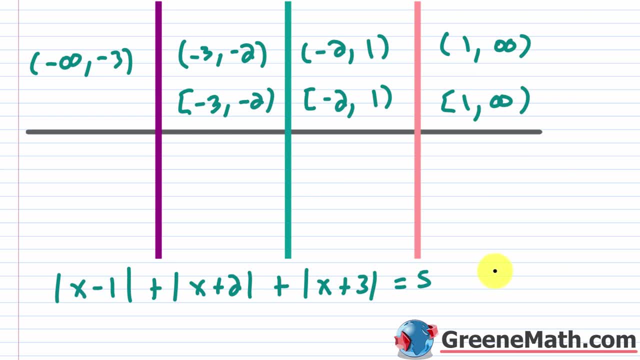 and this equals five. Let's do this one at a time. So first off, let's consider the absolute value of X minus one. So basically this is going to be zero where X is one. So I'm thinking about this column here. 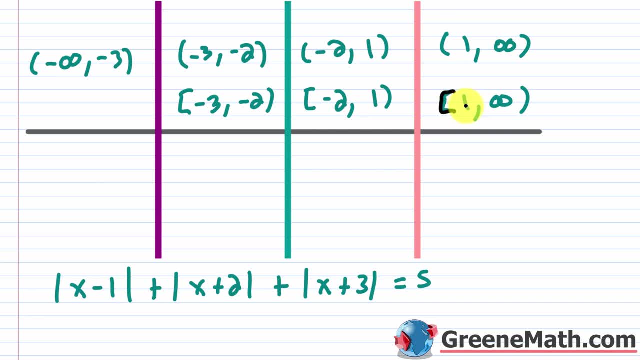 right. So if I include it, then at one it's zero, right, And anything larger is positive. So whether you're doing it this way or this way, you would just drop the absolute value bar in that case, right. so this is just x minus 1. now going to the left here of 1, well, it's always going. 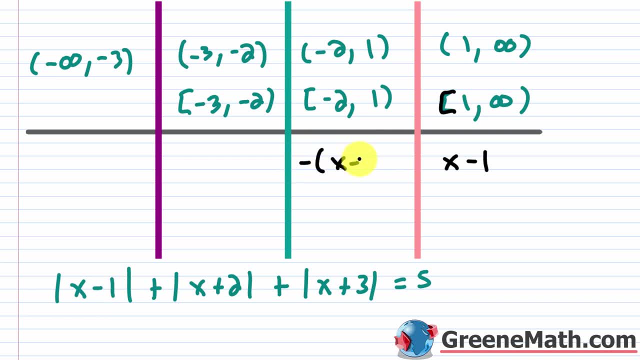 to be negative, right? so i want the negative of the quantity x minus 1, and let's just do that now. that's negative x plus 1. so this is negative x plus 1. this is negative x plus 1. this is negative x plus 1. the other guy is the absolute value of x plus 2. so when x is negative 2, it's going to be. 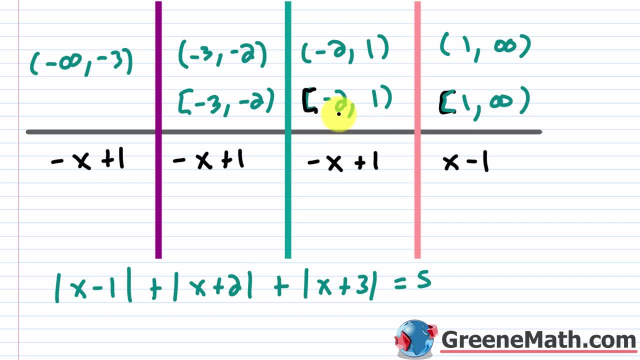 zero. so again, if you had included it right there, that's where it would be zero, and then anything larger. it's going to be positive. so here it's going to be x plus 2. i could just drop the absolute value bars, either for this one or this one, and here it's going to be x plus 2. okay, and then going. 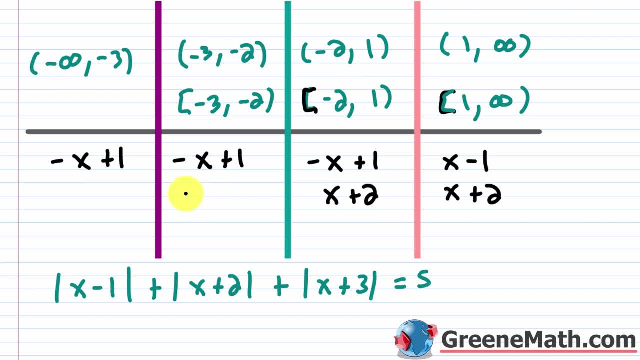 to the left, it's going to be the negative of this quantity: x plus 2. so negative x minus 2, and then negative x minus 2. okay, lastly, we have this x plus 3, so that's going to be zero where x is negative. 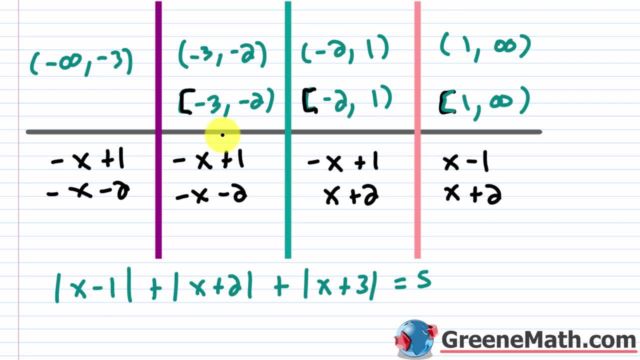 3. so again, if you include it, that's where it's going to be, or it's going to be positive, positive if you're greater than negative three. So again, either way, whether you include it or not, you can just drop the absolute value bars. you get x plus three here. you get x plus three here. 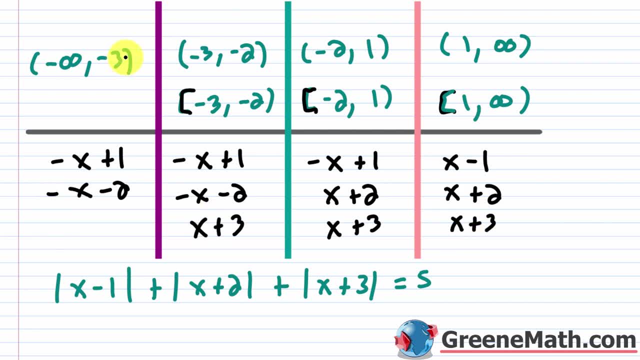 and you get x plus three here And then to the left of negative three, which is where we are here. you would want the negative of this. So this is negative x and then minus three. So let's go through and consider what's going to happen. we're going to see something interesting because 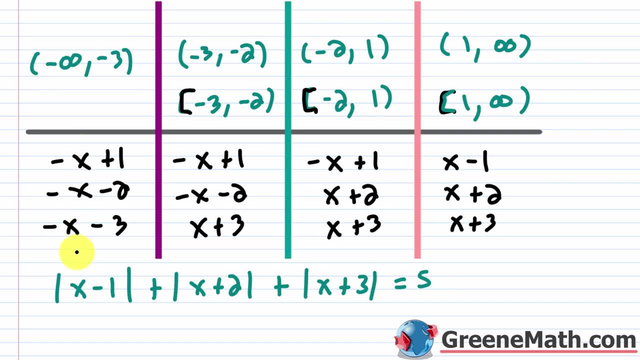 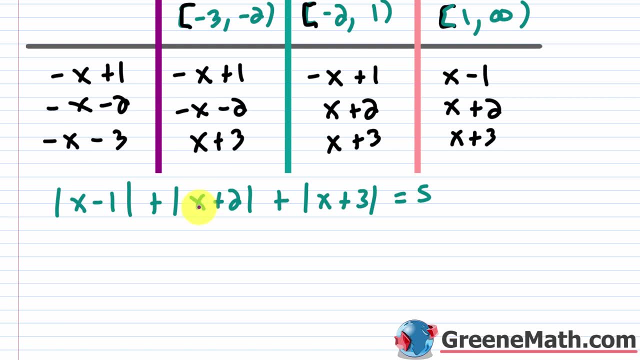 negative. three is going to be a solution when we get in here, And then also it's going to be a solution when we get in here. Okay, so let's come down here And let's think about the first scenario. So we're going to have: all of these guys are negative, So negative x plus one. these are 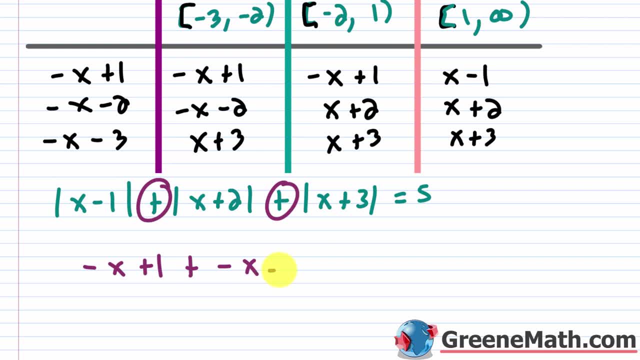 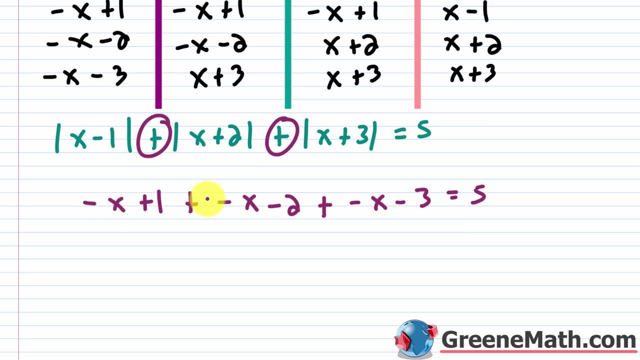 all plus signs. So just go through. we'll say: plus negative x minus two, and then plus negative x minus three, and this equals five. let's just collect terms really quickly: negative x minus x. minus x is negative three, x, and then one minus two is negative one and then minus three is negative. 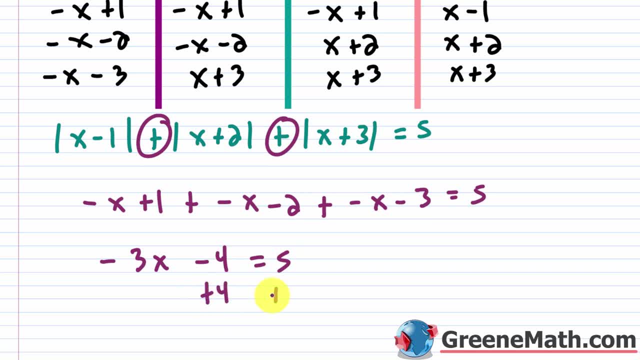 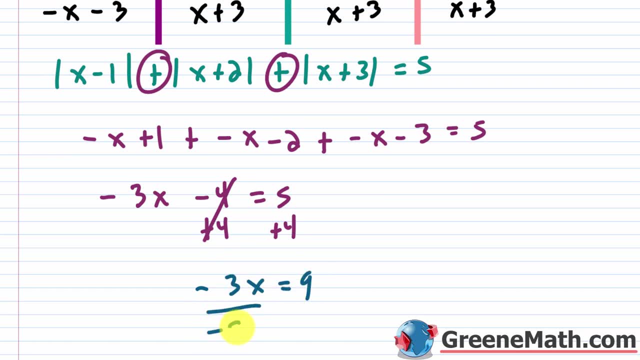 four And this equals four. Let's add four to both sides. we'll cancel this And we'll say that negative three x is equal to nine. divide both sides by negative three And this is going to give me that x is equal to negative. 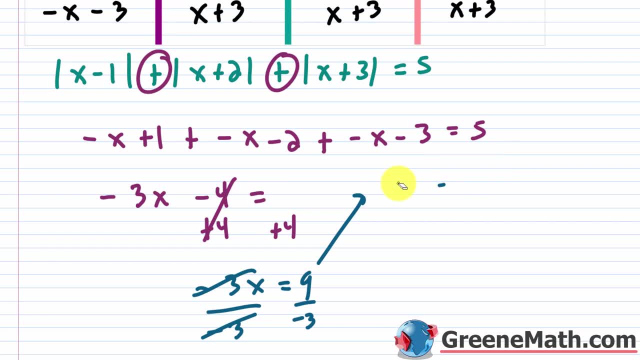 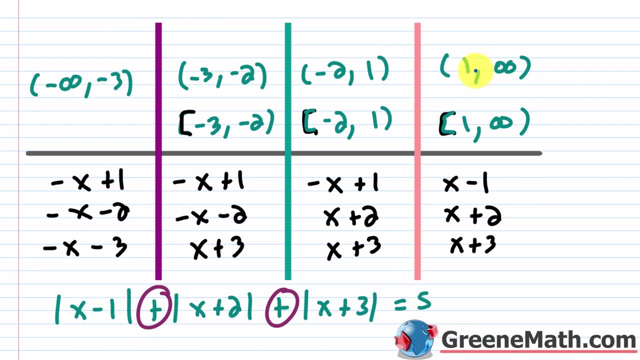 three: Okay, this is canceled. Now, whenever you get something and it's on one of those break points, well, you want to consider it And at this point, because I use this method, I would make myself a little note to check negative three. I would plug it in and see that it works And I 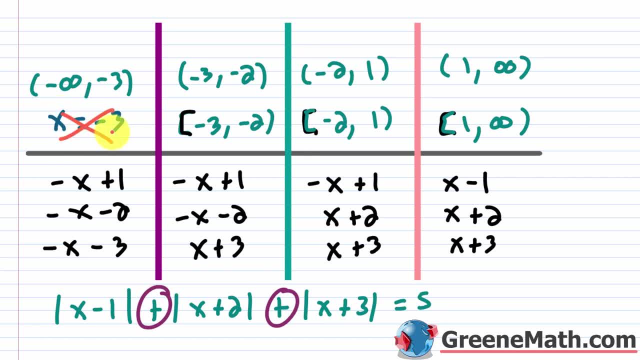 would try to get through this rule for a little more easier. So I'm gonna let you know how to get through this rule and then I'll get through the rest of the problem. but that's gonna be a matter of coming back to this little playbook. Your teacher is generally not going to see this. this is where 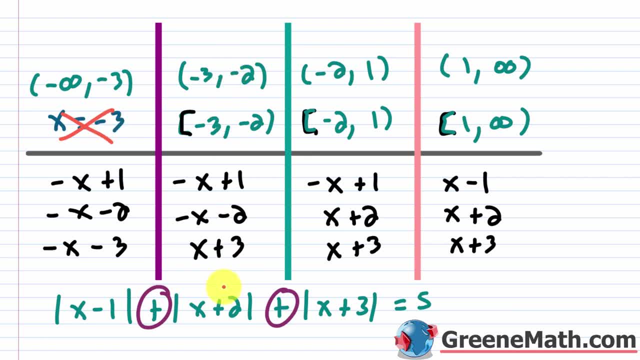 I'm going to reject because negative three is not in this interval, right? This is less than negative three, So negative three is not specifically included. Now, when I solve this one, negative three is going to be the solution again, And here's where you have to make a decision, right? 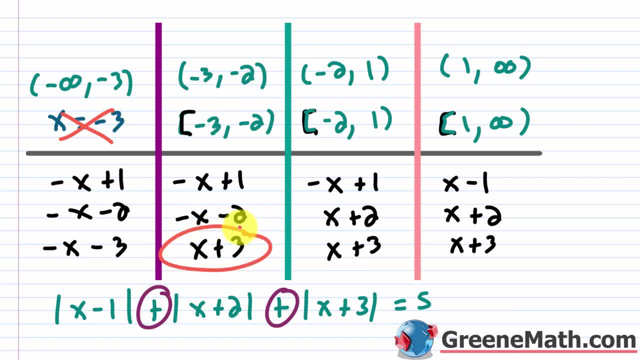 You can include negative three here legally, because it does not change this guy right here. whether it's negative three or something larger than negative three, it's still going to be me just dropping the absolute value bars, Okay. So in this case, if you want to use this method, it's going to be a little bit quicker. 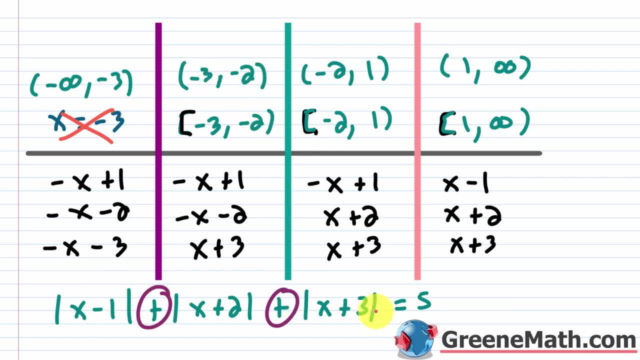 But again for myself, I would use this and I would just test negative three and see does it work. The answer is yes, So then I would include that in my solution set. So for this one let's just go through it. 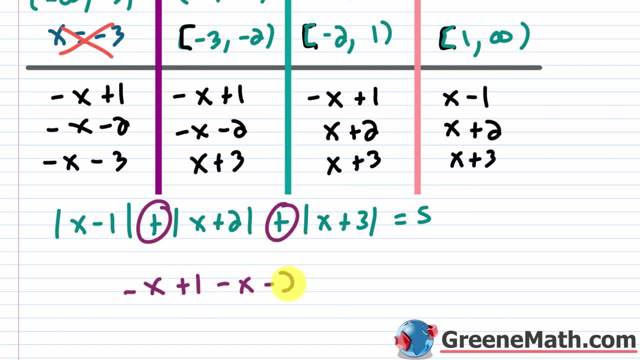 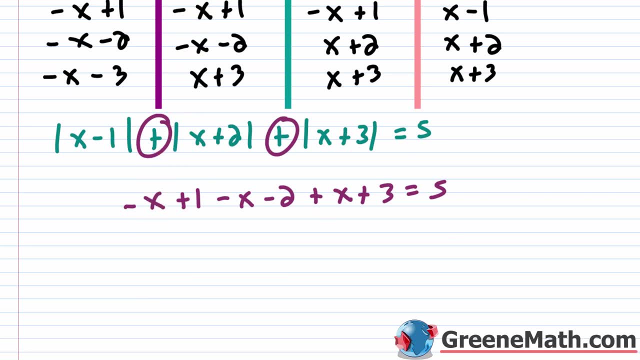 So you have negative X plus one, and then I'll just go minus X minus two and then plus X plus three. This should be equal to five. So negative X plus X. that's gonna cancel. Let me just show that This would cancel. 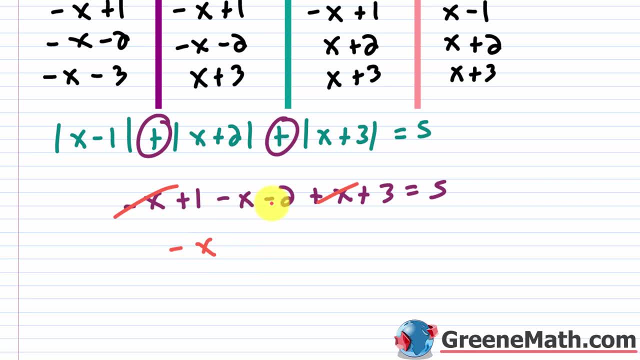 And you have negative X. So one minus two is negative one, And then negative one plus three is gonna be plus two, And this equals five. Let's subtract two away from each side. We'll cancel this. We'll say that negative X is equal to five minus two. 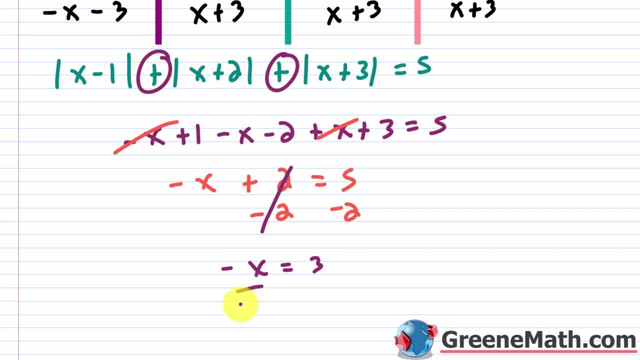 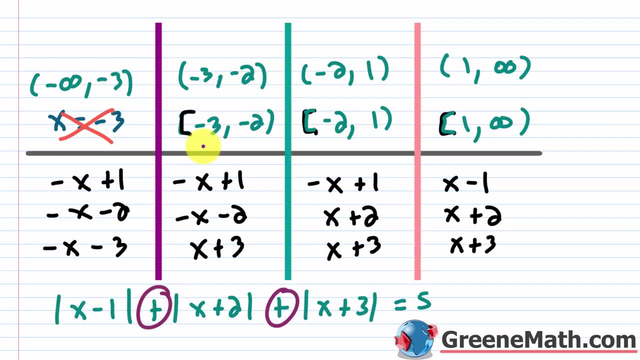 is going to be three. Multiply or divide both sides by negative one, Doesn't matter, Let's just divide both sides by negative one. This will cancel And you're gonna say that X is equal to negative three. So if you're using this one right here, 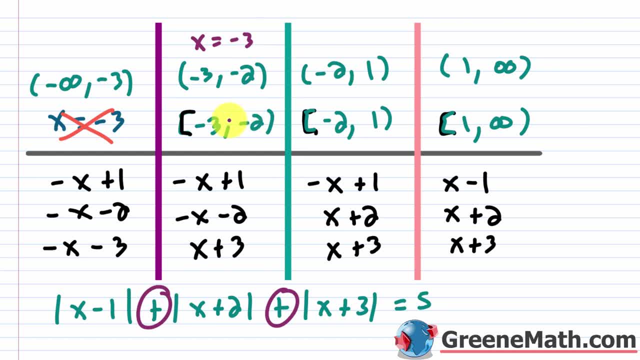 let me write this up here, maybe. So X equals negative three. If you're using this right here, well, negative three is included, So you can accept this solution Now if you're using my method here that I like to use. 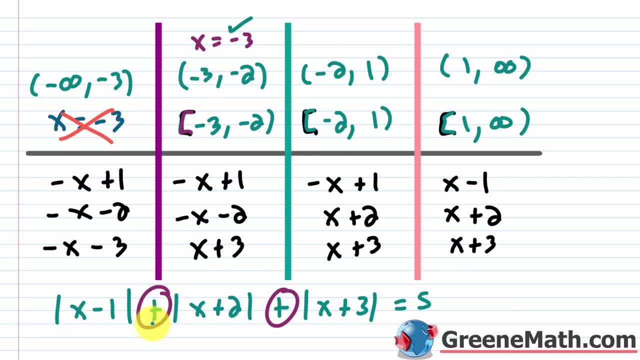 when I get something that's a solution, that's a break point, why just plug it in again and see does it work? And I know negative three works. So when I write my final solution, I'm just gonna include: X equals negative three. 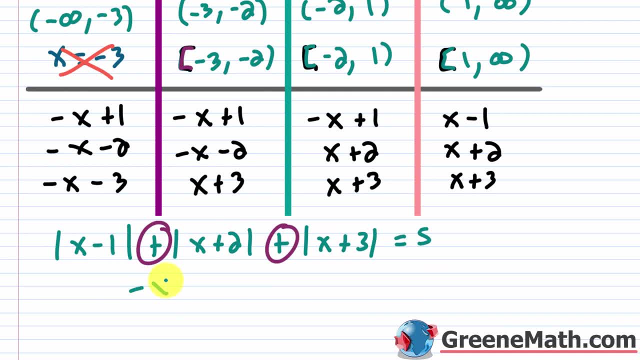 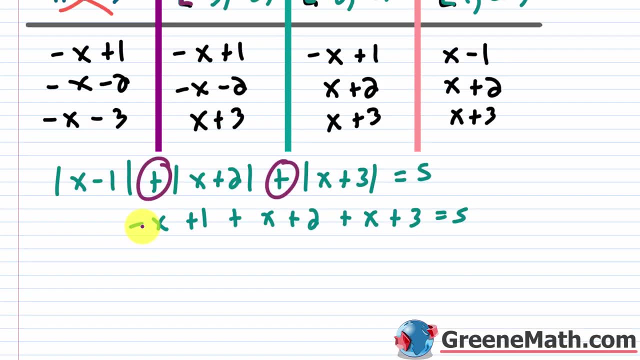 Okay, so that's how we do it. So for this one let's go through and we'll say negative X plus one, and then plus X plus two, and then plus X plus three is equal to five. So negative X plus X. that's gonna cancel. 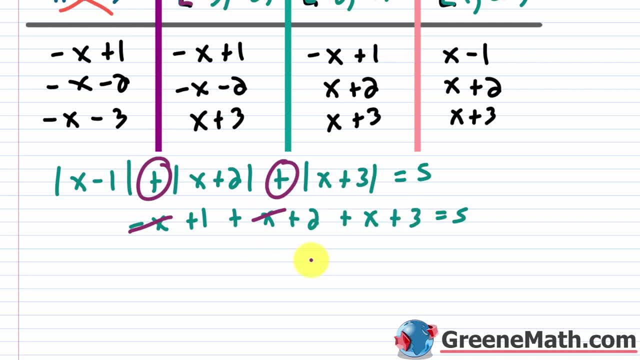 So you have one plus two, which is three, plus three, which is six. So you have X plus three. X plus six is equal to five. If you subtract six away from each side, you get X is equal to negative one. 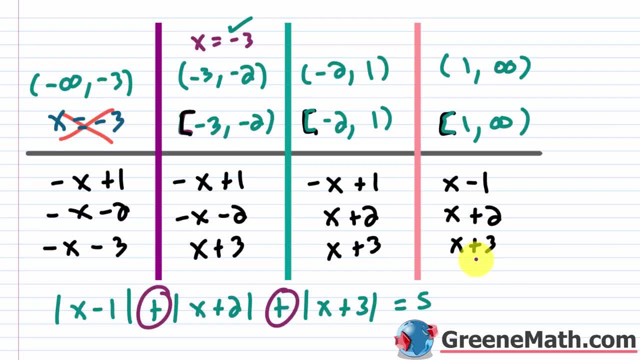 So X is equal to negative one. Would I accept that? Let me write that up here. So X equals negative one. Well, yeah, that's in this interval and this interval, no matter which one you used in this case. So I would accept that. 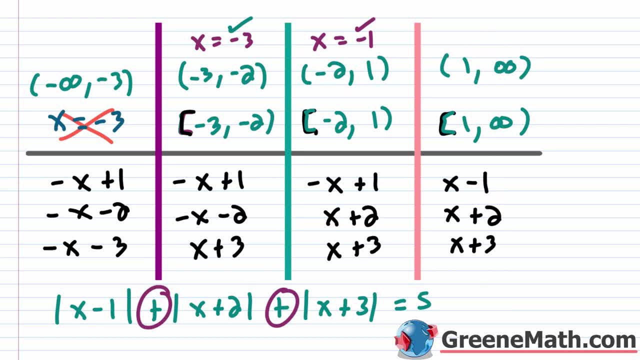 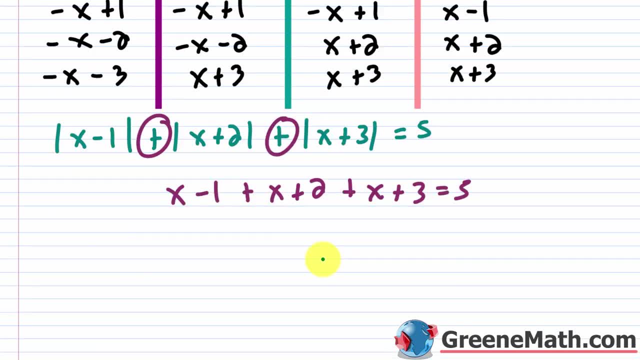 So X equals negative one. All right, let's take this one, We're gonna end up rejecting. So you have X minus one plus X plus two plus X plus three is equal to five. So X plus X plus X is three. 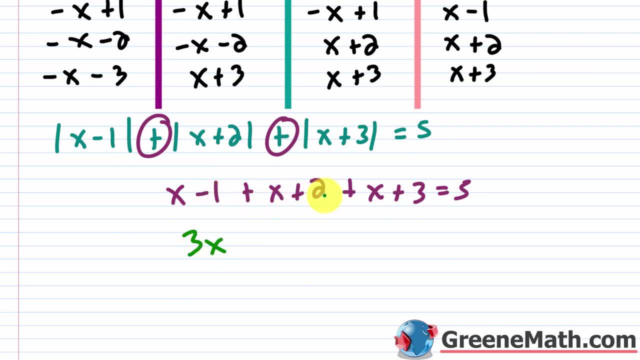 So if I subtract three X, negative one plus two is one, then plus three is four, So plus four is equal to five. Let me make that better. If I subtract four away from each side, let's just say three X is equal to one. 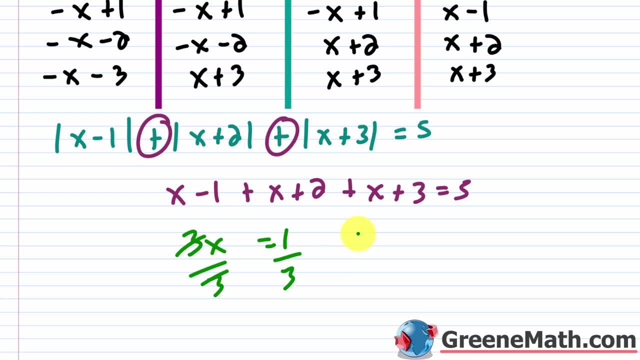 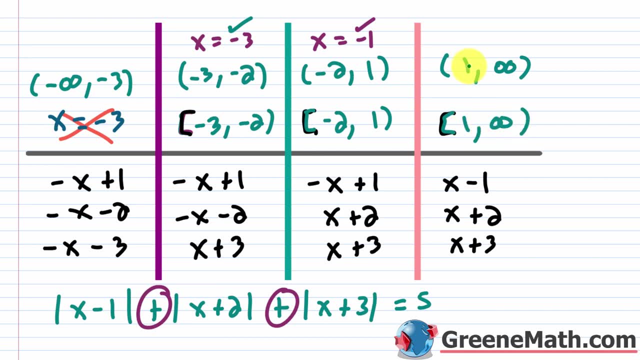 Divide both sides by three. This cancels. you get. X is equal to a third. Now, that is not gonna be in that interval. Remember: this is anything that's one or greater. if you're using this one or this, one is just anything greater than one. 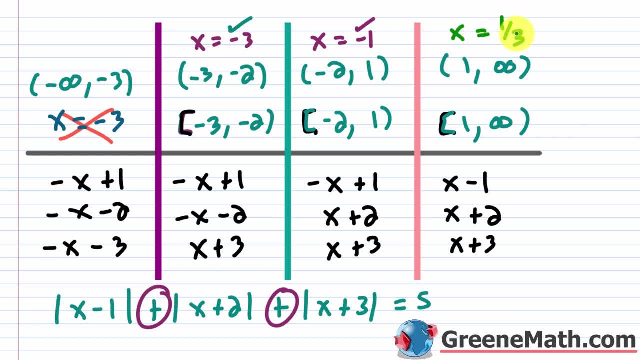 Again, it doesn't matter, because here X is one third right And we have to reject that, So this would be rejected. So, looking at everything again, whether you use this method or this method, you're gonna find that X is negative three. 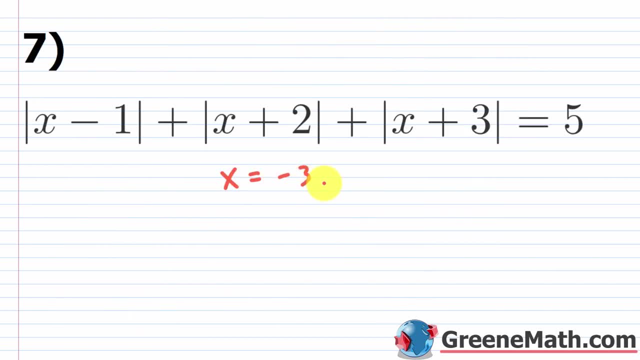 or X is negative one. So, coming back, I'll say X is equal to negative. three then, or negative one, And then again, if you wanna do this graphically, you could take this left side here and punch it into Desmos or MathGV. 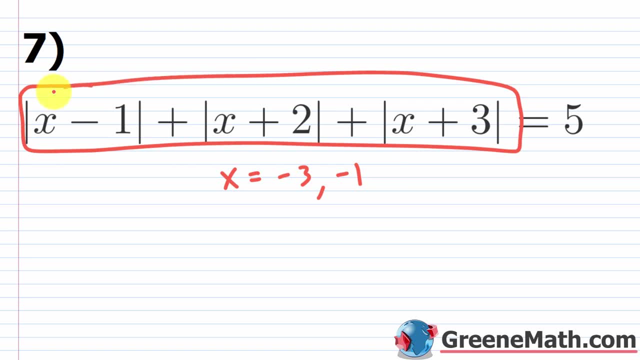 or whatever free calculator you wanna use. Basically, the absolute value of X minus one plus the absolute value of X plus two plus the absolute value of X plus three. Just see where the function's value is five. I see that it would be five. 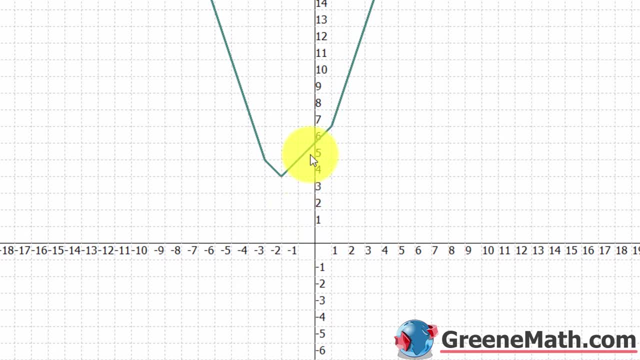 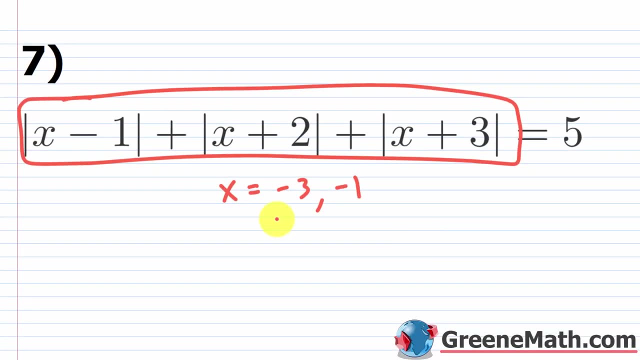 Just going across here: this is where it's negative one. And then going across here: this is where it's negative three. okay, So you can verify that graphically if you have your doubts. but either way, the solution is: X equals negative three. 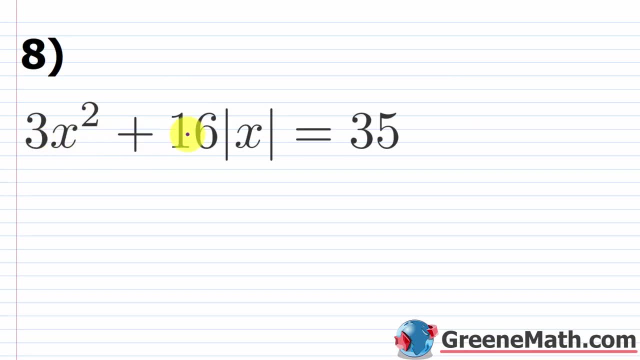 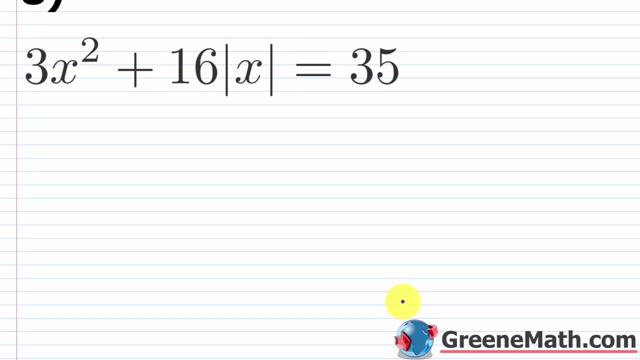 or X equals negative one. All right, let's take a look at problem number eight now. So here we have three X squared plus 16 times the absolute value of X is equal to 35.. So I talked about in the lesson two different ways you could solve this type of problem. 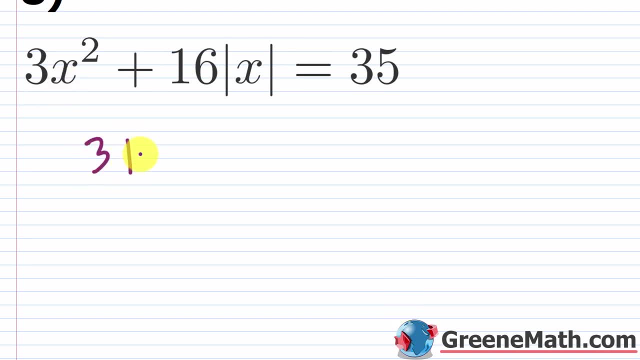 I'm just gonna use a substitution. So first I'm gonna write this as three times the absolute value of X being squared, Because, remember, if I have X squared, that's gonna be equal to the absolute value of X being squared. Those two would be equal. 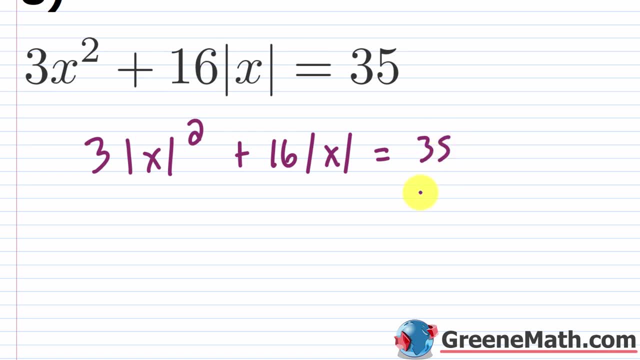 Then plus, we have 16 times the absolute value of X, and this equals 35. So now I'm going to let something like U or Z or whatever you wanna use, be equal to this absolute value of X. So I'm just gonna plug that in here. 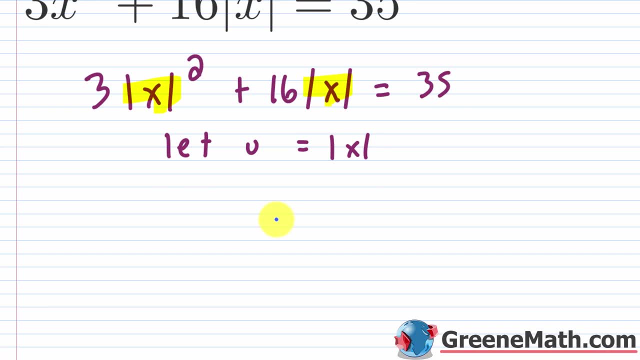 and here and make a simple quadratic to solve. So this would be three U squared plus 16 U, and let's subtract 35 away from each other, So minus 35 is equal to zero. This is something we can solve using factoring. 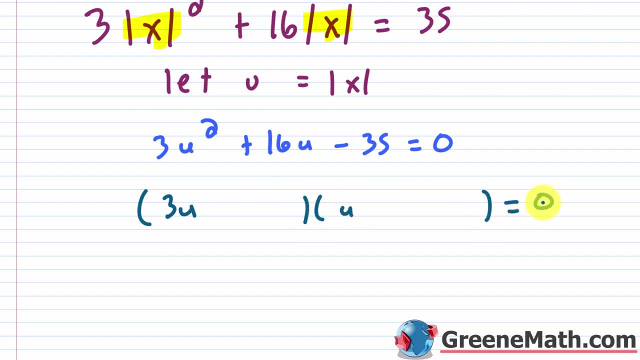 So I'm just gonna put a three U here and then put a U here And let's set that equal to zero there. For this guy right here it's negative. So I know the signs are gonna be different And I'm going to subtract. 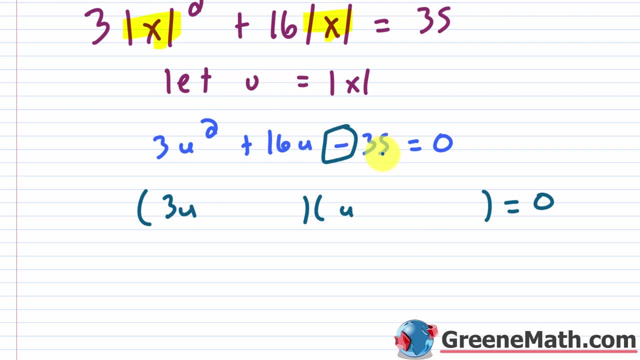 I'm gonna try to get the 16. in terms of absolute value, 35 is one times 35. And that's not gonna work. And then you have five and seven, So that's basically it. So if you put the seven here and the five here, 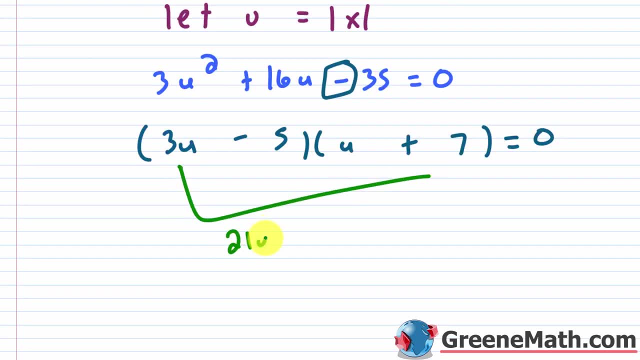 plus and this a minus. it would be good to go. This would give us 21 U and this would give us negative five U. And again, 21 U minus five U would be 16 U. So we would say that three U minus five is equal to zero. 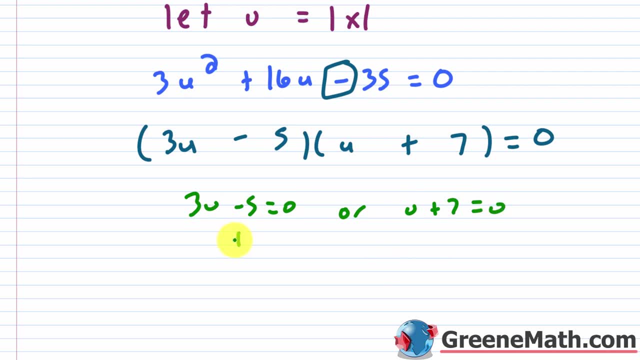 Or U plus seven is equal to zero. Let's add five to both sides. Cancel this. We get three. U is equal to five. Divide both sides by three And we'll say that U is equal to five thirds. So let me put that up here. 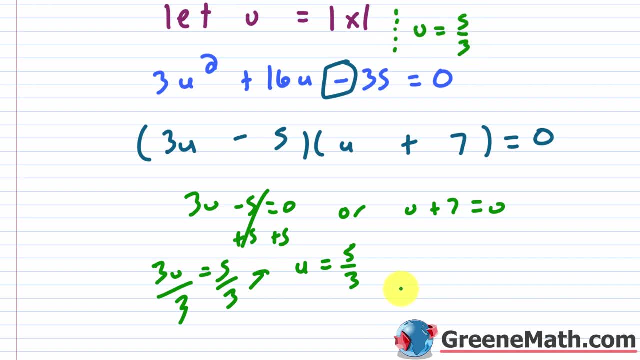 Put U is equal to five thirds, And then we'll say that, and then over here I'm just going to subtract seven away from each side of the equation. Let's cancel that, so it can also be negative seven. Let's put negative seven there. 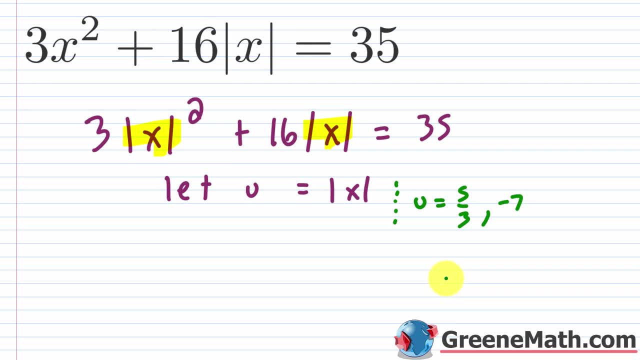 When you solve these, you often get ones that you have to reject, So we let U be equal to the absolute value of X. So I'm just gonna say that the absolute value of X is equal to five thirds, Or the absolute value of X. 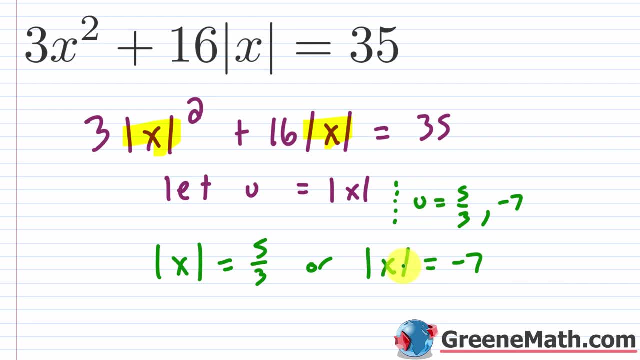 is equal to negative seven, And I'm just getting that by replacing this U with the absolute value of X. Okay, You can actually get rid of this. We don't need it, And you can even get rid of this if you want. You don't need it. 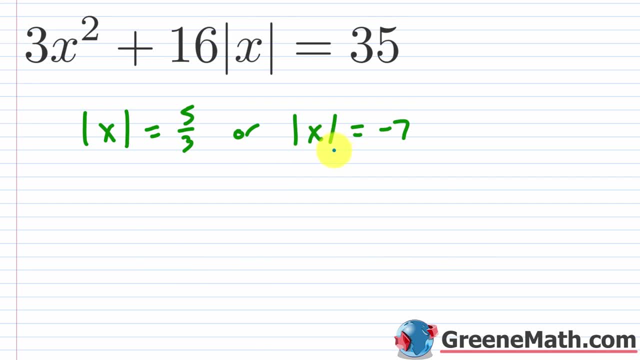 So let's bring this up here Now. this guy on the right has no solution. Right, The absolute value of X can never be negative seven, So we'll just put no solution for this part And then over here. this is really simple. 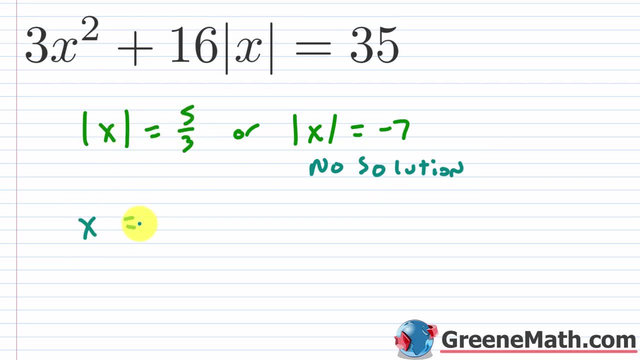 If the absolute value of X is set equal to five thirds, well then, X is five thirds or X is negative. five thirds, Right. And you can write this in a more condensed form by just saying that X is equal to plus or minus five thirds. 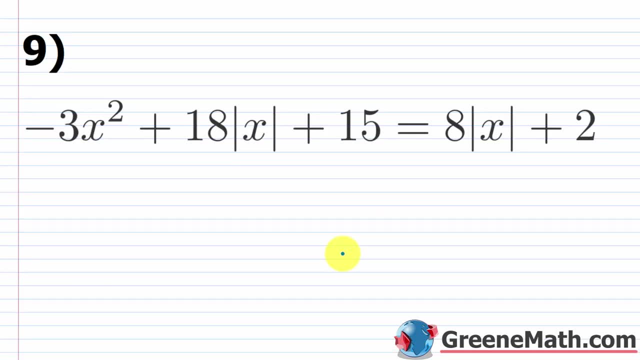 So that would be your solution. You can pause the video and check each one and verify that they work. Okay, Let's look at problem number nine. So again, we're going to use the same strategy here. Now you can clean this up first, or you can substitute first. 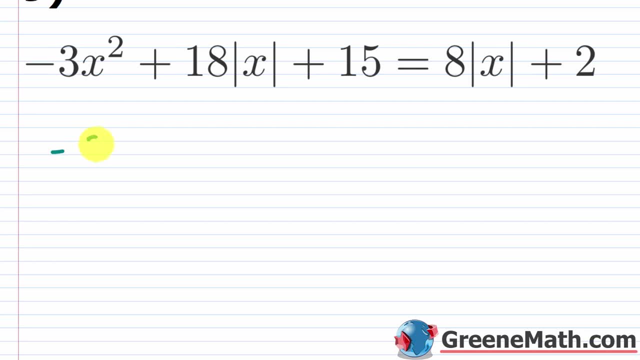 It really doesn't matter. I think maybe we can clean up first. Let's just say negative three X squared, I'm going to subtract eight times the absolute value of X away from each side. So if I have eighteen times the absolute value of X, 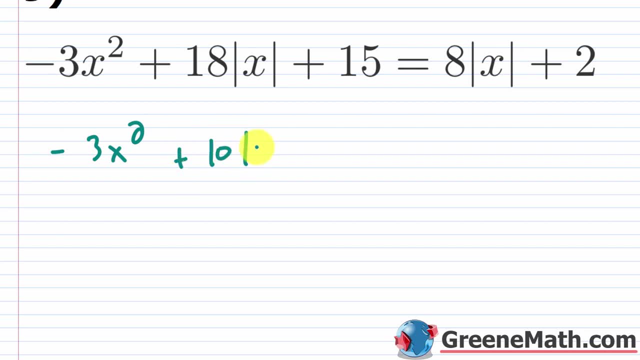 minus eight times the absolute value of X, that's going to be ten times the absolute value of X. Then basically subtract two away from each side. This is going to be fifteen minus two, which is thirteen. so plus thirteen, and this equals zero. Okay, So that's a simpler form. 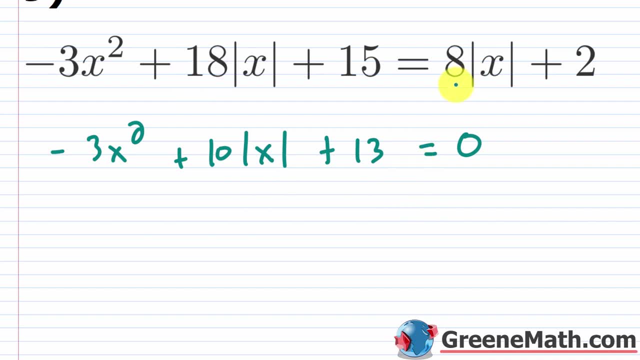 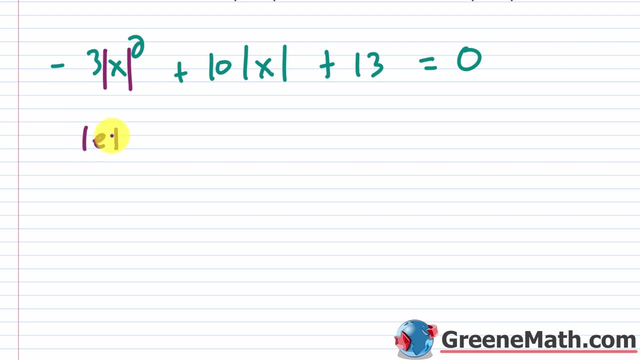 If you want to do the substitution first, you can do that and then simplify Again. it doesn't matter. So what I'm going to do is actually just replace this like this: Again, that's perfectly legal- And then I'm going to let U. 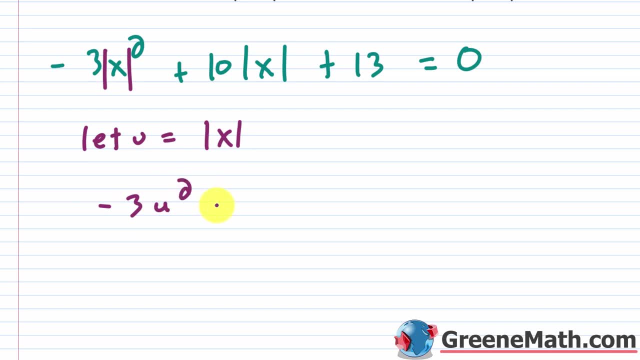 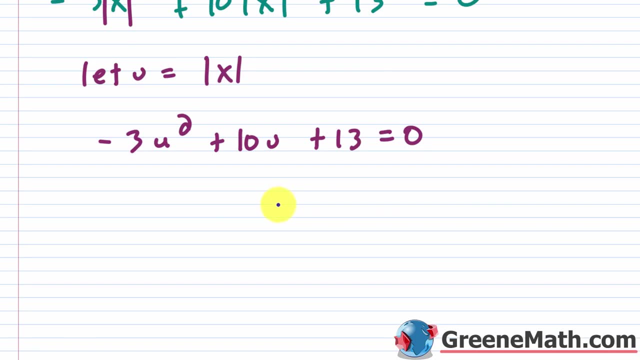 be equal to the absolute value of X. So this is negative. three U squared, then plus ten U, then plus thirteen is equal to zero. And so with this one I'm going to multiply everything by negative one, So I don't have to deal with that negative out in front. 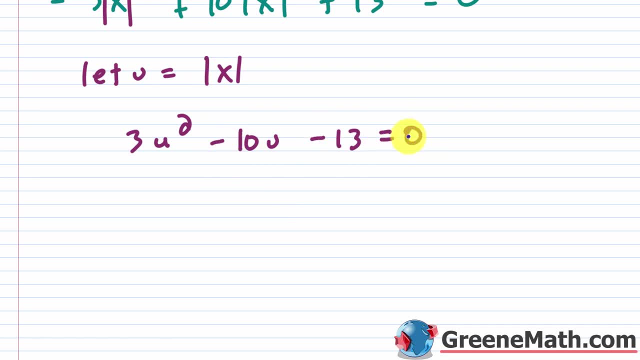 Let's change the sign of all those and then zero times negative. one is still zero. So I'm going to factor this and put this as three U and then put this as U put a zero out here, and so again, this is a negative here. so I know I have mixed signs. 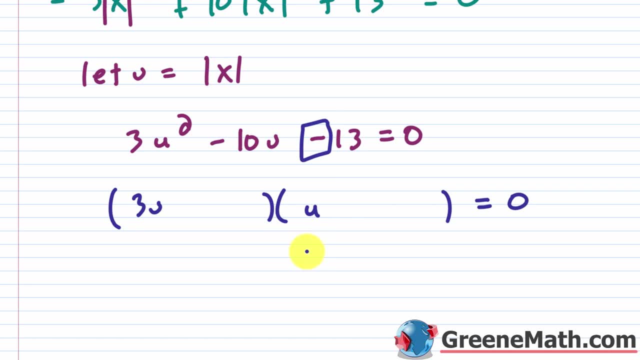 and thirteen is actually a prime number, So it can only be one times thirteen. So it can't be here, because three times thirteen is thirty-nine and it's just going to be too big. So it has to be a thirteen here and then a one here. 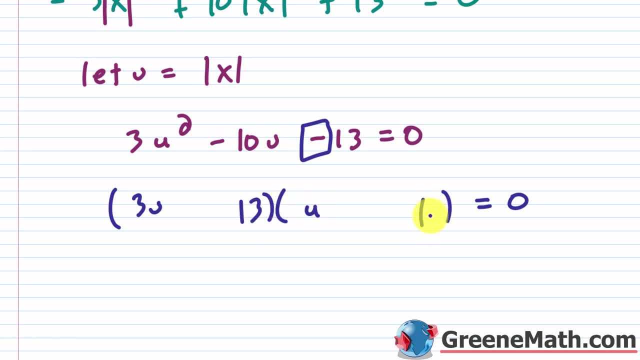 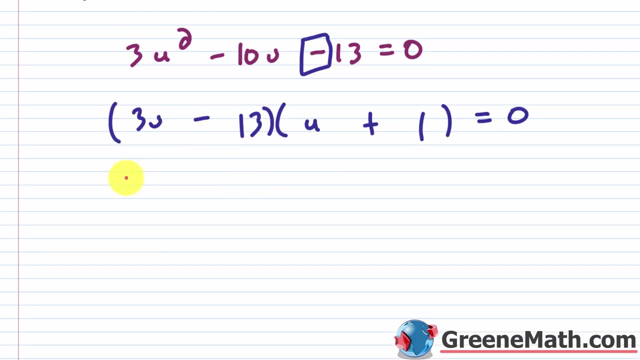 So it has to be thirteen minus three, which is ten. So I need to make this negative and this positive, so that I end up with three U and then negative thirteen U. so positive three U minus thirteen U would be negative ten U. so this is what I'm looking for. 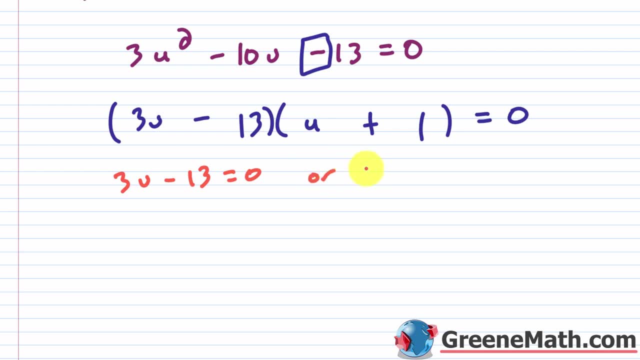 So what I'll do here is say three: U minus thirteen is equal to zero. or U plus one is equal to zero. So this one, we know that basically U is equal to negative one. Right, That one's easy. For this one we would add thirteen. 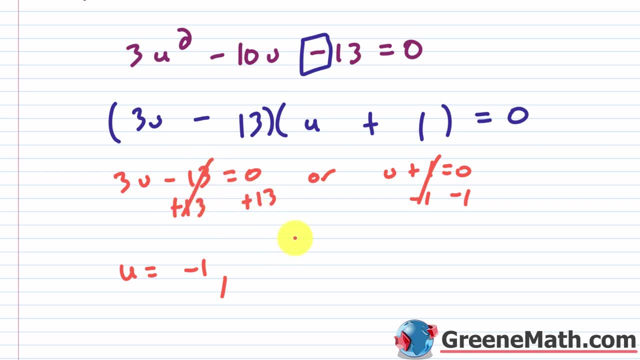 to both sides of the equation. this would cancel and you get three. U is equal to thirteen. divide both sides by three, this cancels, so U could also be thirteen over three. So, coming back up here, I'm actually just going to get rid of this. we don't really need it. 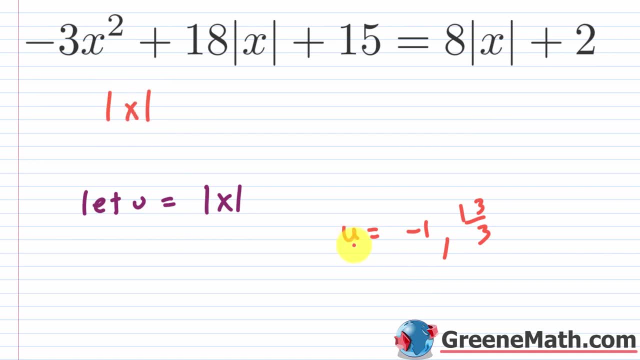 so I'm going to say that we have the absolute value of X, because that's what U is. this is equal to negative one. or the absolute value of X is equal to this: thirteen over three. Okay, So once again we know that the absolute value of X 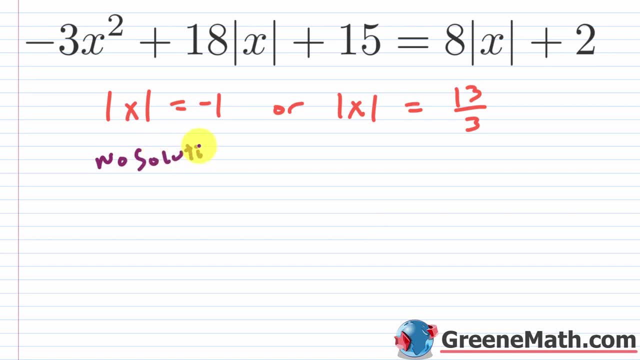 cannot be negative one. This would be no solution. Okay, so no solution there. For this one, it's just that X is equal to thirteen over three or negative thirteen over three. so we'll just say plus or minus thirteen over three and you can get rid of all of this. 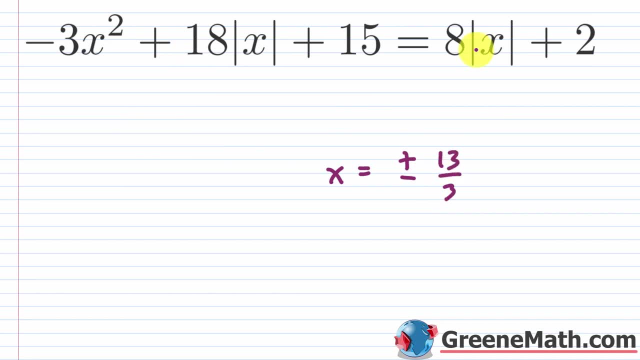 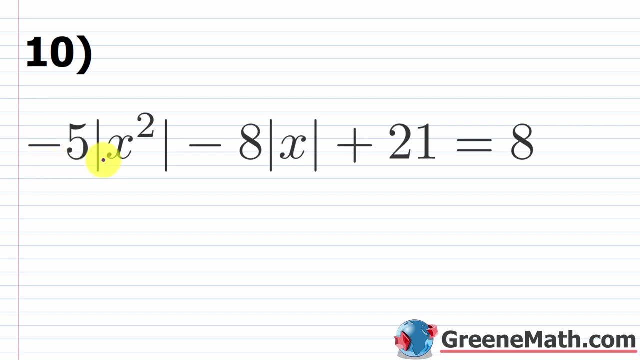 at this point and just report this as your answer. again, you can check each one in the original equation and verify that they work. Okay, let's look at problem ten. so here we have negative five times the absolute value of X squared then minus eight times the absolute value of X. 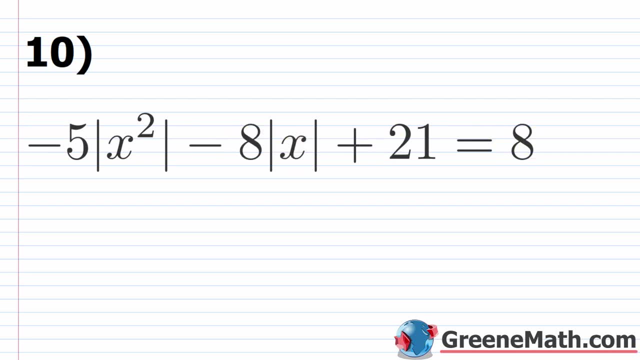 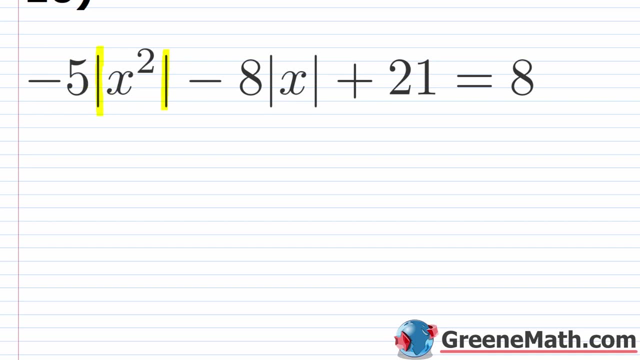 then plus twenty one is equal to eight. okay, so this one is really the same as the other ones. this part right here is meant to trip you up. a lot of books will do this, but you have to realize that the absolute value of X squared is the same thing as if I had. 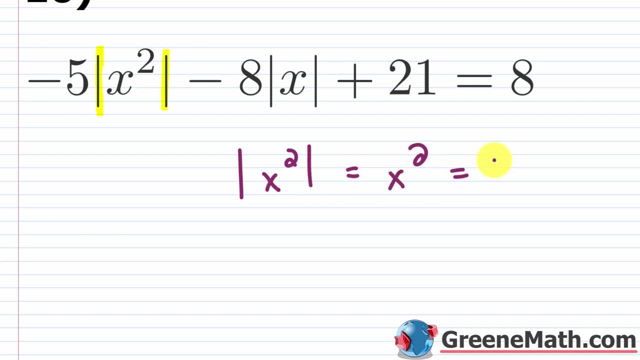 X squared right, these are both going to be non-negative, and it's also the same thing as if I had the absolute value of X being squared like this. in each case, you're going to get the same result, whether you have a negative, whether you have zero or you have a positive right, it doesn't matter. 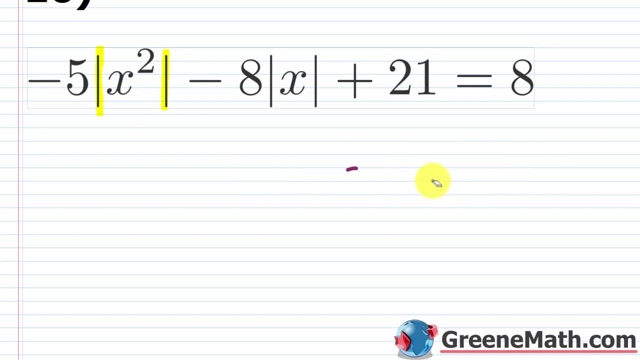 what you plug in, those will always be equal. so what I can do is rewrite this legally and say this is negative five times the absolute value of X being squared like this, then minus eight times the absolute value of X, then plus twenty one, and this equals eight. 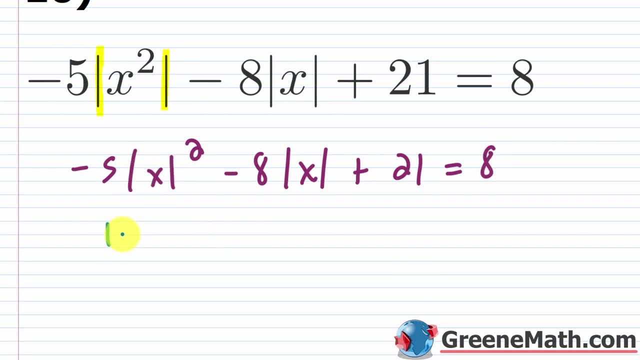 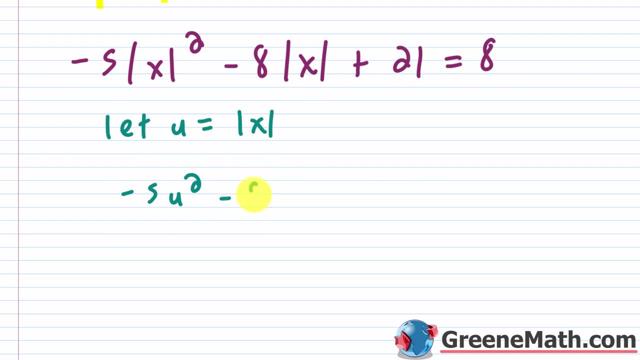 from here again, I can just replace the absolute value of X with U. so let's say that we're going to let U be equal to the absolute value of X and I'll say: negative: five times U squared minus eight times U plus twenty one is equal. 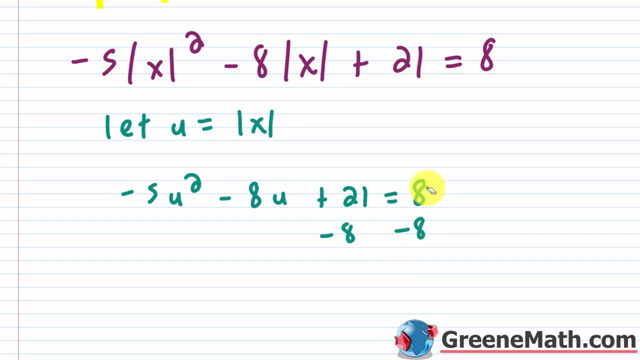 to eight. alright, for this one. let's subtract eight away from each side, so this would be zero, and then twenty one minus eight, that's going to be thirteen. and again, I don't want a negative leading coefficient if I'm trying to factor, so I'm going to multiply everything by negative. 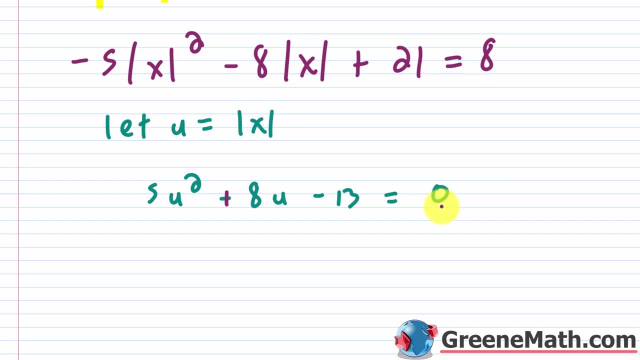 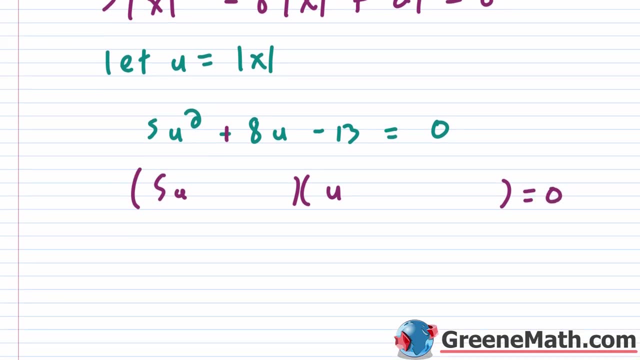 one. so that's positive, this is positive, that's negative and that's still zero. so let me try to factor this. I'm pretty sure that we can, otherwise we can just use the quadratic formula. so this guy, right here again with thirteen. it's one times thirteen only, okay. 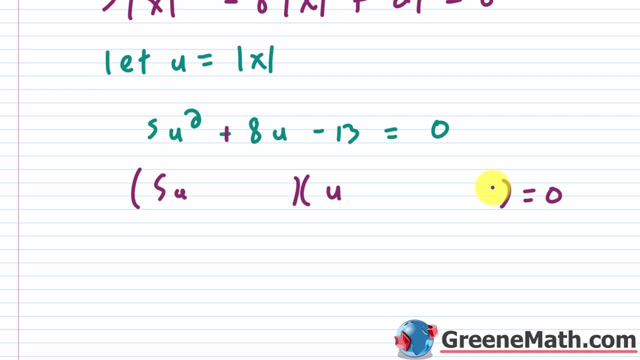 and this is minus. so I have mixed signs. putting a thirteen here is too big, so I have to put the thirteen here and the one here, and so this is five and this is thirteen. so thirteen minus five is eight. so I want to make sure that this is positive and this is. 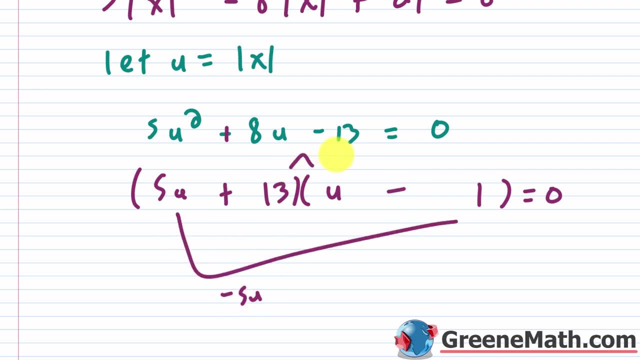 negative right. that way I get a negative five U and a plus thirteen U- let's make that three a little bit better- and so negative five U plus thirteen U, that would be the eight U that I'm looking for. so we would say: five U plus thirteen is equal. 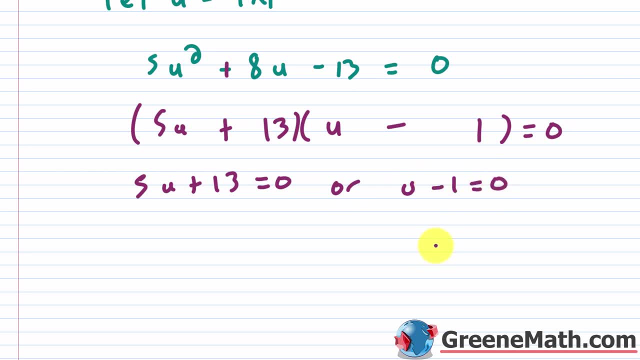 to zero, then, or U minus one is equal to zero. so here let's subtract thirteen away from each side. this cancels, you get five. U is equal to negative thirteen. divide both sides by five and you get U is equal to negative thirteen over five. now do you need? 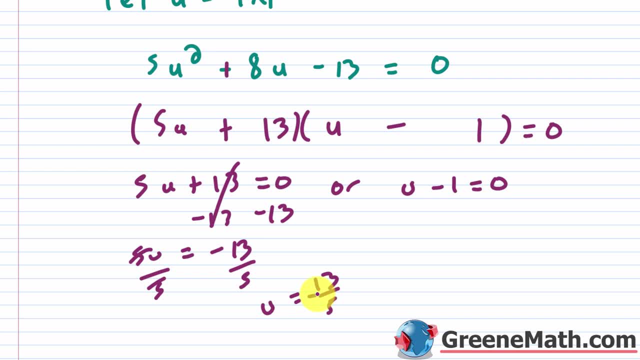 to include this? no, because U is the absolute value of X and the absolute value of X is not going to be negative thirteen over five. so just get rid of this branch, you don't need it anymore. we're just going to consider that U minus one equals zero. 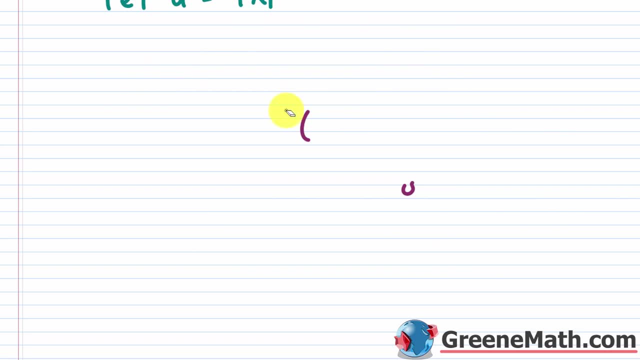 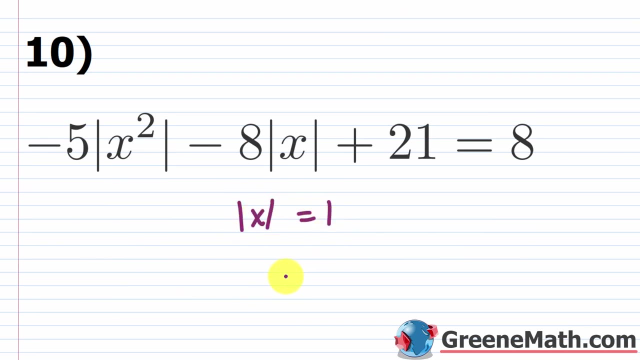 and that's the solution of U equals one. okay, so let's get rid of all this. we're just going to come back up here and say that the absolute value of X is, which was U is equal to one. so that means X is equal to one or negative one, so you could go.